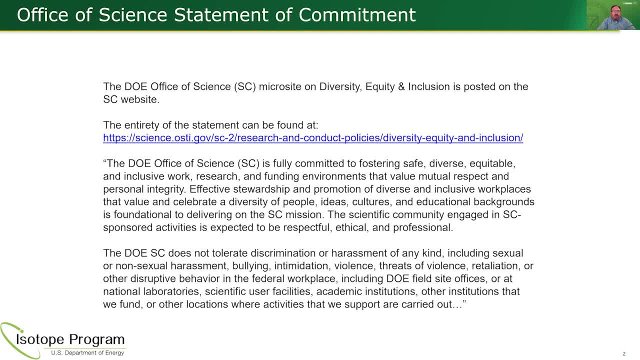 of Science microsite on diversity, equity and inclusion. There is a link that's posted in the slide deck. As Julie said, all the slides are already posted online. You can find the links there, and I believe Julie will be dropping some of these links into the chat window as well. 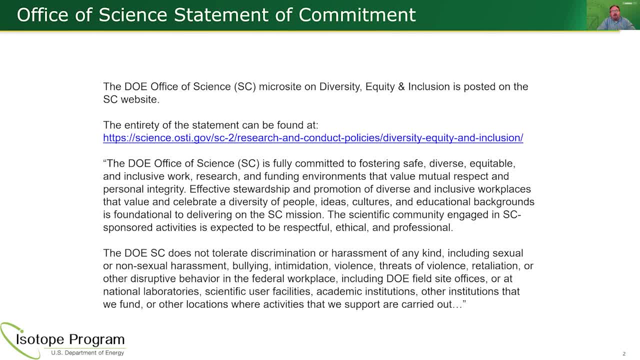 The chat is disabled, But you can use the Q&A function- You're encouraged to do so- to put any questions into us that way. Okay, So I'm just going to read you the bottom two paragraphs. The DOE, Office of Science, is fully. 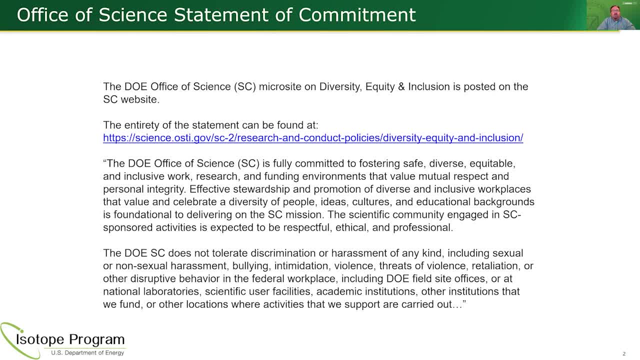 committed to fostering safe, diverse, equitable and inclusive work, research and funding environments that value mutual respect and personal integrity. effective stewardship and promotion of diverse and inclusive workplaces that value and celebrate a diversity of people, ideas, cultures and educational backgrounds is foundational to 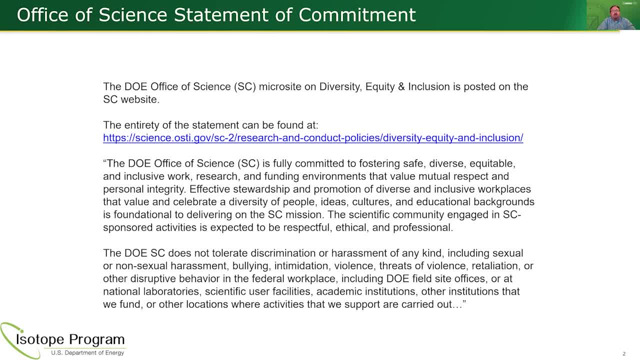 delivering on the SC mission. The scientific community engaged in SC-sponsored activities is expected to be respectful, ethical and professional. The DOE Office of Science does not tolerate discrimination or harassment of any kind, including sexual or non-sexual harassment, bullying, intimidation, violence, threats of violence, retaliation or other disruptive. 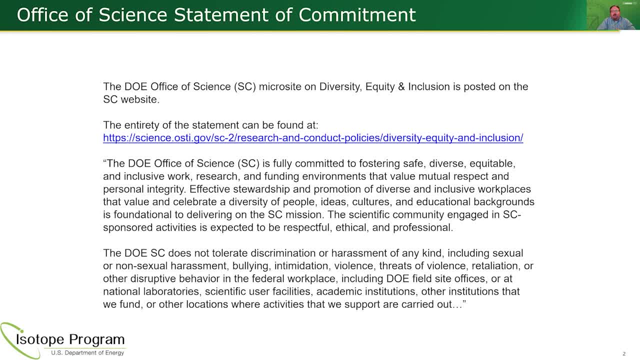 behavior in the federal workplace, including DOE field site offices or at national laboratories, scientific user facilities, academic institutions, other institutions that we fund or other locations where activities that we support are carried out. So I would ask that everyone please just act in accordance to the statement of commitment. 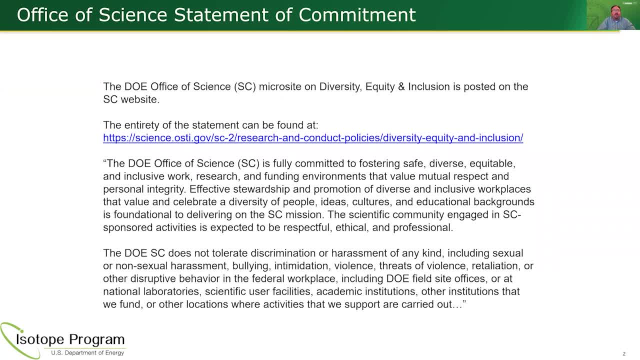 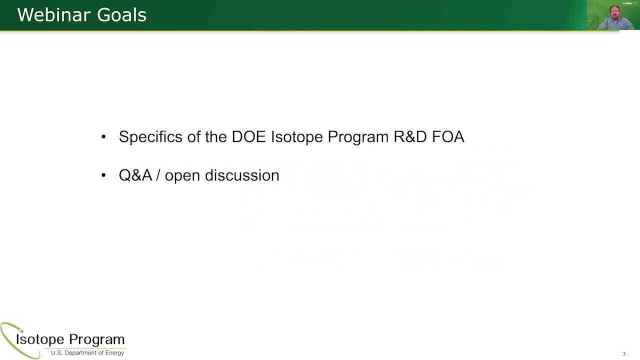 And with that we'll go right into the webinar for today. So there's a brief agenda. I'm going to walk you through the FOA itself. We'll talk a little bit about specifics. We'll talk about how to read it, how to interpret it, how not to interpret it. 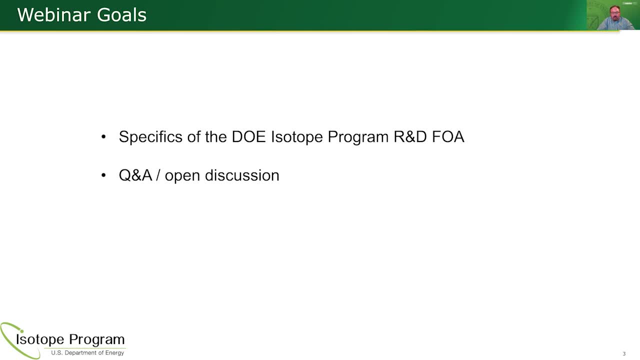 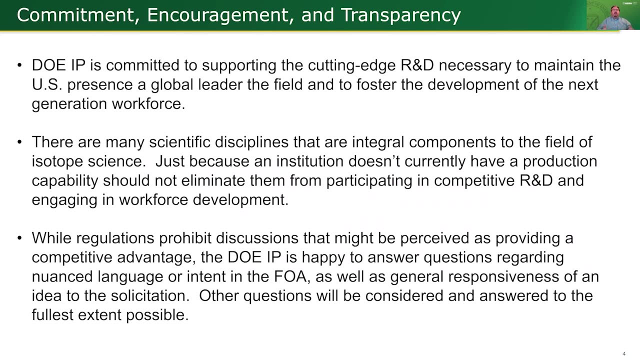 and then we'll open up for Q&A and anything that you would like to ask to the program directly. So, as far as being transparent about the goals of this particular FOA, it stems from three specific topics. So the first one is that, the iZotope. 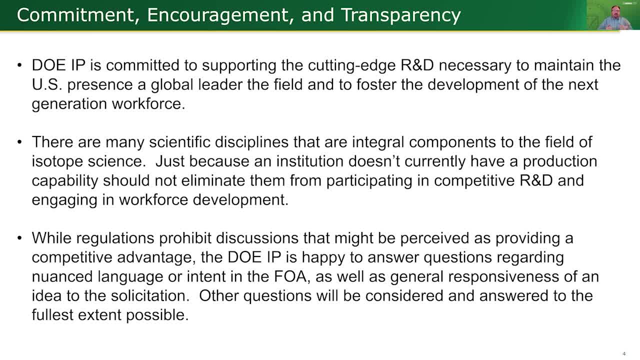 program is committed to supporting the cutting edge R&D that is necessary for the US to maintain its presence as a global leader in the field and to foster the development of next-gen workforce. Going along with that is the concept that isotope science itself can't be pigeonholed. 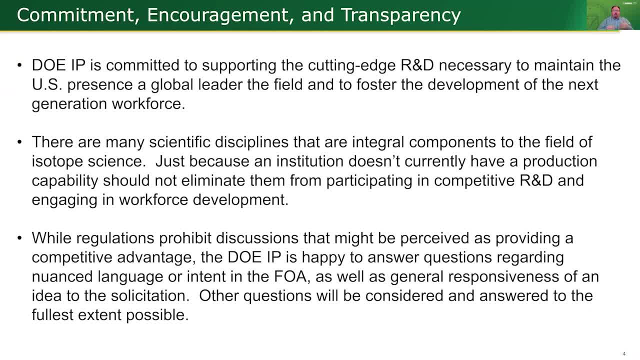 into one specific discipline. So when you're considering making application to this or any other FOA that the isotope program issues, one should always be conscious of the fact that just because you don't necessarily have a production capability at your institution, or should you not at that point, it might not necessarily eliminate you. 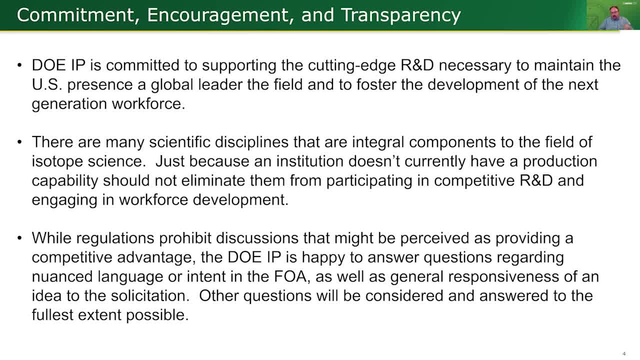 from participating in competitive R&D and engaging in workforce development. In fact, you may have capabilities in other areas that other institutions are lacking and that they might wish to really develop a strong collaboration with, and we encourage that. So, lastly, there are some regulations that prohibit discussions that might be perceived 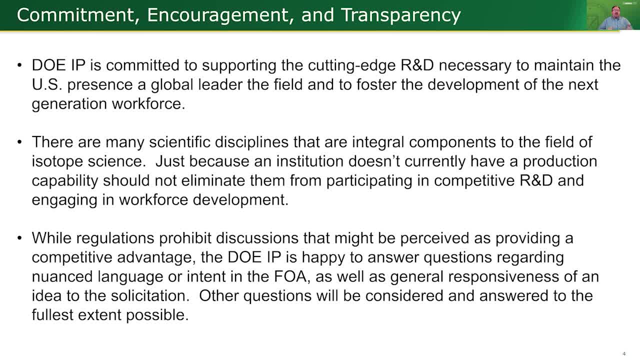 as providing competitive advantage. Obviously, I can't engage in providing those types of advantages, but we are happy to answer questions regarding any nuanced language that appears in the FOA, what the intent of the FOA is, as well as general responsiveness of an idea to the solicitation itself. Any other questions are: 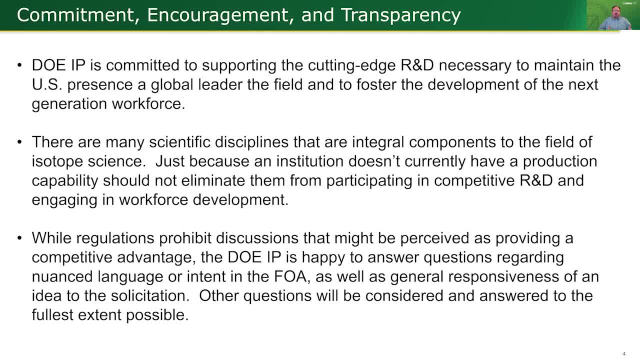 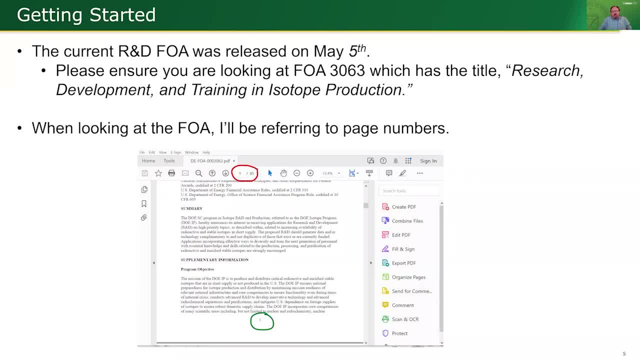 All right. So the current FOA is solicitation 3063 and has the title Research, Development and Training in Isotope Production. It was published on May 5th, So if you're following along, based on the PDF file that you can get from scienceenergygov, then you'll want to make sure. 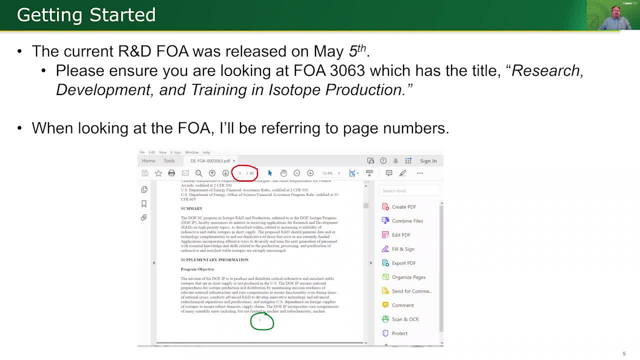 that you have the correct FOA open and it will open in Acrobat with uh window similar to what you see on the screen. I will point out that I'll be referring to page numbers and I will utilize the page number that is circled in green at the bottom of your screen. 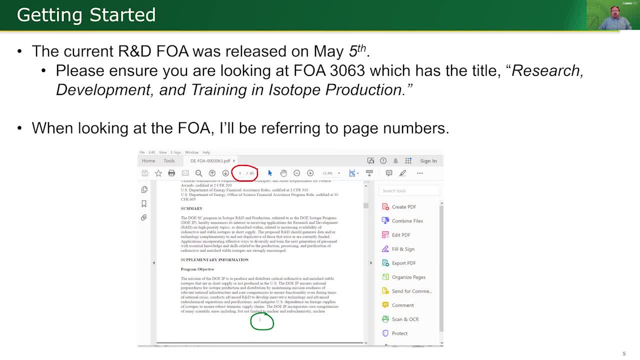 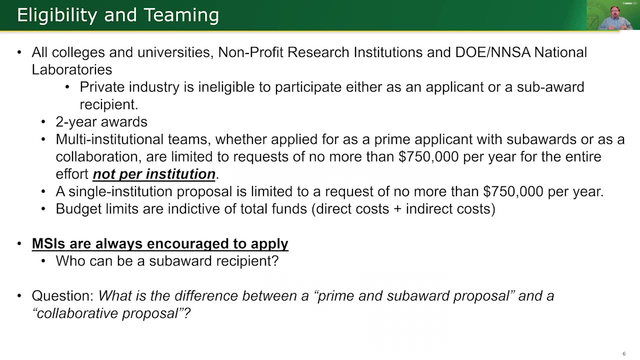 as opposed to those circled in red, because there's a disparity between the two. So I'll be referring to the PDF page numbers or the- I'm sorry, the document page numbers as opposed to the PDF page numbers. All right, Who's eligible? So all colleges and universities, non-profit. 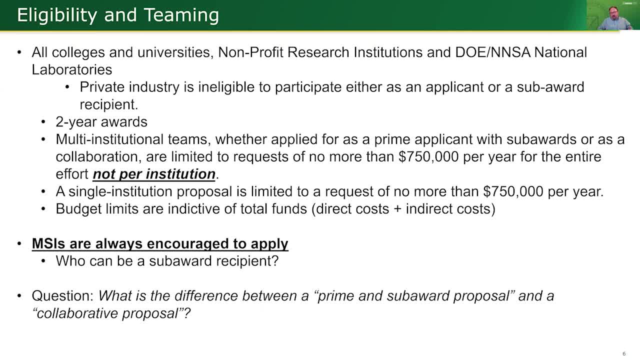 research institutions and DOE and NSA national laboratories are eligible to make application to this particular solicitation By special request. private industry is ineligible to participate either as an applicant or a sub-award recipient. These are in keeping with previous FOAs that issued by the program. These are two-year awards. 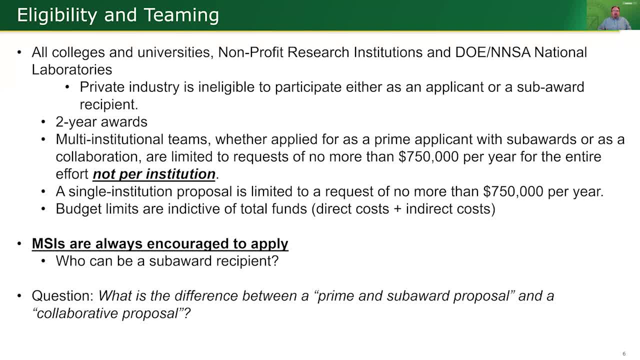 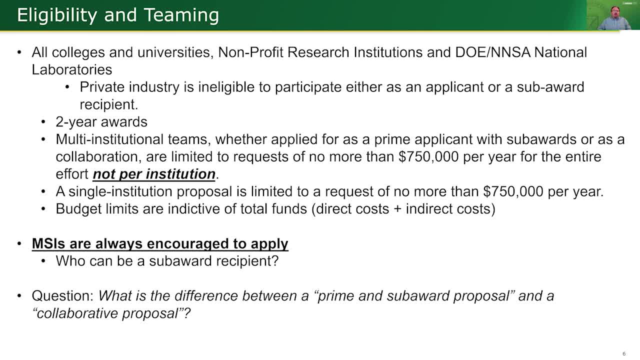 Does this include auditing or grant oppenn Forces? I do. I do obviously need to. may not need to call them. you know, go to, they may not be синced into, I might not be able to your sample here or, notwithstanding this discipline, whether on this. 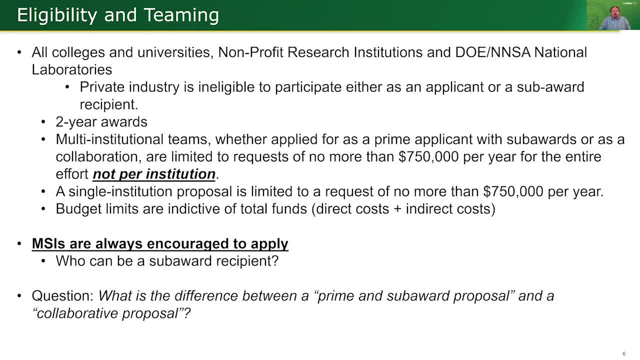 directs being separated out. So these are total fund budgets. Okay, MSIs are always encouraged to apply. And then that develops the question of who can a sub-award recipient be? Any of the eligible institutions? So that brings up the next question is: what's the difference between a prime? 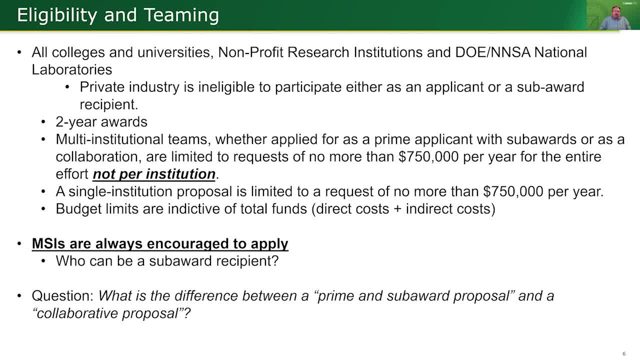 and sub-award proposal and a collaborative proposal. In a prime and sub-award proposal you've got a leading institution. For the sake of argument, we'll say that that lead institution happens to be a university. They might wish to have a certain PI from either another university. 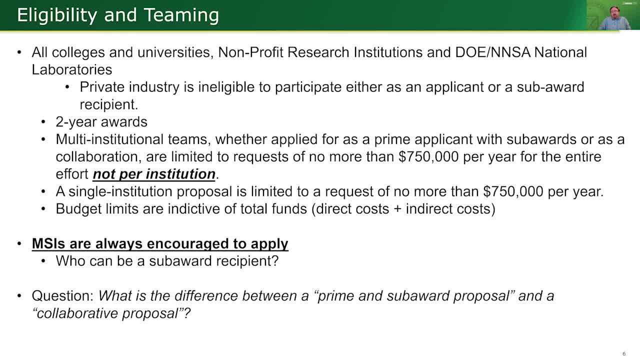 another nonprofit research institution or even a national laboratory conduct some of the funding And then they might wish to have a sub-award proposal, Some particular scope of work. but that scope of work is really just a service that's being procured in furtherance of the actual scope of work that's been proposed by the lead PI at the 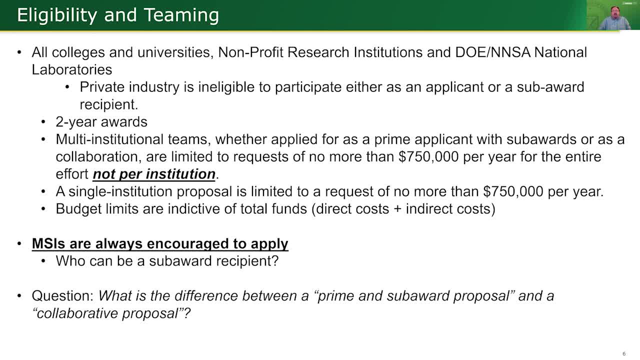 lead institution or the prime institution. In that case, the sub-award recipient is actually nothing more than a line item in the lead principal investigator's budget. You're procuring a service from that institution, And then you have a sub-award recipient, And then you have a sub-award. 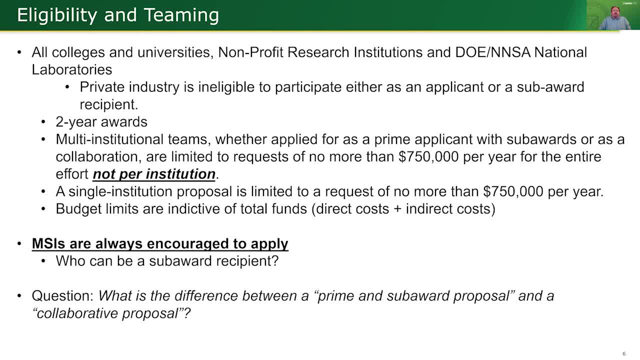 recipient from that researcher. In a true collaboration, you would have two proposals submitted with the same title and the same narrative. What differs is the scopes of work that are proposed at each institution and the budget and justification. obviously So in that case you have multiple PIs. You have the PI at the lead institution and then you have the PI. 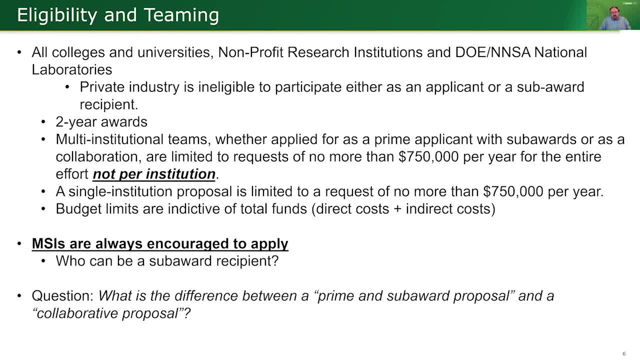 at the collaboration institution, And then you have the PI at the lead institution, and then you have the PI at the collaborating institution or institutions And they are seen- all PIs are seen- as playing an active role in the direction of the scope of work that's been proposed. 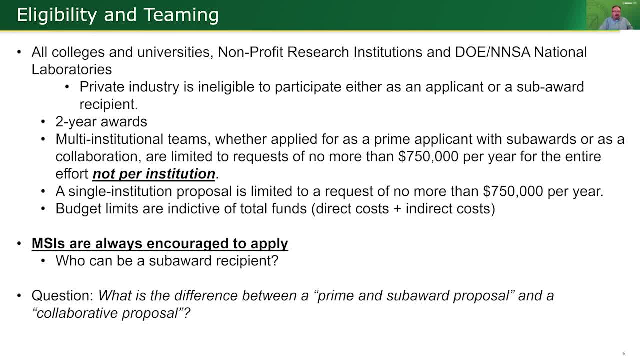 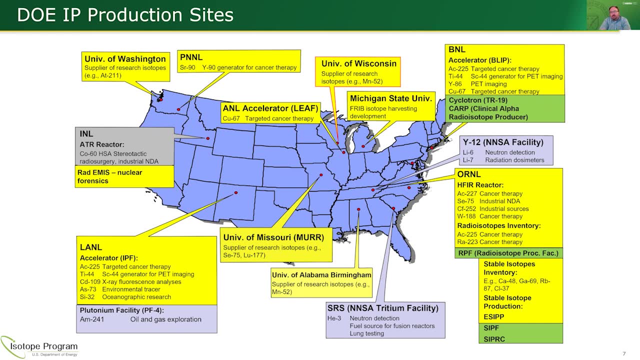 And if there are questions about that we can discuss. after the fact. It's kind of a complicated concept, but most people catch on pretty quickly, All right. So if you want to collaborate with folks, where are the sites that DOE Isotope Program utilizes to do the things that? 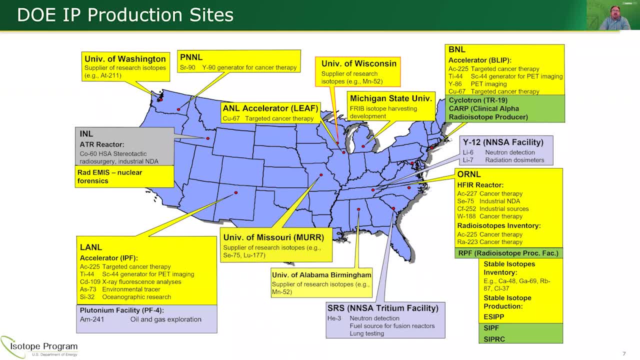 we do. You'll see in front of you a map of the US. You've got a mixture of national laboratories as well, as you'll see some academic research institutions. Those academic sites are part of what we refer to as the University Isotope Network. Those 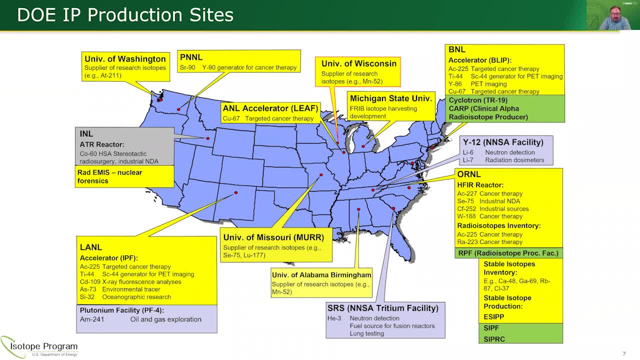 those network participants have unique facility as well as personnel that are are highly skilled at what they do and capable of carrying out routine isotope production, And we utilize those facilities and leverage them to make sure that the nation meets it's its isotope demands. 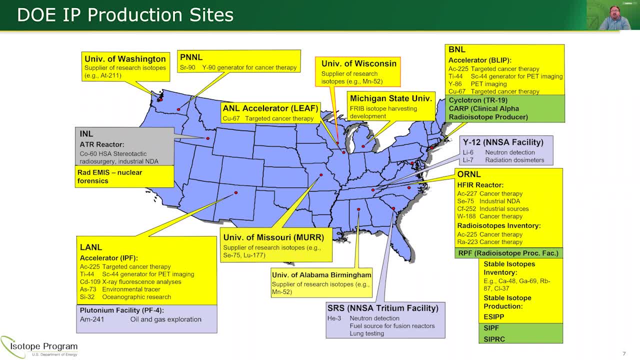 And we utilize those facilities and leverage them to make sure that the nation meets its its isotope demands. With respect to the national laboratories, we'll go through who they are, where they are and so forth in the next couple of slides. 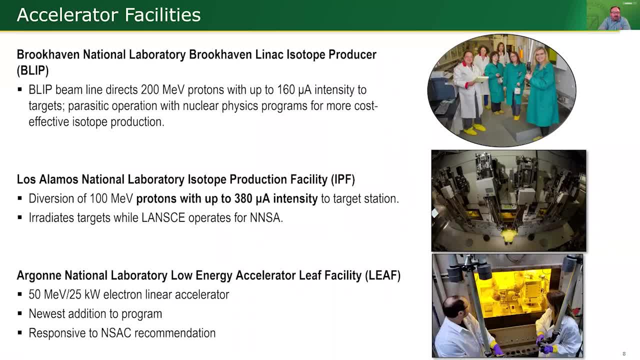 So accelerator sites, and we can split the national labs into three basic categories. You have accelerator sites, you have reactor-based sites and then you've got quote-unquote other isotope activities or other isotope production sites. So we'll start with accelerators. 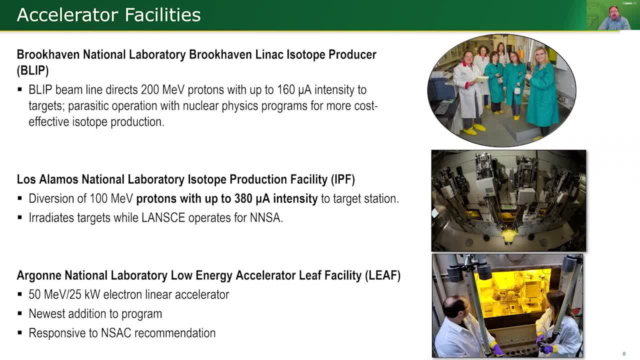 You've got Brookhaven National Laboratory. They have a LINAC isotope producer. It's a high-energy proton accelerator and you can see the beam characteristics of that site. The previous slide showed you some of the things that they're working on in terms of the isotopes they're producing. 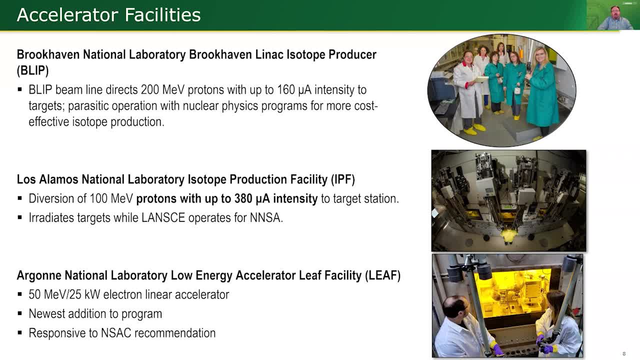 Similarly with Los Alamos, you have the IPF, which is the isotope production facility. So slightly less beam energy, But much higher current. And I should point out that these two sites run off-cycle of one another because both are proton accelerators. 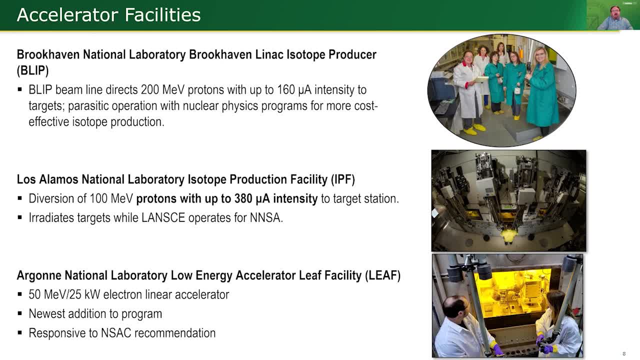 They back each other up. So when Brookhaven is producing, Los Alamos is down for preventative maintenance, and vice versa. We've also got Argonne National Laboratory with a low-energy electron accelerator And it's very, very high-energy And the beam profile is characterized in the first bullet. 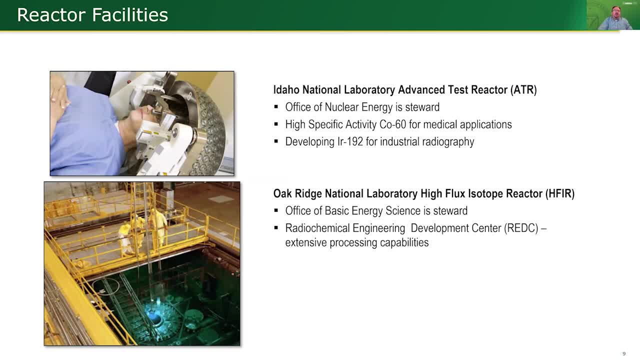 Right. Moving to reactors. We have Idaho National Laboratory's ATR, the Advanced Test Reactor, primarily used for production of cobalt-60, although there are other applications at Idaho National Lab that are either under development or being considered- And then by far the workhorse of reactors. 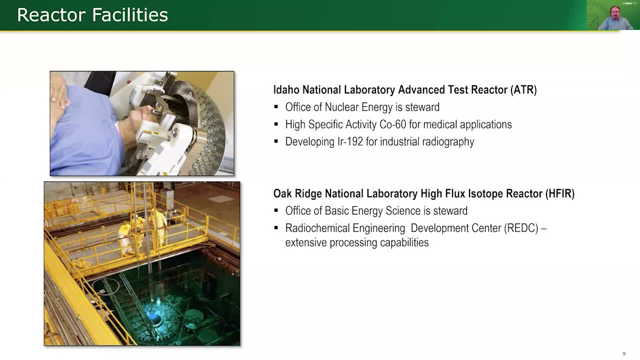 One of the most successful in reactor production within the portfolio of DoEIP is Oak Ridge National Lab's HyPher, or high flux isotope reactor, and the suite of processing facilities at Oak Ridge as well that feed into what their activities happen to be. 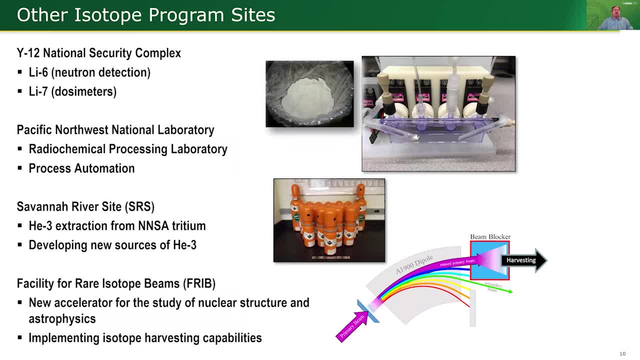 Some of these other isotope production sites. we do some work at Y-12.. Pacific Northwest National Laboratory has some work on this. We do some work at Y-12.. Pacific Northwest National Laboratory has some work on this. extensive expertise in process automation. 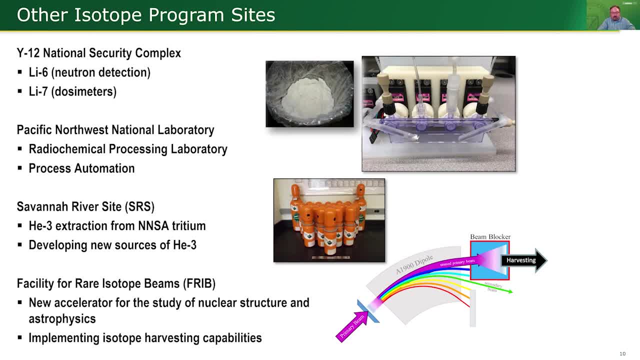 as well as conduct some separation science and dispensing. There are activities at Savannah as well as the newest of the scientific user facilities within the Office of Science, FRIB or the Facility for Rare Isotope Beams at Michigan State University, where those folks are actively engaged in R&D. 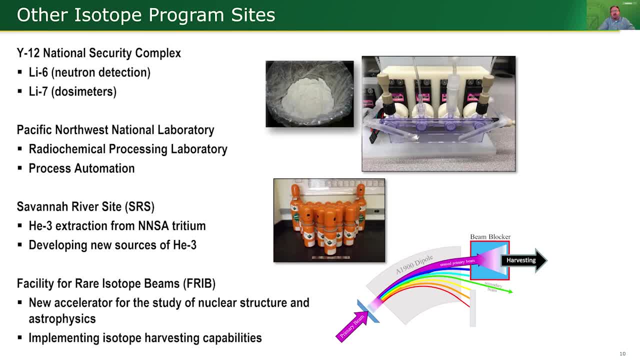 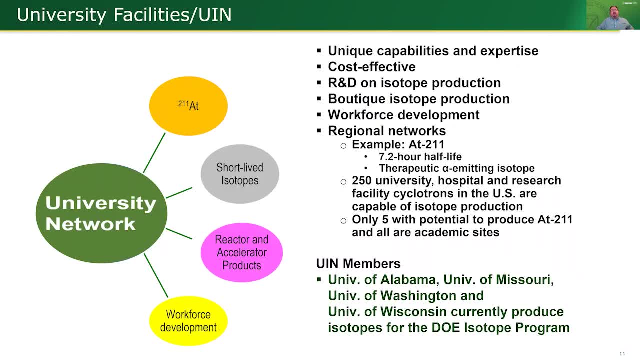 as well as implementation of isotope harvesting out of a bean dump and other areas. Okay, so I spoke briefly earlier about the University Isotope Network. There are some unique capabilities and expertise, as I mentioned, but this network was largely born out of the idea. 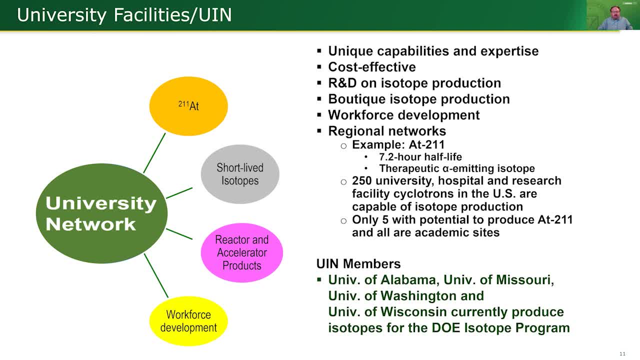 that there were certain cases where isotopes might either have a short half-life or be needed in smaller batches, these quote-unquote boutique isotopes, which would be better facilitated through universities than through trying to schedule batches at a national laboratory, which would just serve to increase the cost. 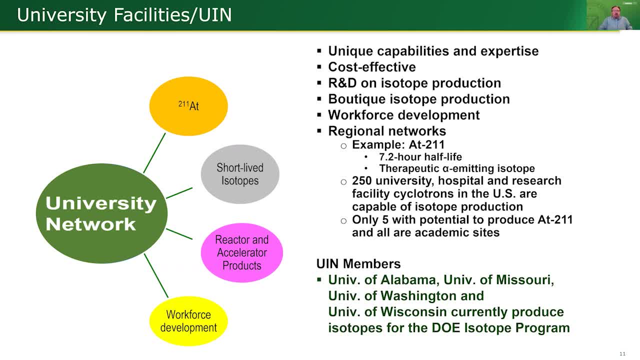 and or in certain cases, national laboratories might not have the correct beam to be able to produce them. Specifically, the case of Astatine-211 has come to mind, and that was the first one. That was the first isotope that we started. 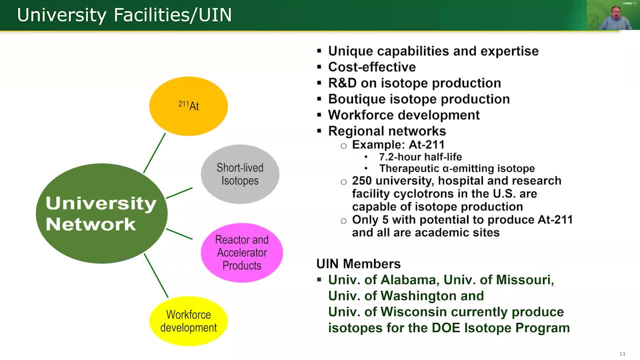 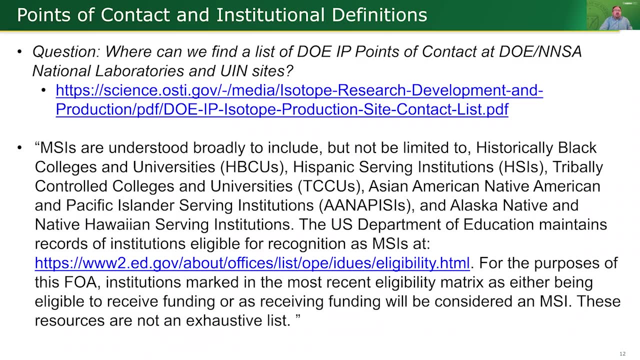 with the University Isotope Network. So those members are listed on the screen at the bottom and we can talk more about those if you have questions at the end as well. So the questions that often develop after seeing those first few slides are: where can you find points of contact? 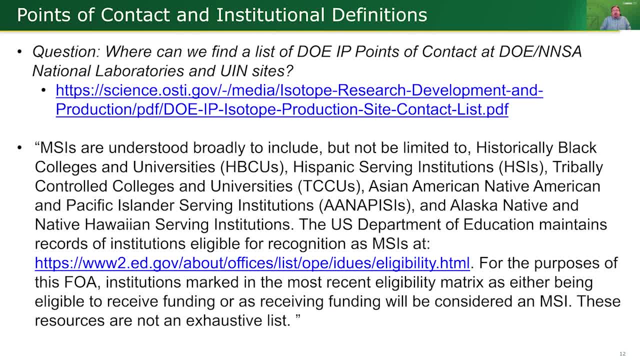 at the various labs and UIN sites. So there's a a hyperlink that's in the slide will also be in the chat and that's a point of contact list. You're free to reach out to those folks and they can best direct you to the people. 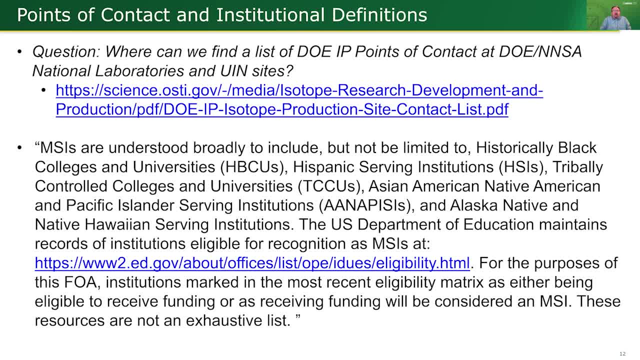 at their facilities with whom you might establish collaborations. There's also a list of who are currently identified by Department of Education as MSIs and the various, the various categories of MSIs that exist. That's that second hyperlink in the second bullet. 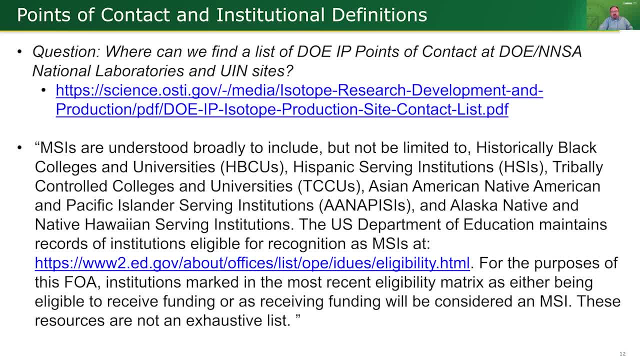 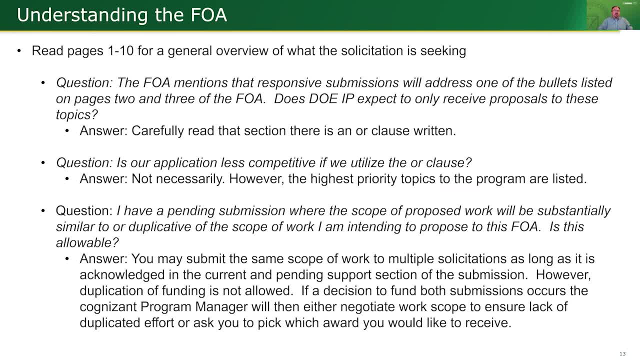 Encourage you to take a look there. That's the the most current list, although it's not exhaustive. Okay, so let's get truly into the meat and potatoes of the FOA. Where do you begin? Well, start with page one and read to page 10.. 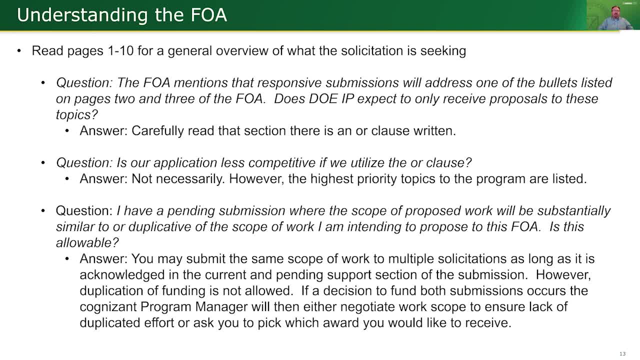 That gives you general flavor for the overview of what the solicitation is truly saying. So the first question is: typically the FOA mentions that responsive submissions will address one of the bullets listed on pages two and three. Does the isotope program expect to only receive proposals? 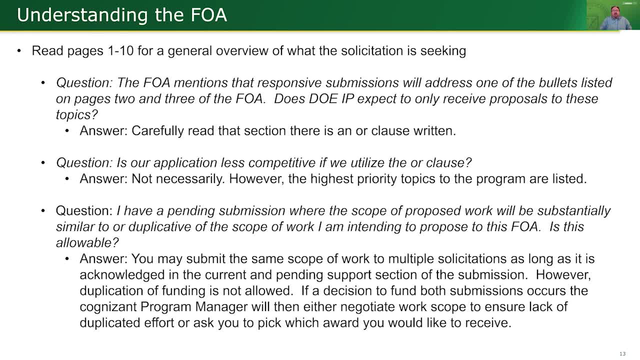 to those topics. So I would encourage you to carefully read that section, because there is a quote, unquote or clause written into there And that would then feed into the second question, which is: is our application less competitive if we utilize that or clause? 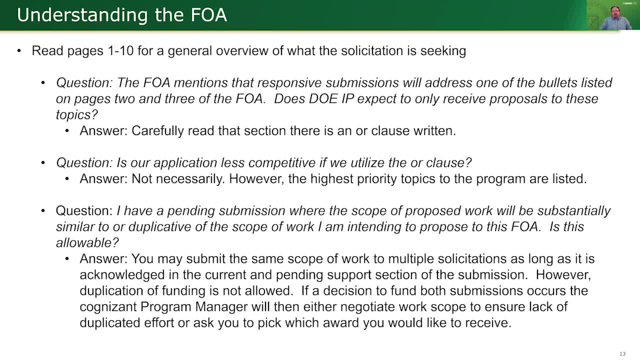 Not necessarily. However, I would point out, as is stated explicitly in the FOA, that the highest priority topics to the program are listed, And this is a good point to bring up this particular topic, which is read the FOA without interpreting anything. 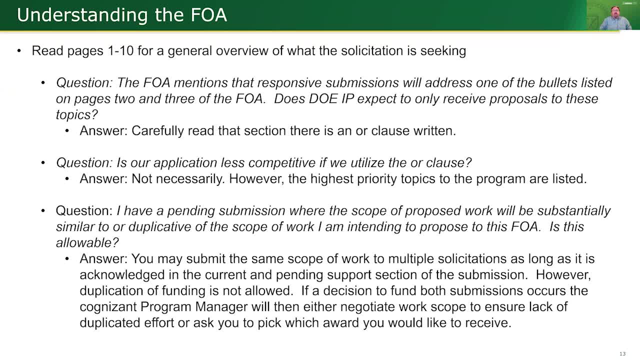 Take it at face value And if you have questions or feel like you need to interpret something, that's when you reach out to the program. But the FOA is written in a way to be very transparent and stated succinctly, All right. so the next question that I typically get is: 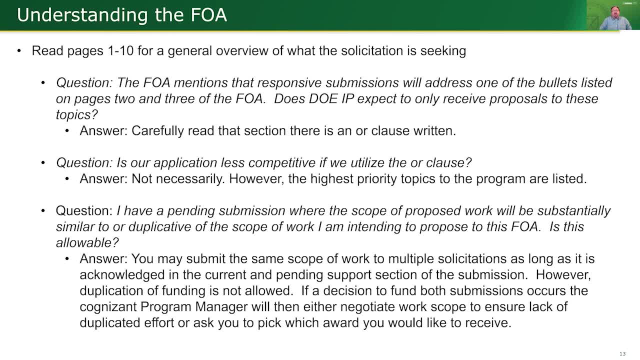 I have a pending submission where the scope of proposed work will be substantially similar to or duplicative of the scope of work I intend to propose to this FOA. Is that allowed? So the answer is: you can submit the same scope of work to multiple solicitations. 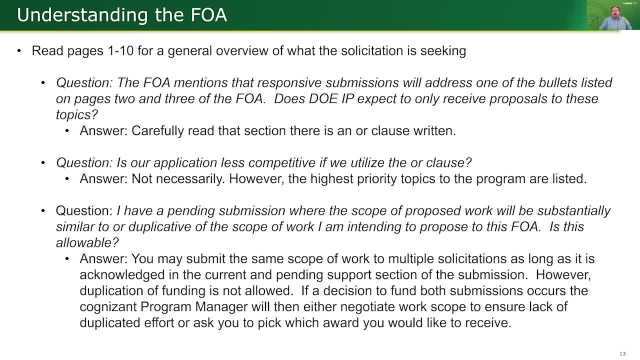 as long as you acknowledge it in the current and pending support section of your submissions. But duplication of funding is not allowed. So if the decision to fund both submissions occurs, then the cognizant program managers will reach out to the PI and either negotiate the scope of work. 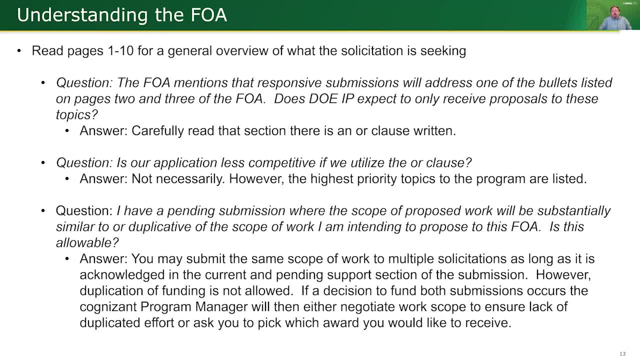 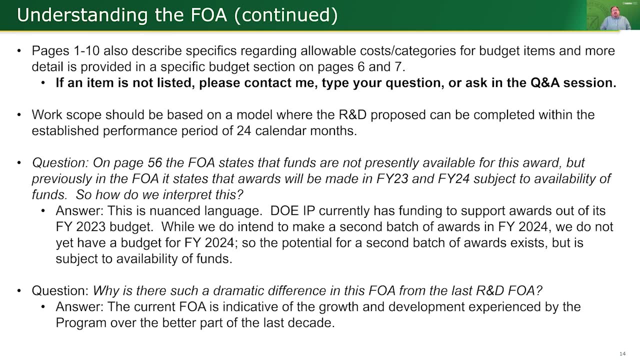 that's gonna be funded to ensure allowable duplication, or we'll ask you to pick which award you would like to receive, And that's another question that we can delve into a little bit more if you'd like. So pages one through 10 also describes specifics. 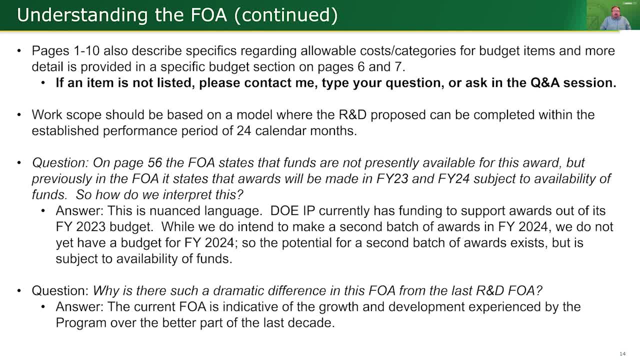 regarding allowable costs, slash categories right, And those allowable costs and categories have dramatically increased in the past couple of fiscal years. I really encourage everyone to take a look at them. You can find them specifically laid out on pages six and seven. If an item is not listed, 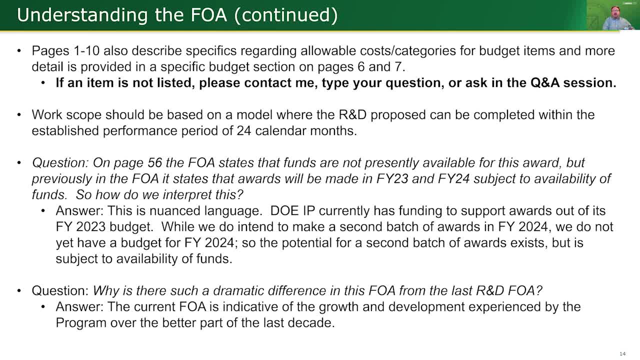 contact me or type your question into the chat, because it's not an exhaustive list, but it's worth asking if you have an item that you're thinking of that isn't listed. Okay, So what next? Well, your work scope should be based on a model. 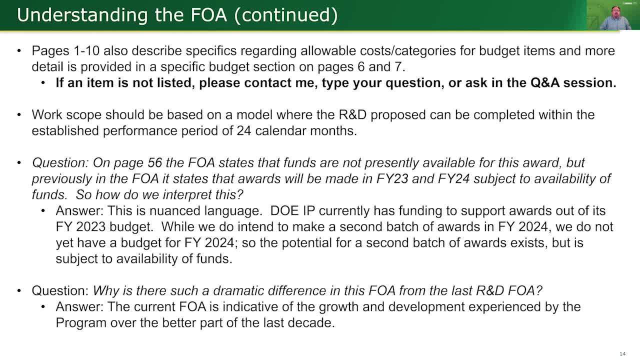 where the R&D that you're proposing can be completed within the established performance period of 24 calendar months. You know it should be a book-ended scope of work that you reasonably think you can complete. So that's a standalone statement. The next question is probably going to be based: 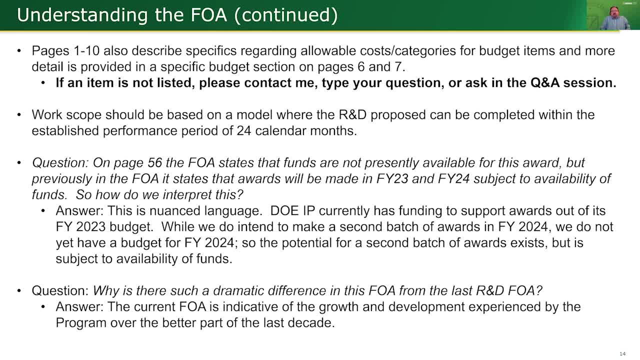 on something that you'll read, And on page 56, it states: the FOA states that funds are not presently available for the award. But previously in the FOA it also states that awards will be made in FY23 and 24.. 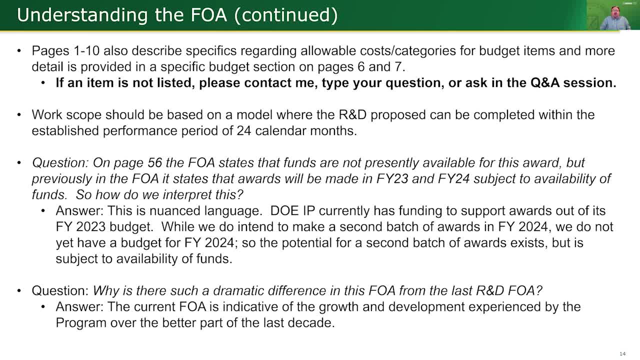 So, and we also state that it's subject to the availability of funds. So how should one interpret that? So it is nuanced language. Our intent is to make a batch of awards using our FY23 appropriation, which we currently have Subject to available funds in FY24,. 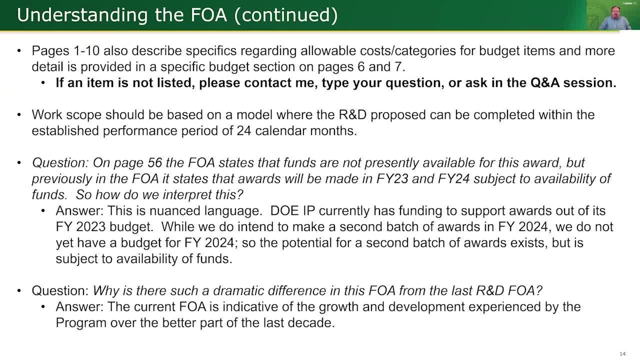 we'll make a second batch of awards, But we have no idea what the magnitude of that budget is yet. So that's why the second statement sort of appears, but it's not to say that anything has changed, So it shouldn't be taken as conflicting statements. 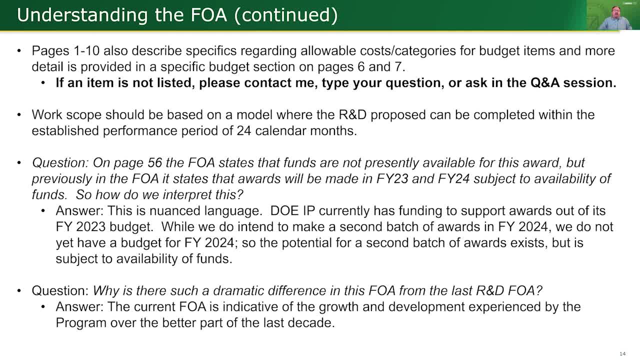 All right. next question: Why is there such a dramatic difference in the appearance of this FOA from previous FOAs with respect to what DOE IP used to send out in R&D? Well, it's kind of indicative of the growth of the program. 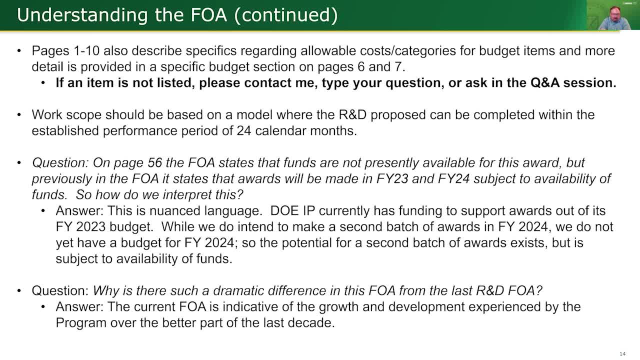 And develop development of a very robust program of research over the better part of the last decade. When the FOA was initially released, in the first part of, I want to say, 2011,, there wasn't much in the way of the availability for the community to seek R&D to engage in isotope. 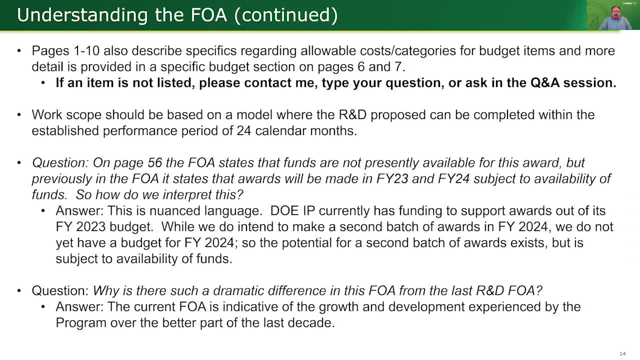 production-related activities. That's changed thanks to the FOA, thanks to other funding opportunities as well, And we now find ourselves, as a program, in a situation where the swimming pool is vast and we needed to establish some swim lanes. So, in an effort to be transparent, 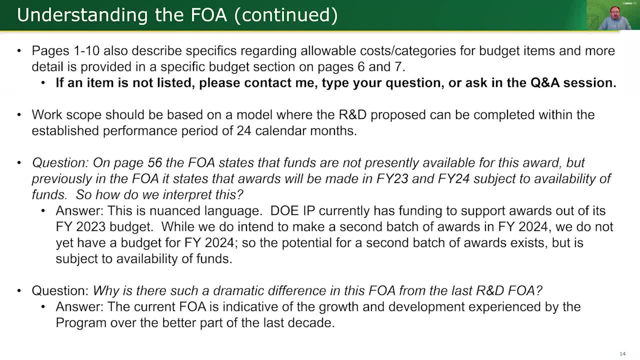 we established priorities that are listed within the FOA, and that's what's driving this, Recognizing, of course, that there might be things that you can think of that aren't listed there, which has that or clause as I described, but it's still got to be relevant to the program. 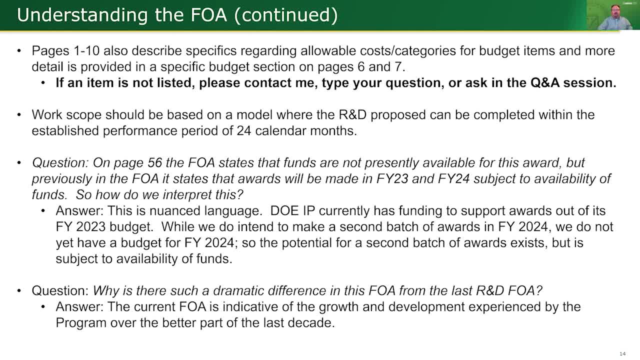 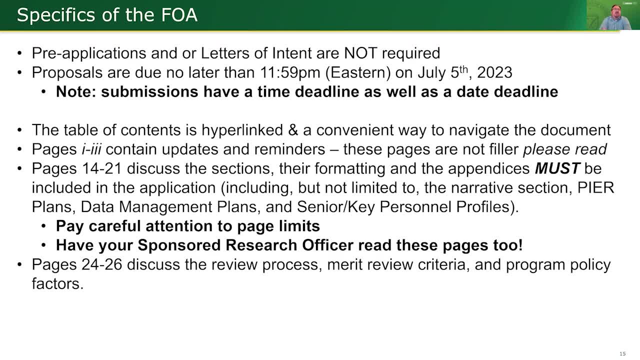 So I think that that stands on its own All right. so specifics of the FOA. There are no pre-applications or letters of intent that are required. Proposals are due no later than 1159 pm Eastern time. Please be mindful of the time zone as well as the dates. 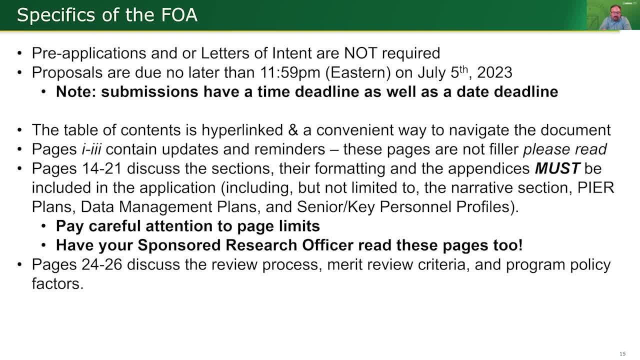 because once that window shuts, it's shut. The table of contents in each of the FOAs is hyperlinked within the document, So clicking on that is the most convenient way to navigate through. I'm going to go back to what could be a 100-plus page document to get to the correct section. 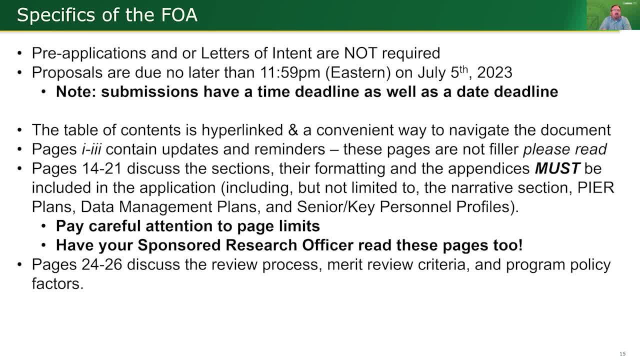 I don't need to read all of these bullets to you. You should concentrate on pages 14 to 21.. That's where the majority of the sections that we anticipate seeing in a responsive proposal can be found. It also discusses formatting and the appendices that must be included. 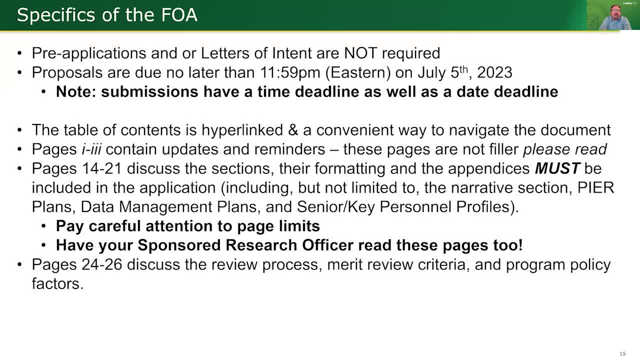 So make sure to capture the things that are listed there and pay careful attention to page limits. It's also a very good idea to have your SRO read those pages as well, because sometimes they catch things that you might miss. Pages 24 to 26 discuss the review process, the review criteria. 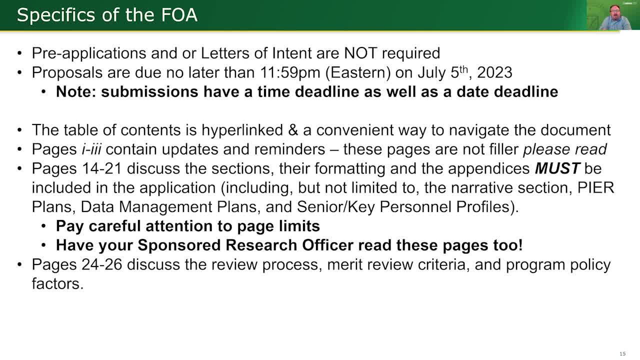 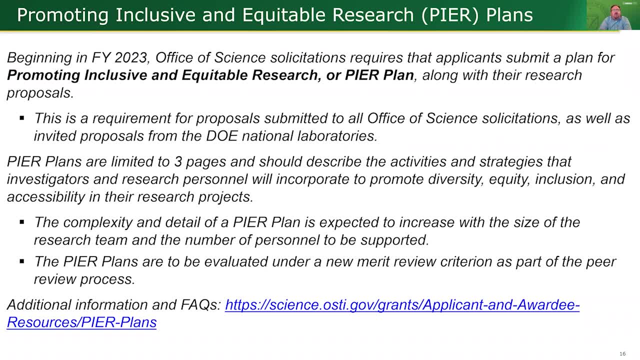 as well as program policy factors that may be applied. And I'm going to say one thing about peer plans, and that's beginning in 23,. so this particular fiscal year that we're currently in The Office of Science has begun to require what we call 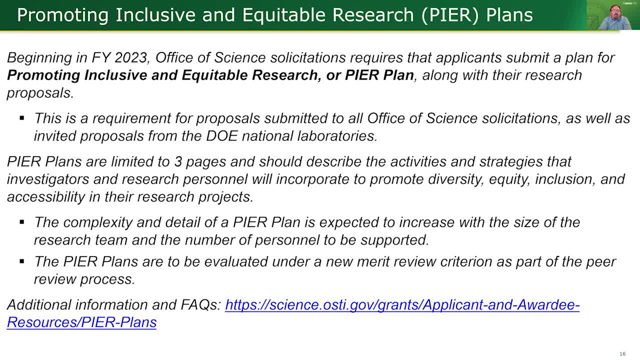 promoting inclusive and equitable research or peer plans, along with research proposals. They're to be included as appendices and you'll see requirements listed in the FOA, as on the previous slide. These are requirements for all proposals that come to SC solicitations. There are page limitations. 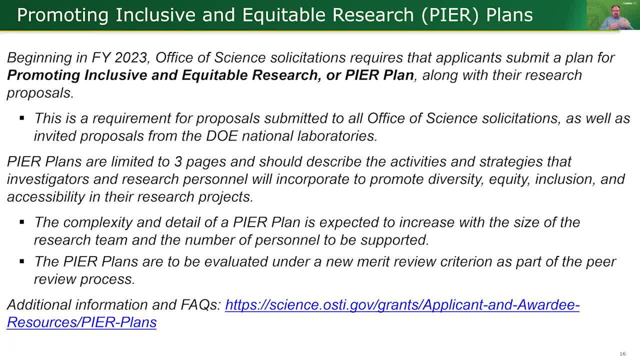 There are various components that we anticipate seeing, but a peer plan from solicitation to solicitation can vary dramatically and it should be tailored to the the actual solicitation that you're dealing with. Um, there are some guidelines that could be found if you use the link that's listed on the bottom lines of this slide. 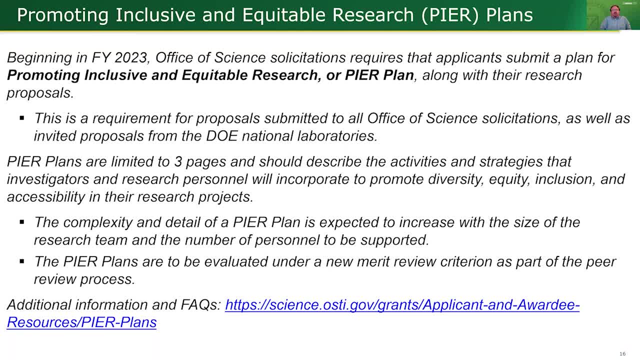 and it'll give you, hopefully, a good feel for what's anticipated to be submitted and what the reviewers will be looking for. Alright, I'm going to stop sharing because I've exhausted my time here, so I'm going to stress you out on our next slide and click retard for another one for your si시. 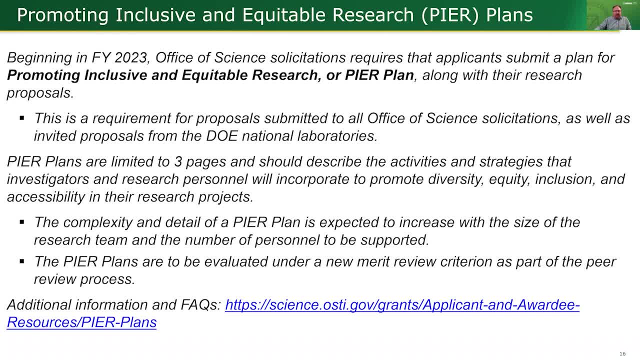 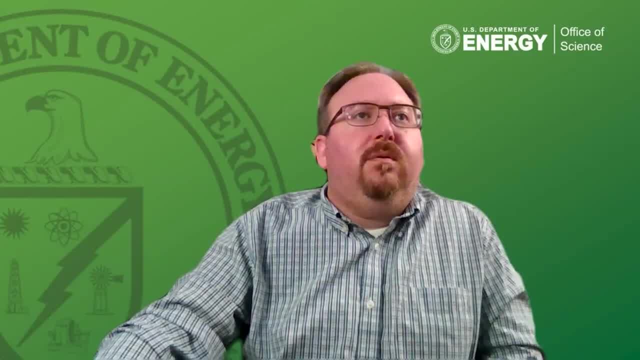 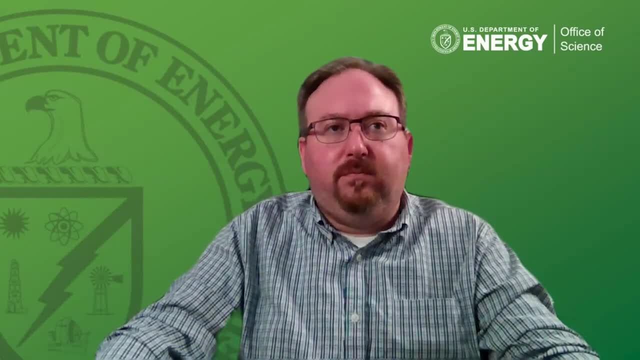 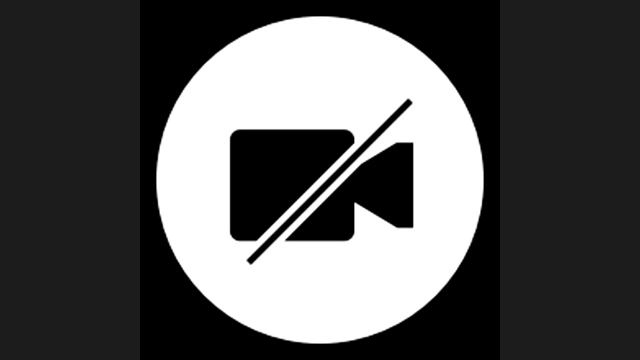 Whatever slide deck at this point And we can take questions. So, Ethan, we've had just a few questions in the Q&A, So just a reminder. please, if you have questions, go ahead and type them in in the Q&A section at the bottom of your screen. 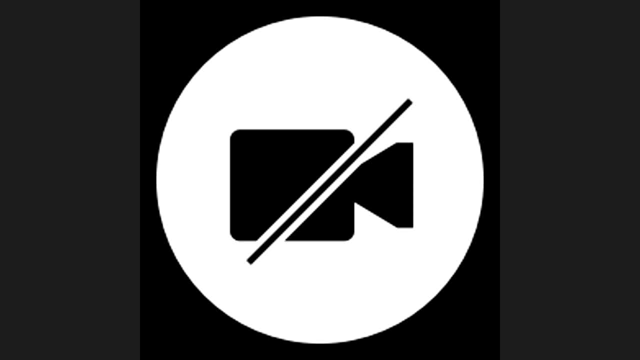 Just a reminder that commercial entities cannot participate in this FOA And that is due to the isotope program is prohibited from competition with the commercial isotope industry. The slides are already posted. I have put the links in the chat. If you're having trouble reaching those, just let us know. 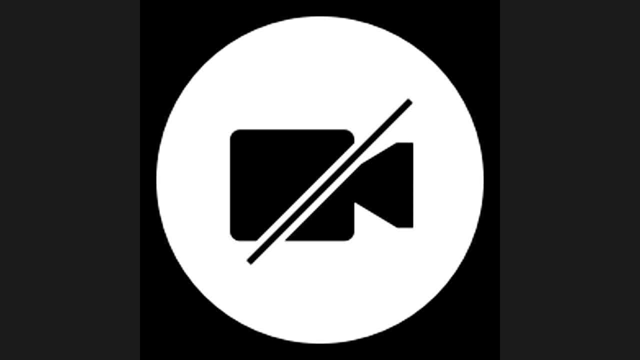 I also put the links that Ethan mentioned with respect to minority-serving institutions and the promoting inclusive and equitable research. Those links are also in the chat for you. So we do have a question, Ethan: How many proposals may we submit as a primary or co-PI? 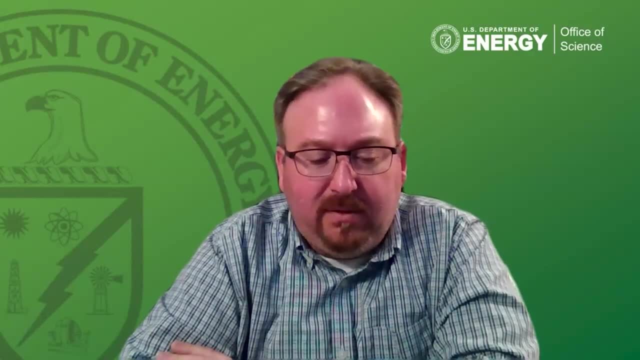 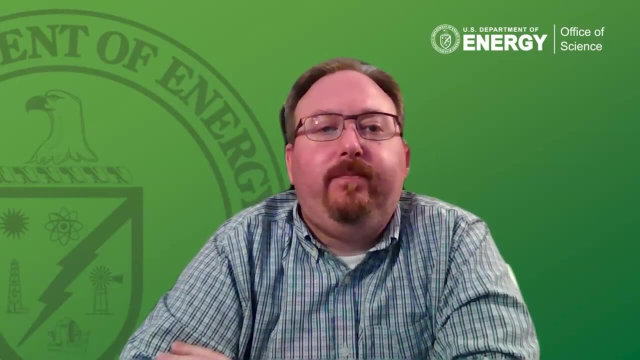 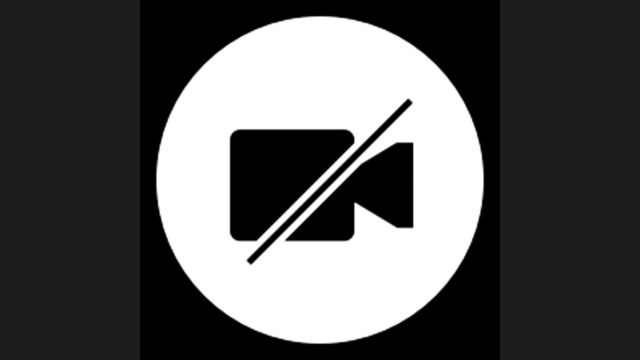 Very good. The DOE isotope program does not limit the number of proposals per institution or per PI. Okay, Another question. There are some- I'm assuming- trigger reactors not shown in the slides. Would you like to see them to apply? 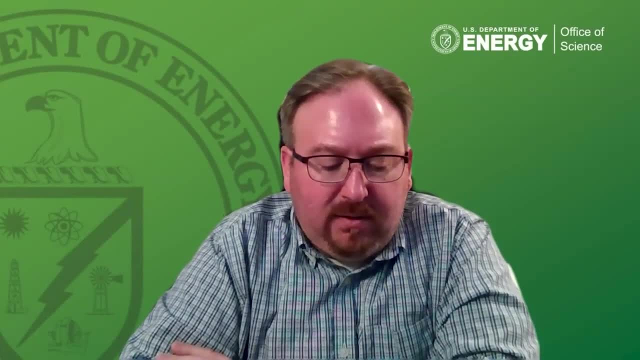 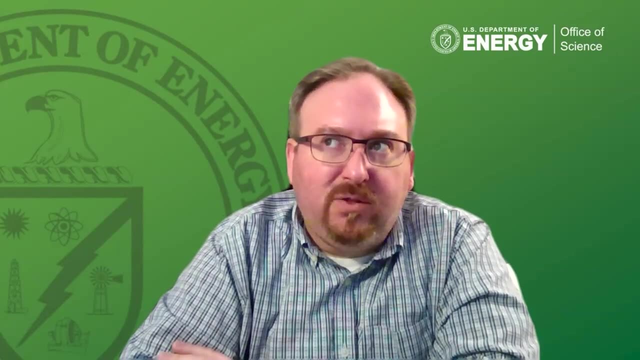 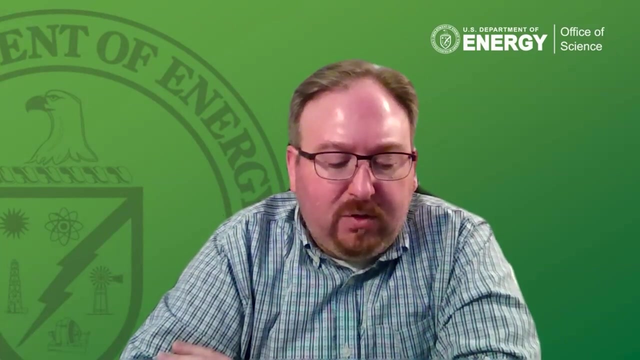 The reactors that appear in the slide deck, as I stated, are solely those which are members of our university isotope network, And that's why there are other university-based reactors and other university sites that aren't on that map As to whether or not a facility, as to whether or not. 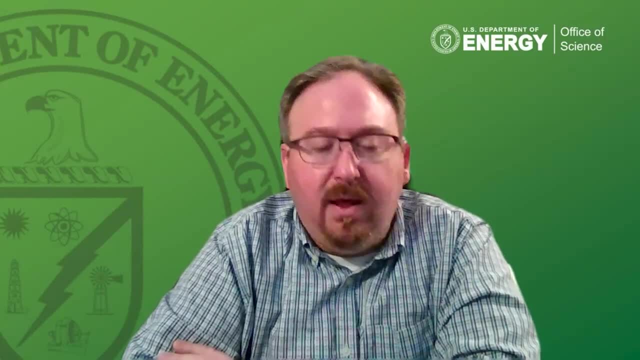 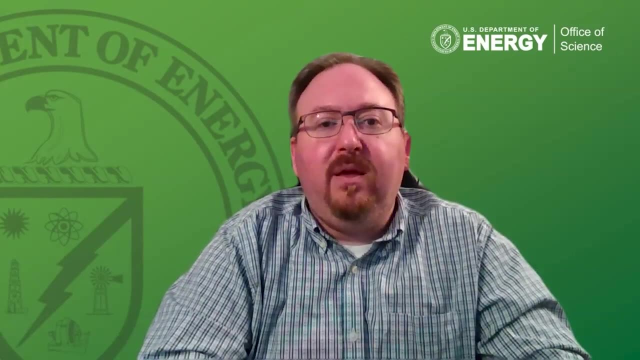 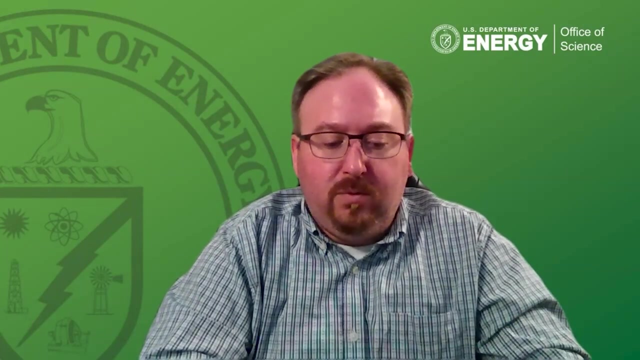 the isotope program would like facilities to apply or not. we would like to see the solicitation to provide an opportunity to the community to seek R&D funding If you have a compelling idea and you'd like to throw your hat into the competition. 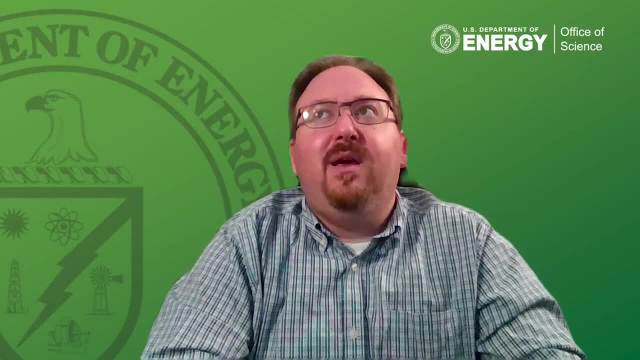 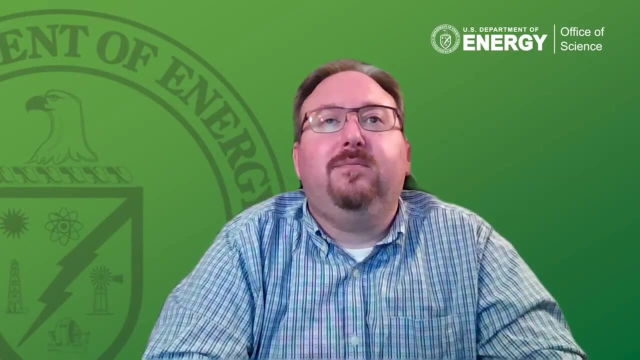 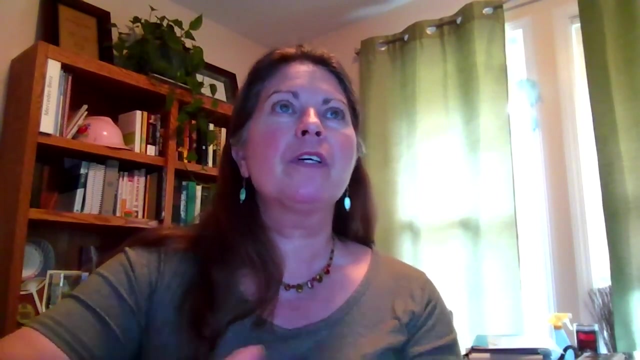 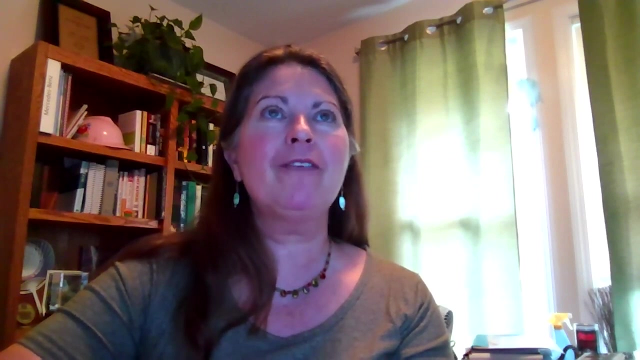 we encourage applications from all entities as established under the eligibility criteria. I apologize, I didn't have my camera on, So this starts out with thanks for the information. We will all read the provided document carefully. The title of the FOA covers a lot of ground: R&D, development and training. What does the office 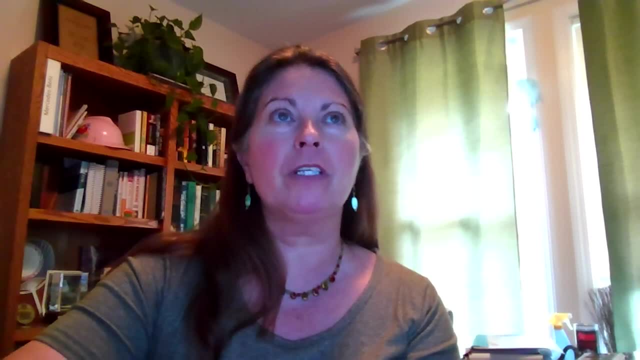 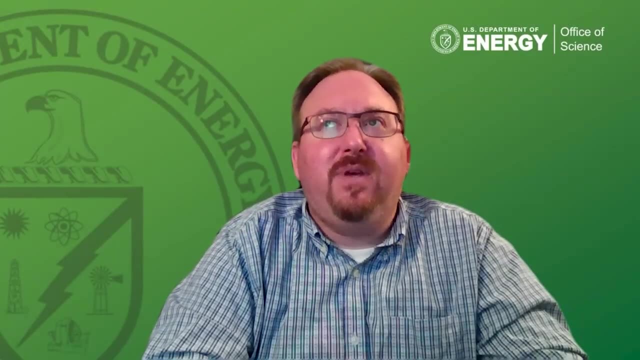 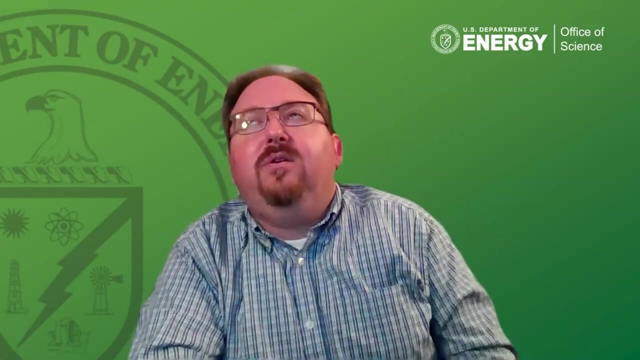 anticipate in terms of focus for competitive application, Will applications need to touch on all three? So I would suggest that you take a look at pages one through ten Compelling applications. I mean you'll see in the, not the summary section but the general section and pages. 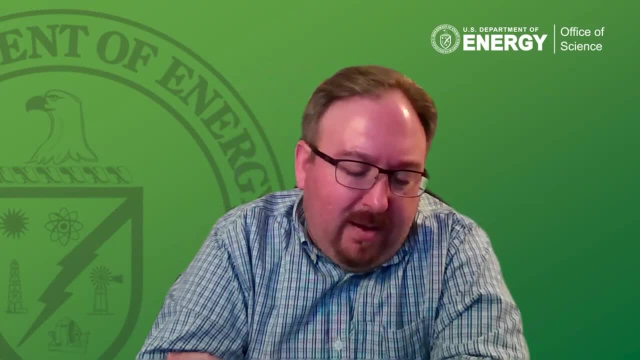 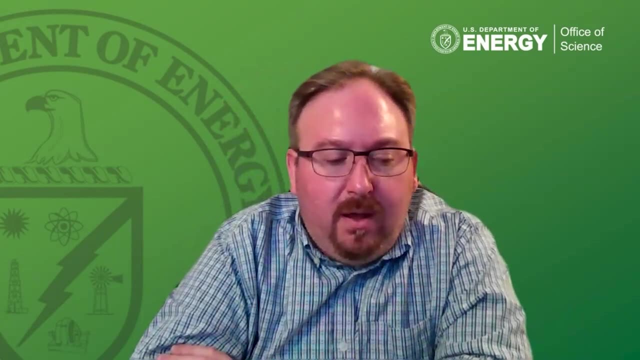 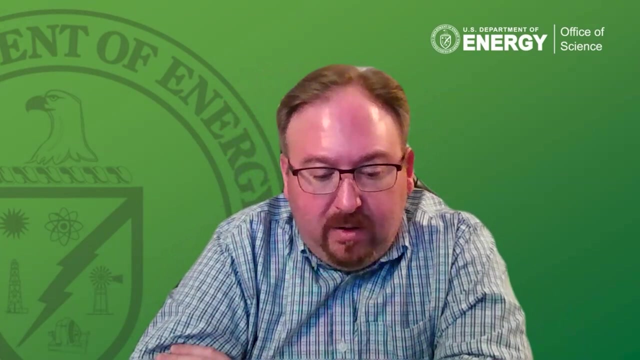 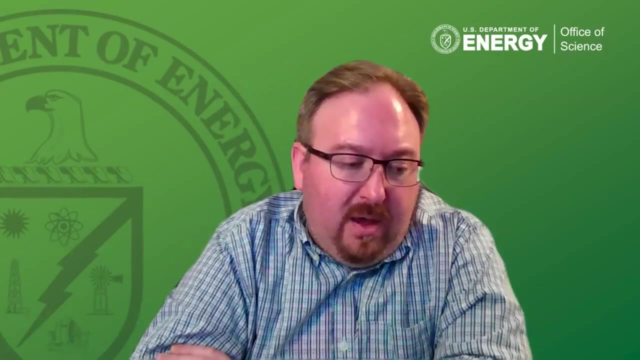 oh, I believe it starts on page two or three where it specifically lays out the FOA. There is some language in there that describes that competitive applications typically include training as well as other aspects that the program considers to be high priority. As to whether you have to touch on all three aspects, 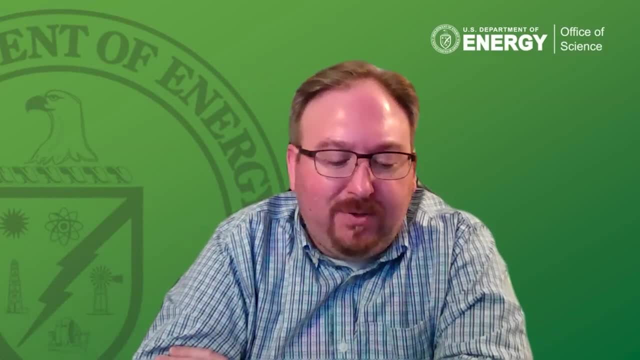 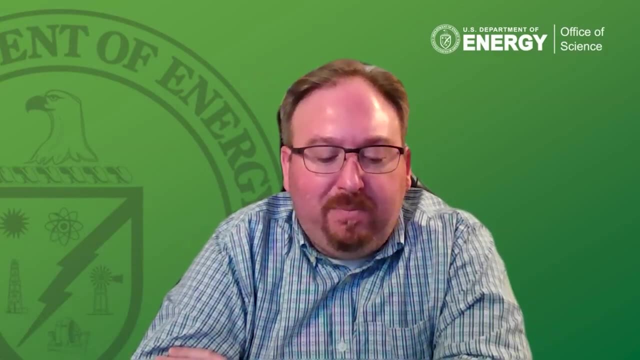 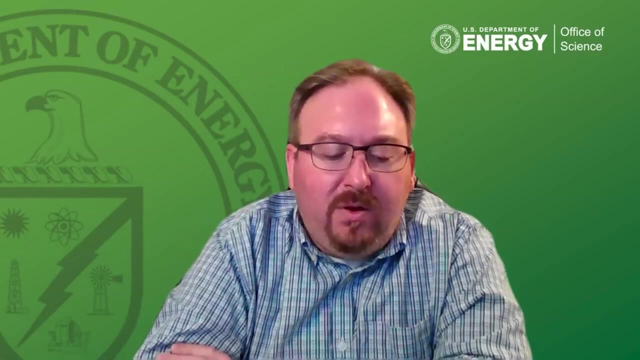 I think that's something that each PI will have to discern for themselves- And you can. it should be fairly. it should be fairly plain in terms of of what we are seeking When you read pages one through ten, And then again fourteen to twenty-one. 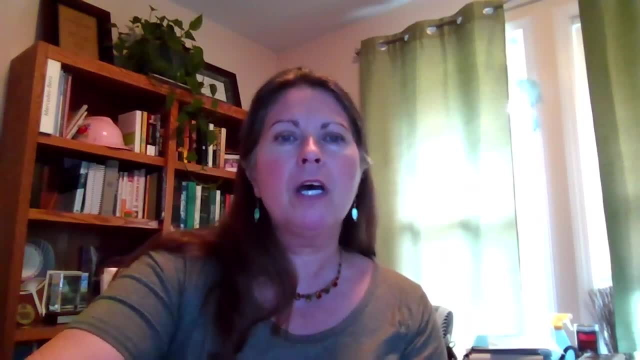 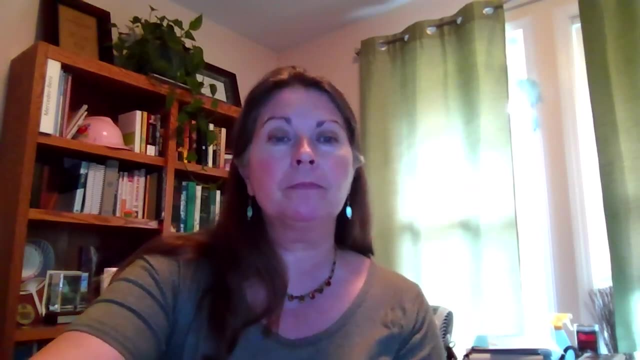 The next few are kind of in a similar vein but slightly different. To what degree will the emphasis on fundamental research versus applied research impact the success of the proposal? Ah, okay, So as a as a program office within the Office of Science, DEE, is the students to all work, work in five routines? The United States isicamente ashore element of node research in both speciesemporally and centrally, To understand should the field or an amiability-based overall to a, a Madmenuga or an aligned approach with a CPA, is not a do doing at all. 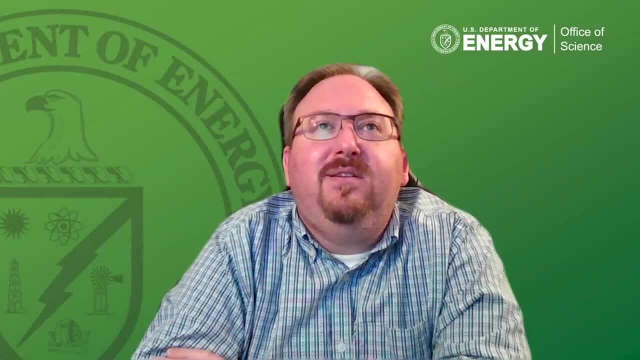 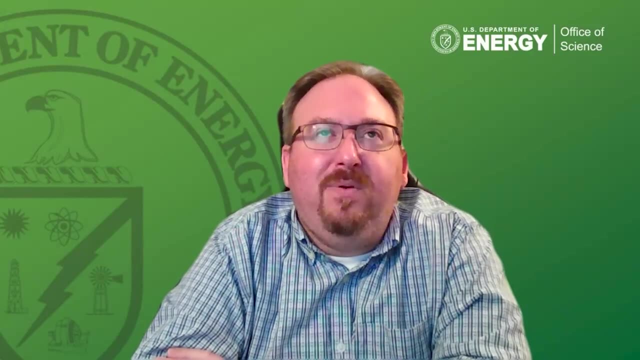 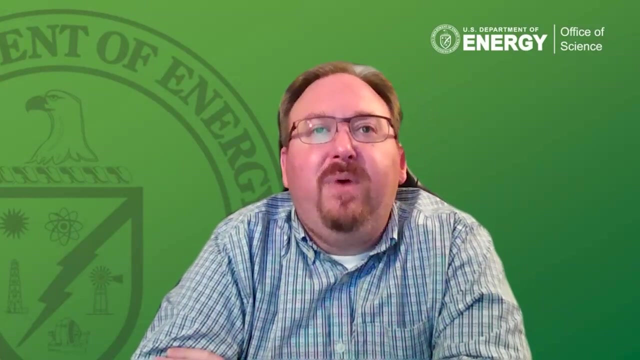 as a program office within the Office of Science, DOE only funds basic science research. We do not fund applied research. If you want to make an application for applied research, that's a different funding agency. The work that the isotope program funds is considered basic science. 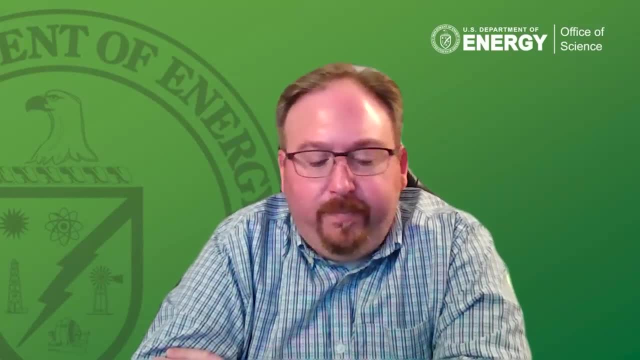 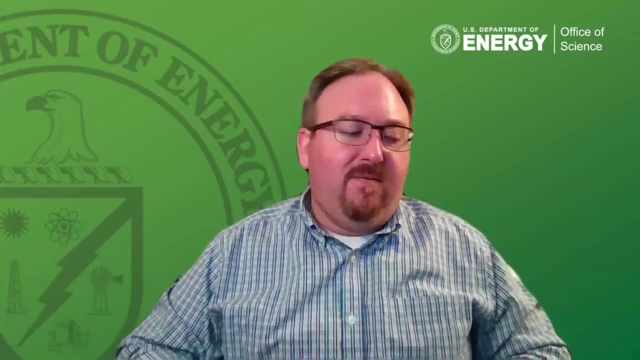 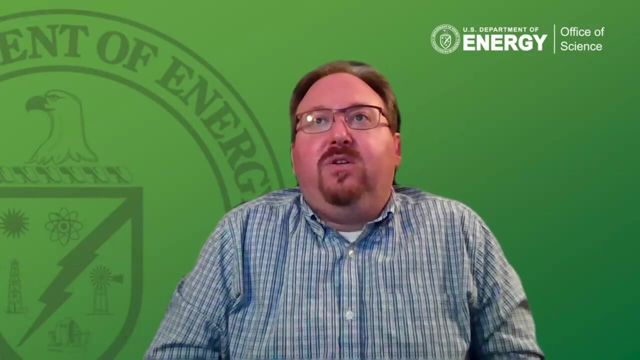 up to a certain point. So you know I have to make certain assumptions here. I'm going to assume, for the sake of argument, that the researcher in question was considering potential medical application, in which case there is a clean line that is drawn between where DOE funding would have. 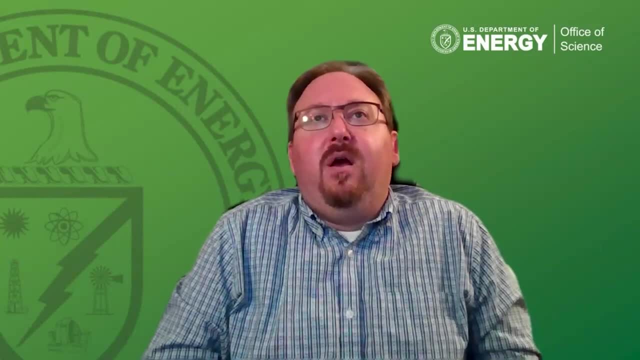 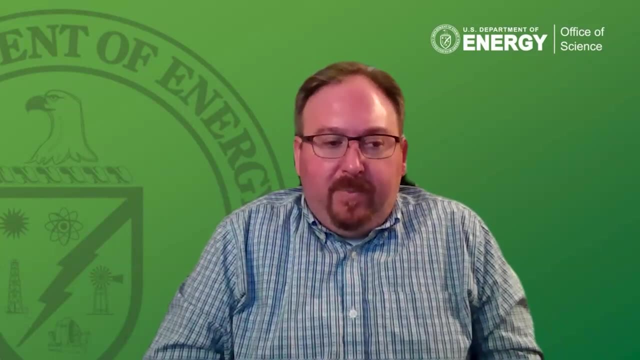 to end and where NIH or some other funder of biomedical-based research would have to begin, And you know that typically occurs at or near the end of the year. So I'm going to assume that the isotope program funds basic science. 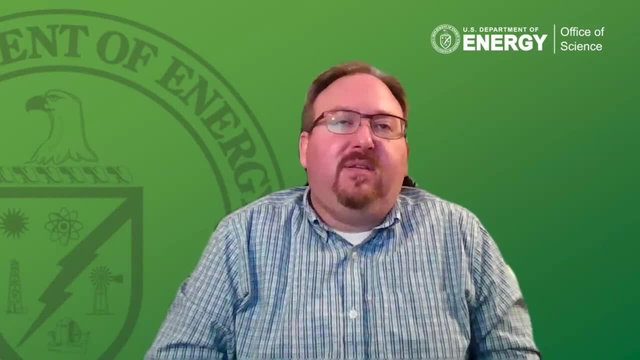 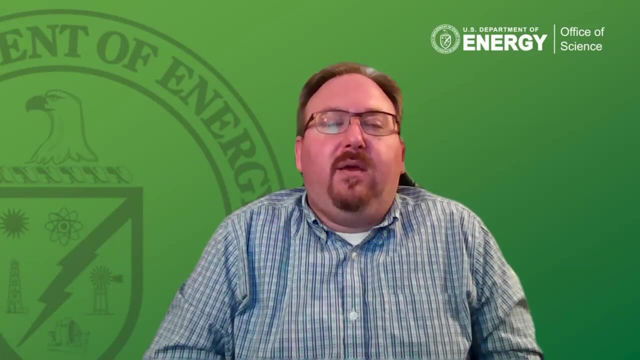 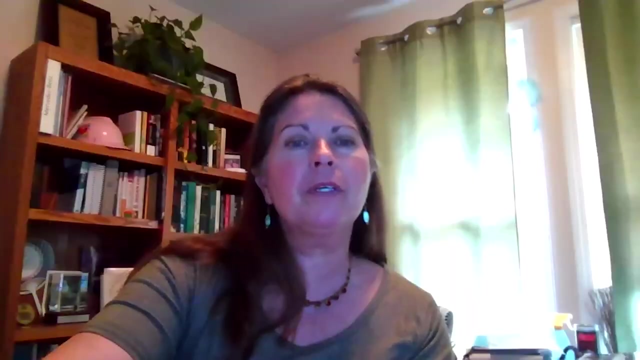 the question of efficacy in a living system. I can discuss in detail if the person wants to reach out. Next one: Would the research on particle beam sources listed as an R&D point in the FOA also include the development of a mass separation capability with an offline 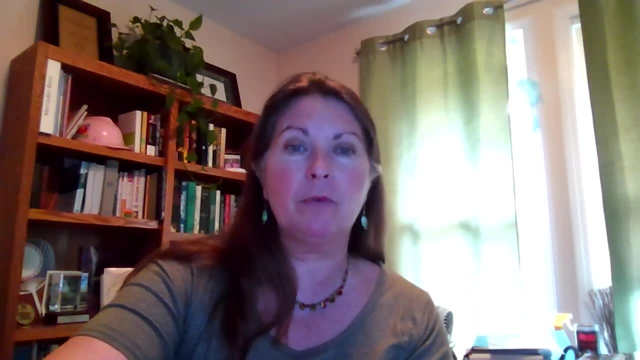 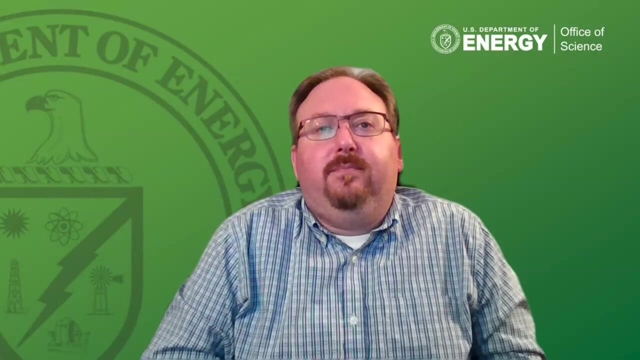 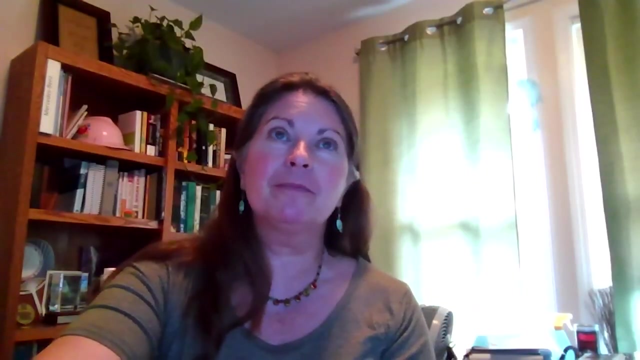 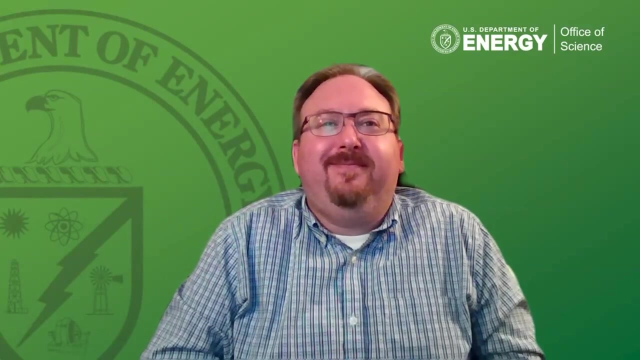 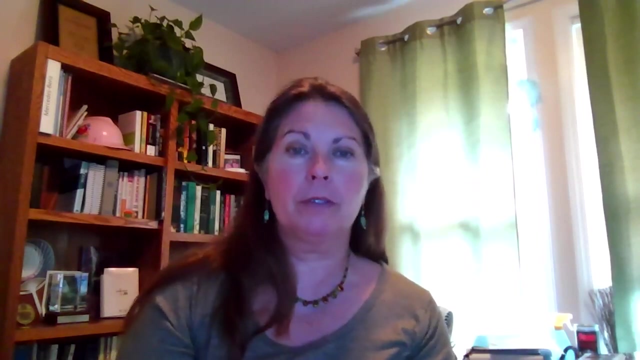 ion source to produce high-specific activity radioisotopes? Potentially, yes, Are high-risk ideas encouraged? Absolutely. The DOE isotope program lives on high-risk, high-reward research. The data is currently being used by the NIH, the NIH's and other. 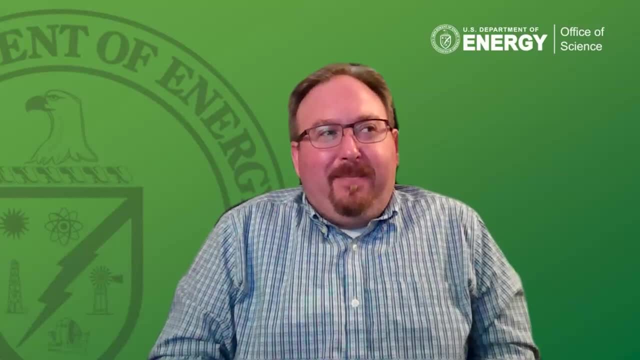 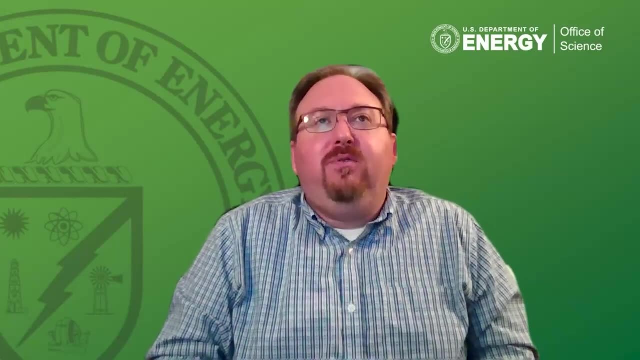 synthetic researchers and their partners in the field to help facilitate the development of innovative, highly-experienced and innovative solutions. Can the proposal exclusively revolve around cold work? That's a double-edged sort of a question, if I've ever seen one. So potentially, yes. You know, if you're an emerging research institution and you don't have your research institute, have a research institution or a research center or a research center or one of your research institutions and you don't have the capacity. 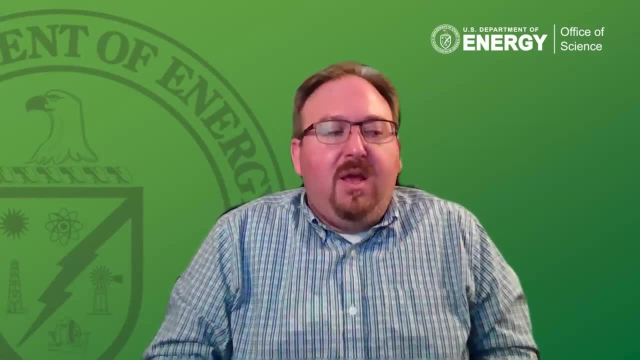 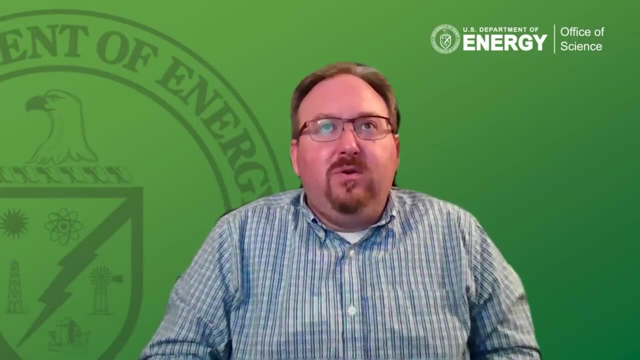 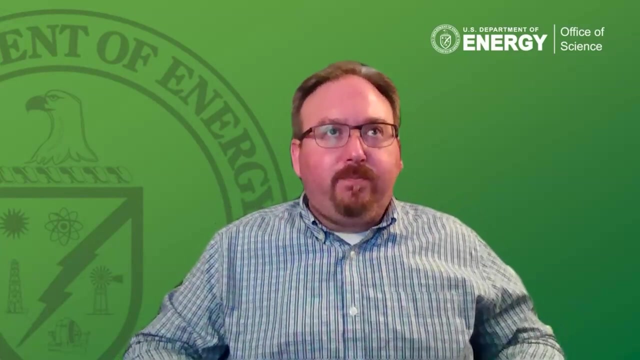 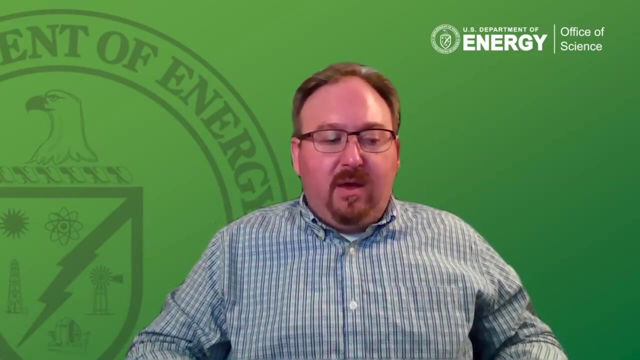 your university, your institution does not have a license to possess radioactive material, but you can fundamentally do quote-unquote surrogate science on a quote-unquote cold isotope of the same element and that fits the needs and addresses the nature of the work that. 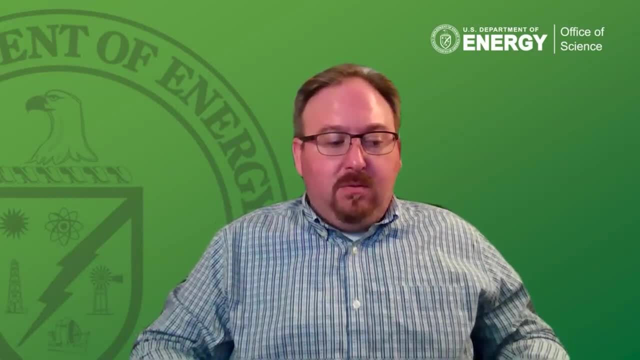 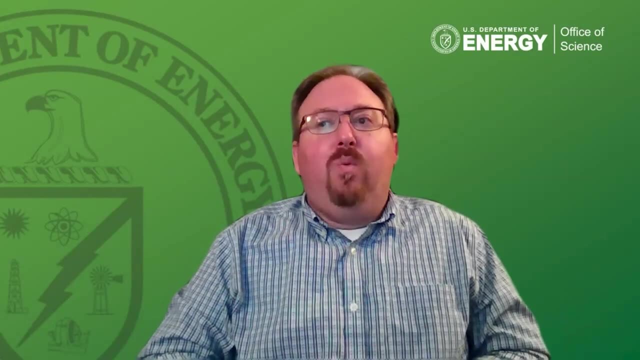 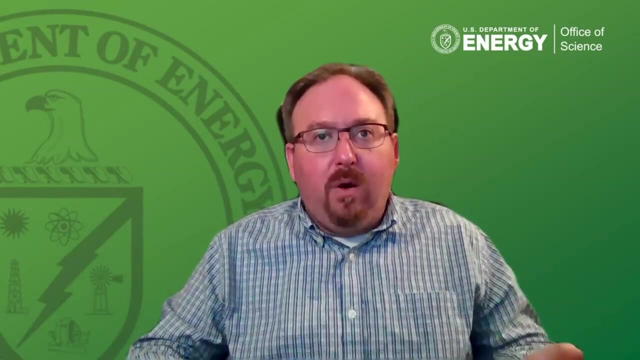 you're proposing and you know, as long as the reviewers don't have a problem with it, I don't have a problem with it either. At some point one would anticipate that it would translate over to quote-unquote hot work either at the site where the work was first proposed. 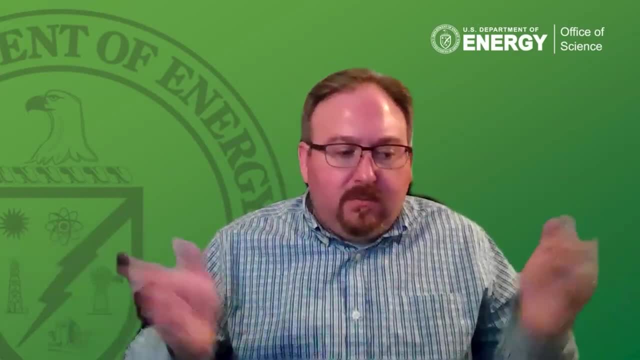 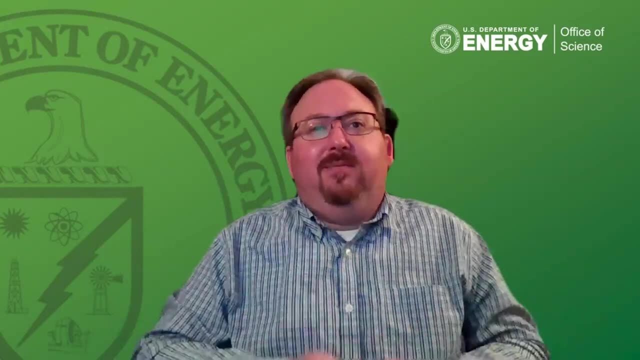 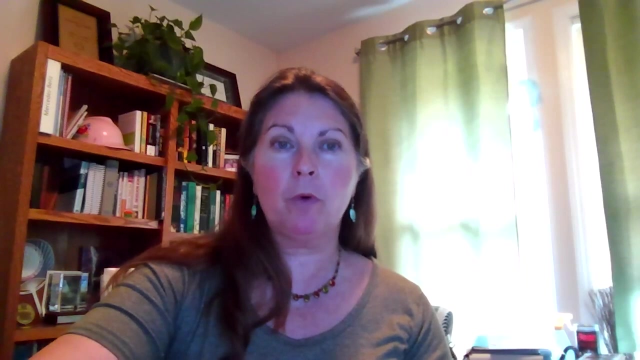 or via collaboration, and that's for the PI to decide. but at some point we would prefer, if it's going to be hot, that we see hot work For the separation of radium from uranium and thorium ores. is it sufficient to separate the? 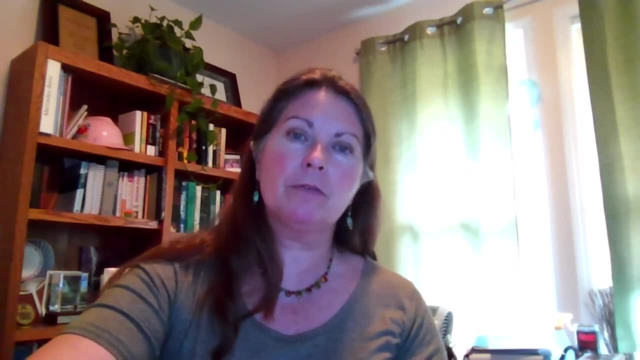 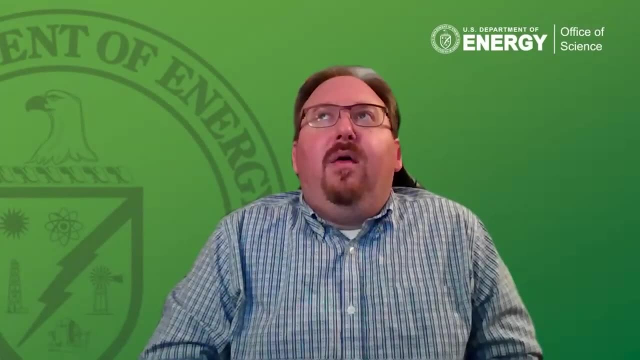 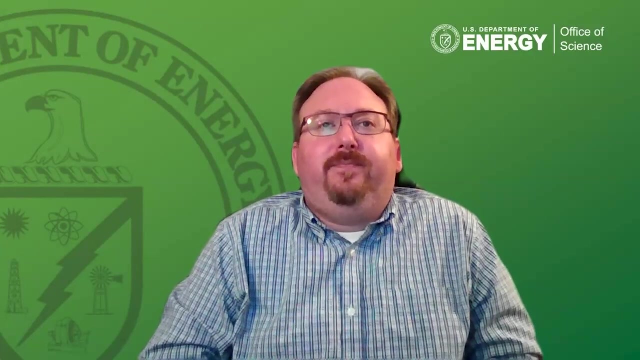 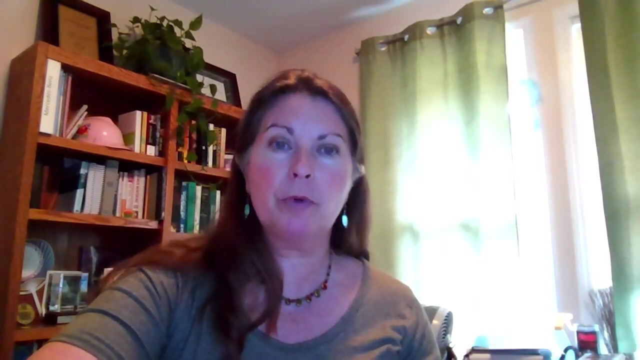 element or must the separation target specific isotopes, for example radium-226?? The question is up for the PI to decide. Both would be acceptable. Does the current FOA focus solely on production, or does it also consider separation? 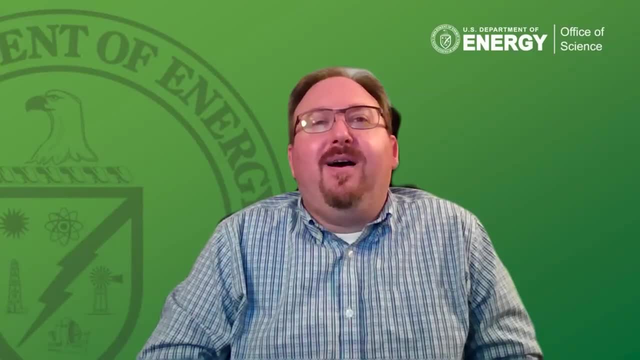 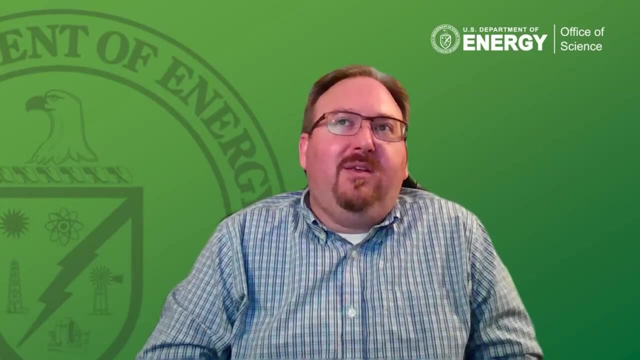 I suppose I have to ask the question: in what context? right, Because separation science is part of processing. Processing is what happens post-production. Unless- well, yeah, Unless- you're considering separation, you're not going to be able to do that. 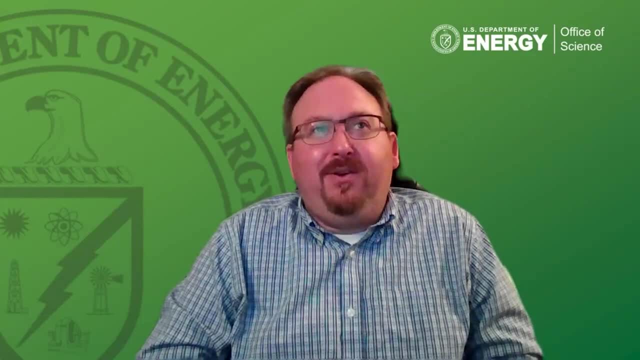 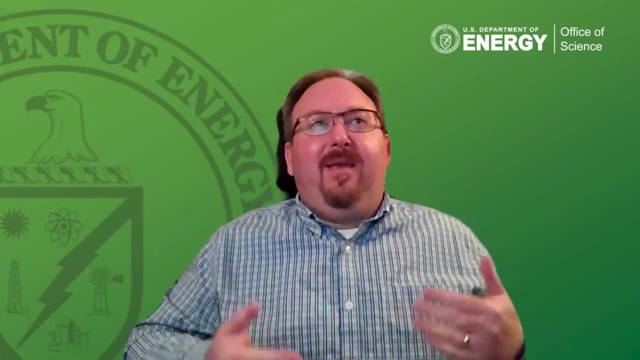 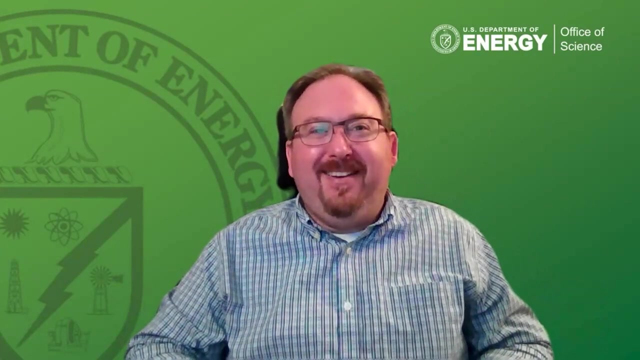 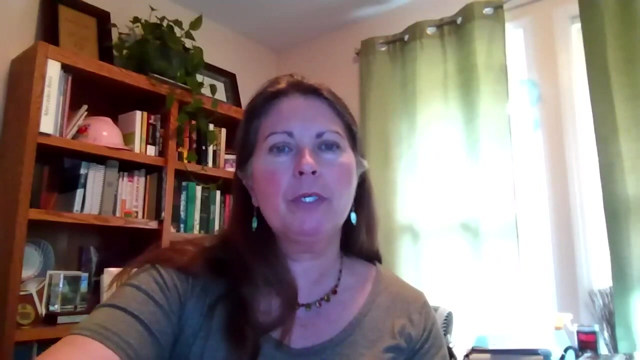 Unless you're considering enrichment, in which case separation is quote-unquote production of your enriched isotope. So I suppose the answer to the question is yes. right, It's got to focus on everything, all aspects. Is there someone we should contact to advise on some of the proposed ideas before the deadline? 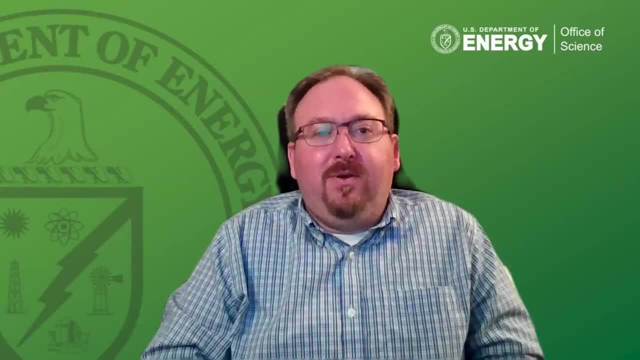 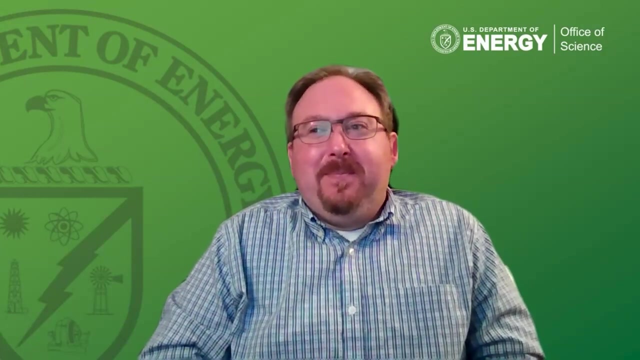 the technical contact You can reach out to me. My information is located within the body of the FOA, I believe on the first couple of pages as well as the last couple of pages, because we bookend things. Yeah, so you can reach out directly to me. 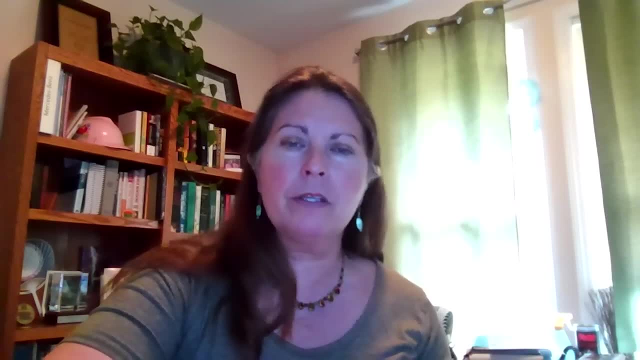 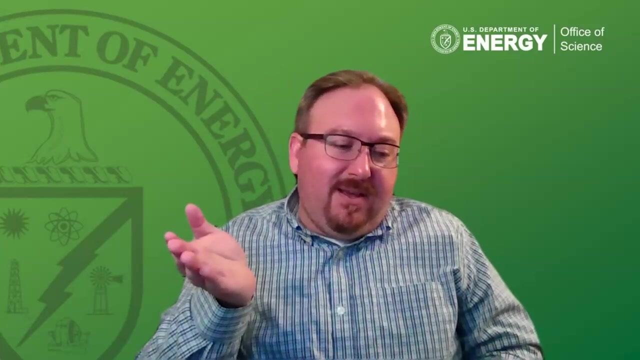 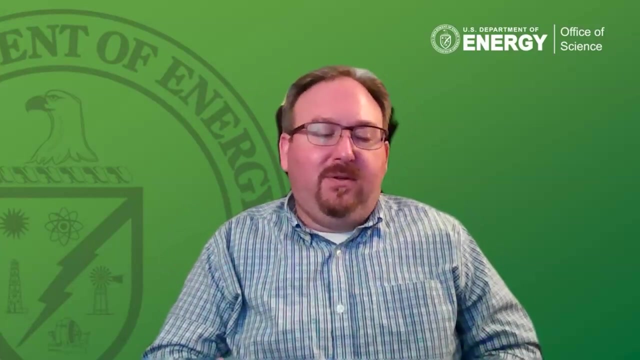 Is the NIDC product catalog considered an acceptable source of radioisotopes? I suppose I need a little more clarification. an acceptable source? So the NIDC is the business arm of the DOE isotope program. right, It's a virtual store front for isotopic sales. 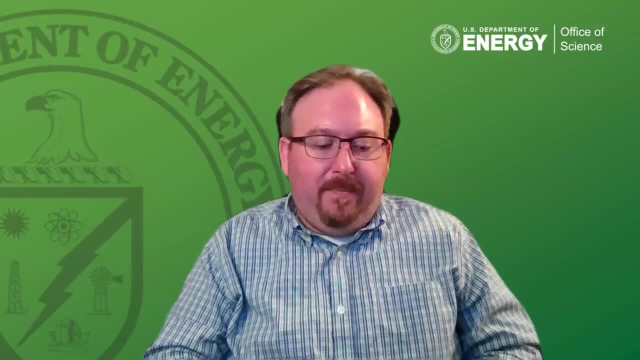 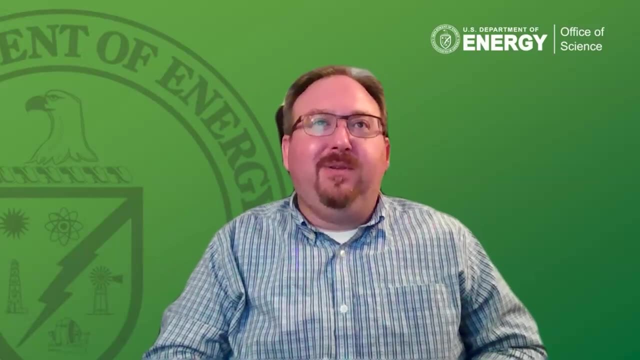 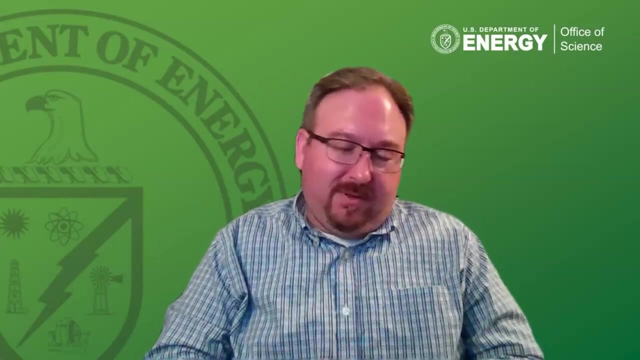 of products developed by the isotope program. Is it an acceptable source? Absolutely, In some cases it is, But I don't think it's an acceptable source. In some cases it's the only source I would, and this is a good point. this is a good time to bring this up. I would highly recommend. 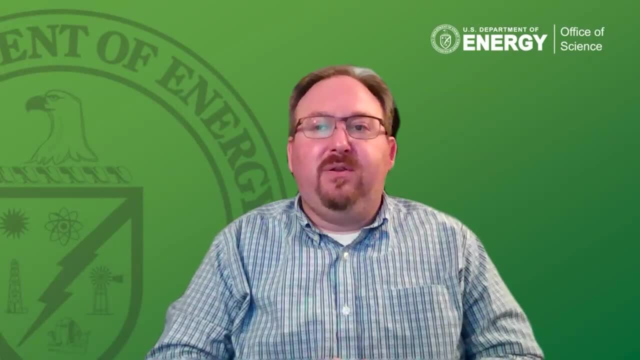 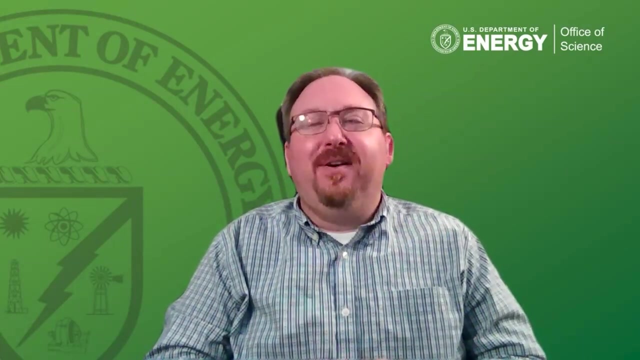 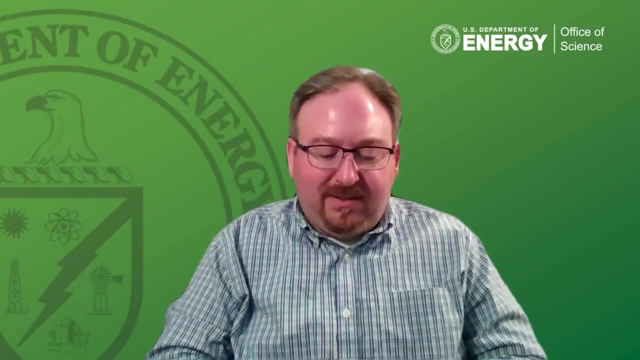 that if you're going to apply to this particular solicitation that you include? oops, it looks like I've lost my moderator. That's okay, We'll roll with the punches. I highly encourage anyone who is going to make application to this particular solicitation to obtain a quote. 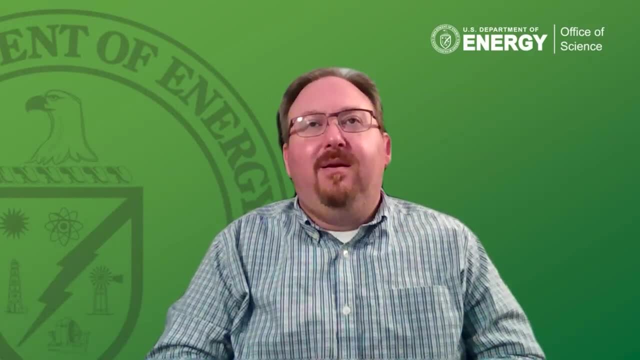 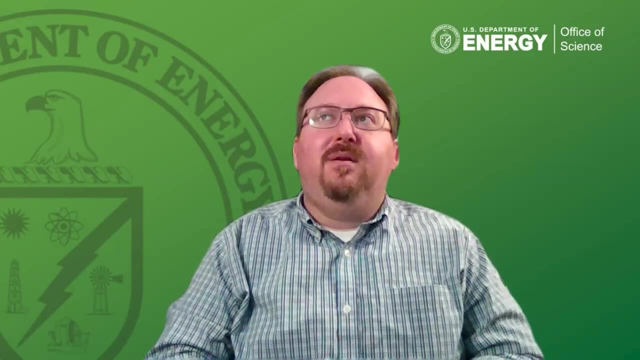 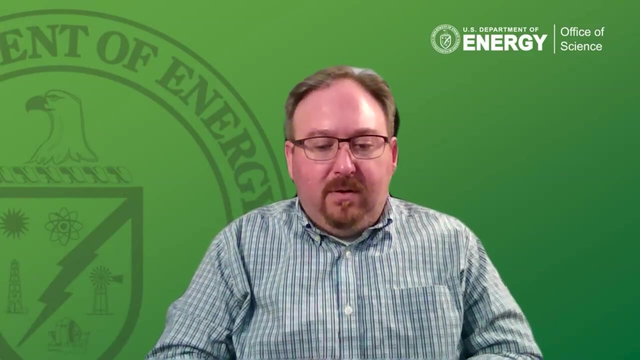 for the cost of any starting material they might need for several reasons, But not the least of which is work funded by the DOE. isotope program Typically receives Joann Se� PhD, the isotope Тамanna. It's that protein, Estáonder monomer. This is the fluoride tamanna. These home타pe tonic. sanktoásch, because it does contain products, is slightly out of balance with other platforms of the ISO". 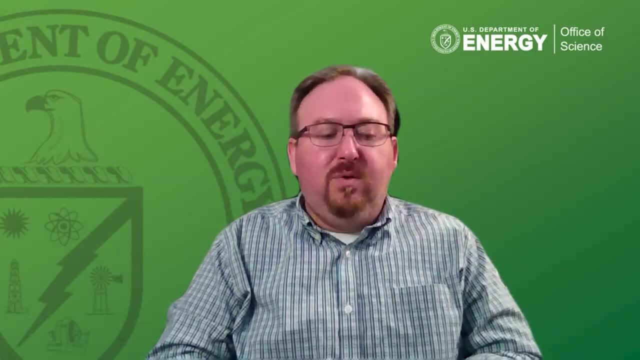 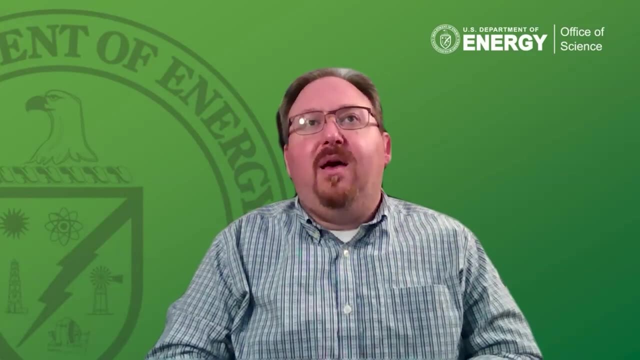 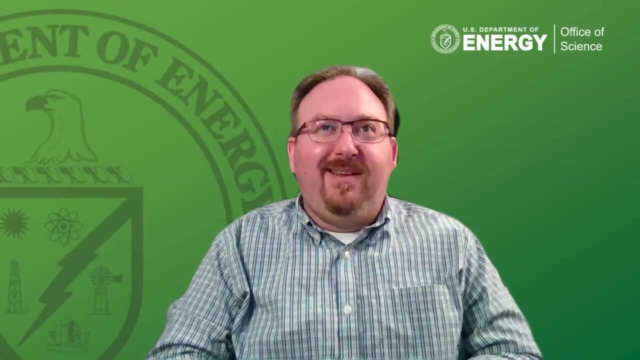 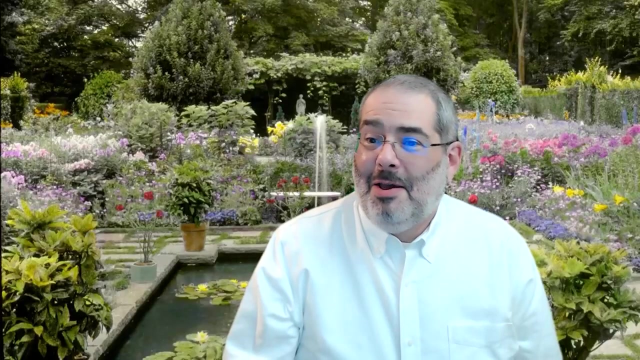 the isotope that they need to do the work that they are funded to do, at no cost from the program. So if it's in your budget I can then strip that portion out, But if you don't include the cost of the material I can't add it in. You also have another question, Ethan, that the NIDC. 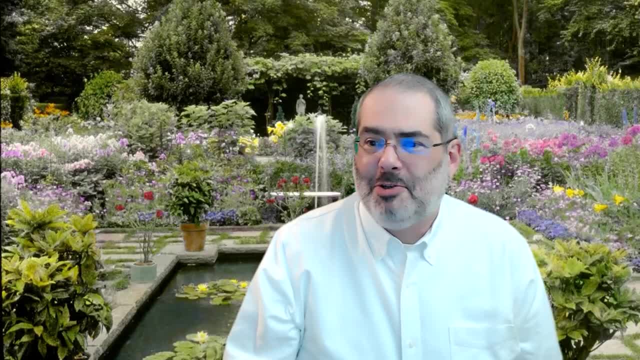 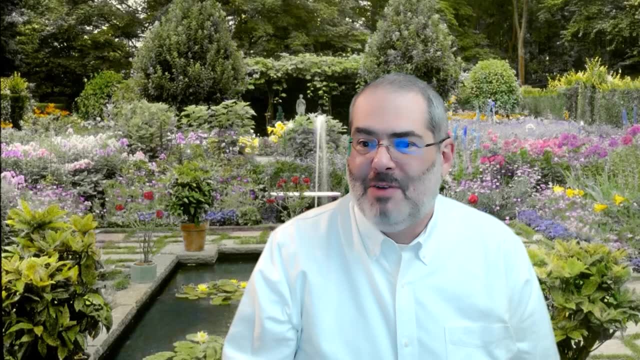 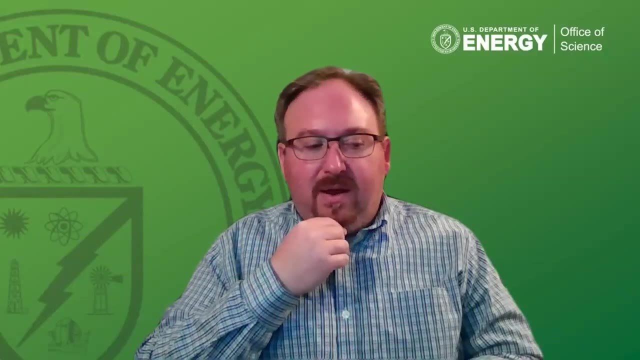 announcements recently have indicated greater availability of many isotopes, As an example bromine 77 and bromine 76. Are isotopes such as these of little interest for this FOA due to their stated availability? If something is already available, then seeking production in it. 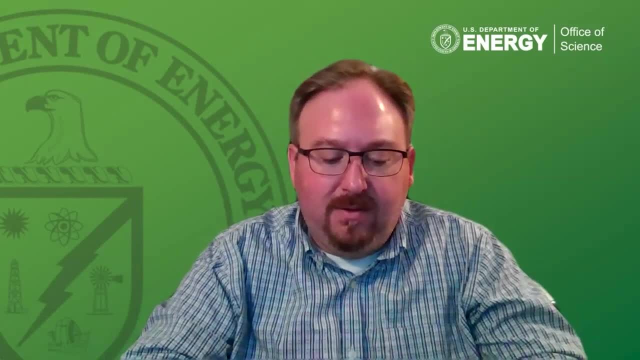 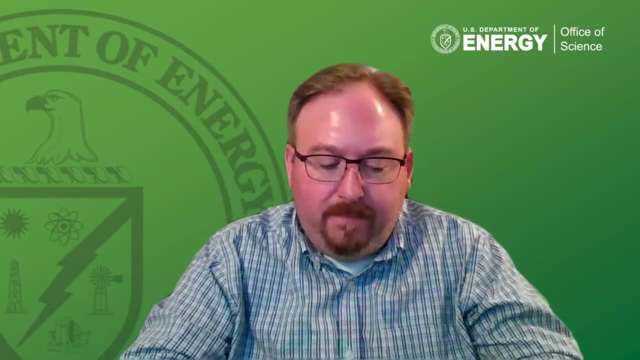 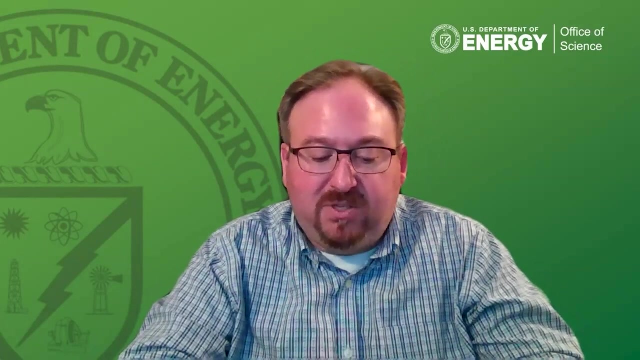 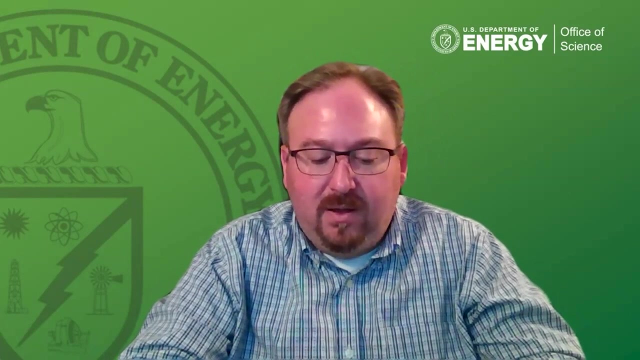 might find lower programmatic relevance. You know, that's as much as I can say about it. Unless you can identify something that is substantially going to increase yield and or purity over what the existing capabilities are, then you know it's been funded, It's in the catalog. There's no reason for us to really look. 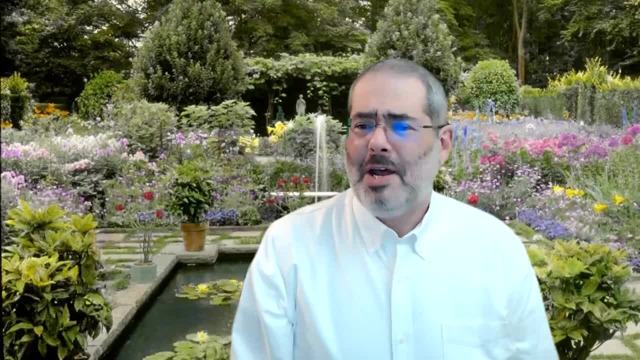 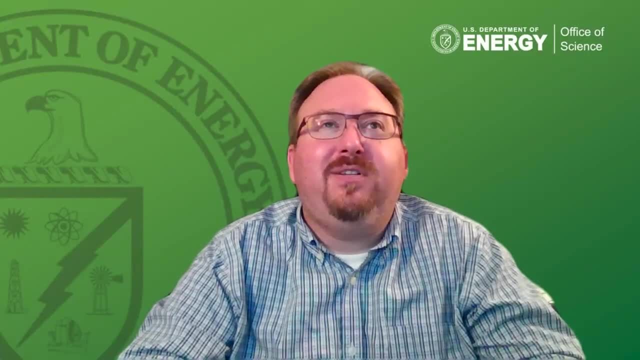 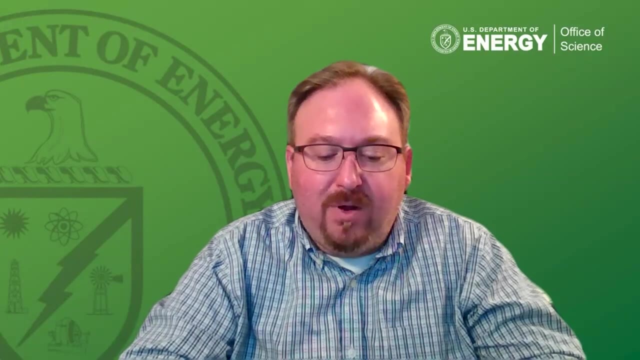 at it again: Is any preliminary data required in a proposal? Always a good idea. It's a good idea to anticipate the questions that the reviewers will have, But I can't say that there is any requirement for any data. You have to make a compelling. 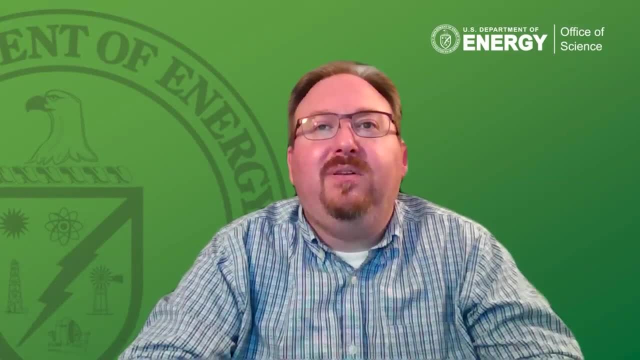 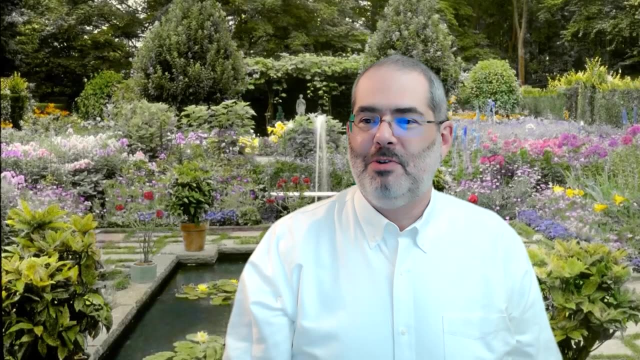 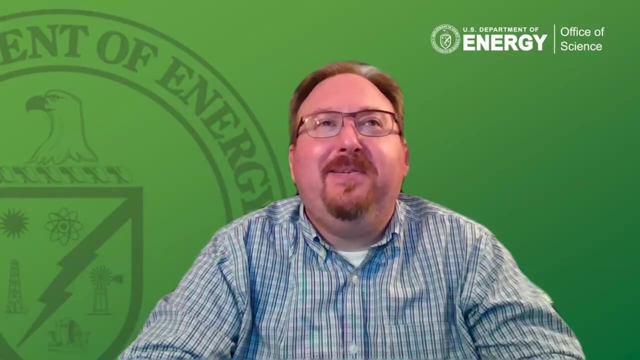 scientific argument. How you construct that argument is up to you. This programmatic relevance statement should be in future FOAs. The field would find this very helpful to understand what is most compelling for funding. We completely agree. Hence its appearance here. Thank you for the feedback. 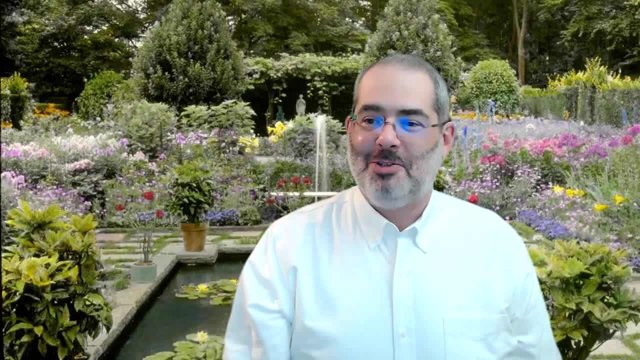 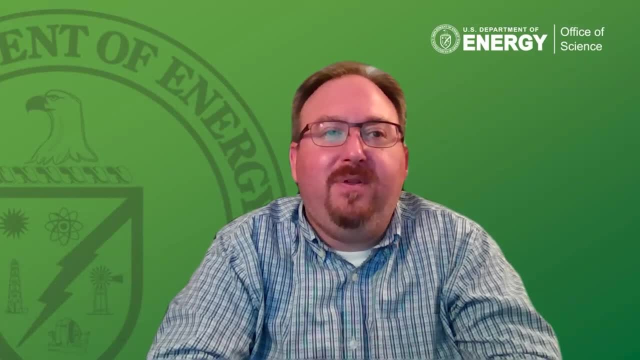 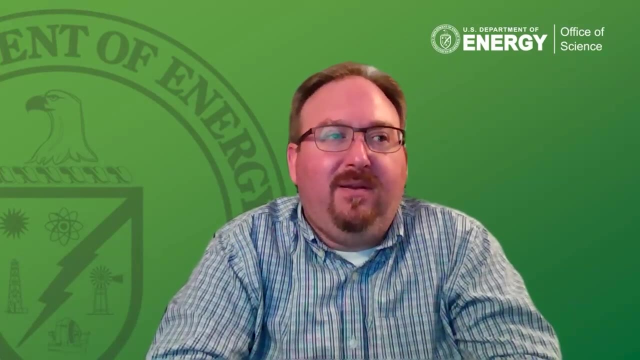 Is the area of nuclear nanotechnologies an acceptable area of research, As long as it is responsive to one of the topics that appear, one of those five or six bullets? then, yes, you know, independent of the bin that you choose to put yourself into. 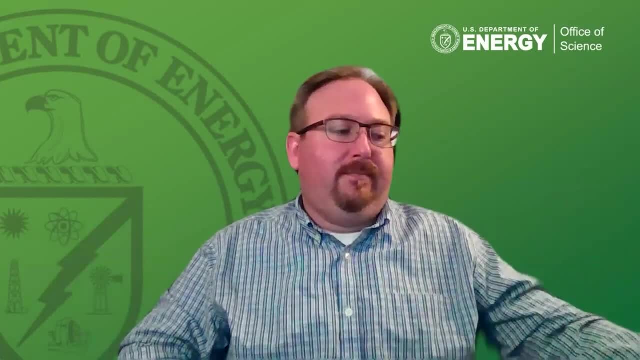 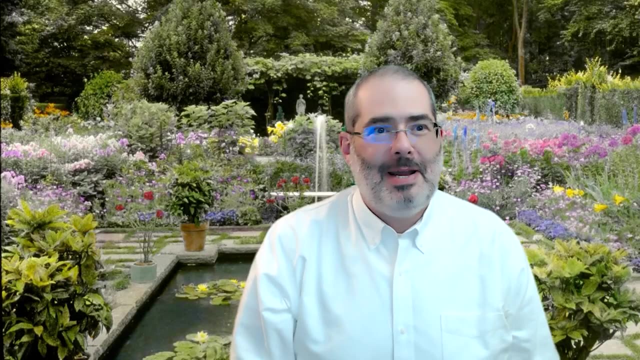 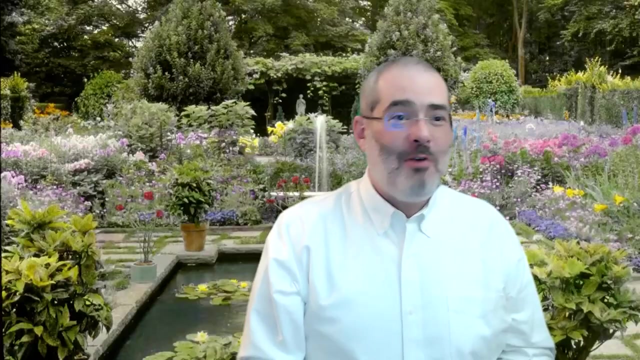 you just have to be responsive to one of those bullets. Will software licenses be treated similar to material LGTB procurement from a budgetary point of view? And let me know if you need me to take that one. Yes, please do. OK. Software licensing is an allowable cost when the software license is reasonably 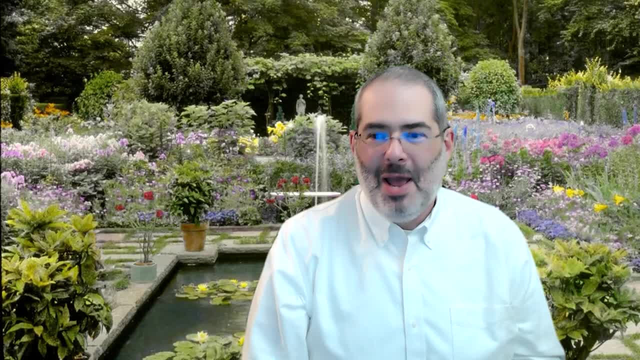 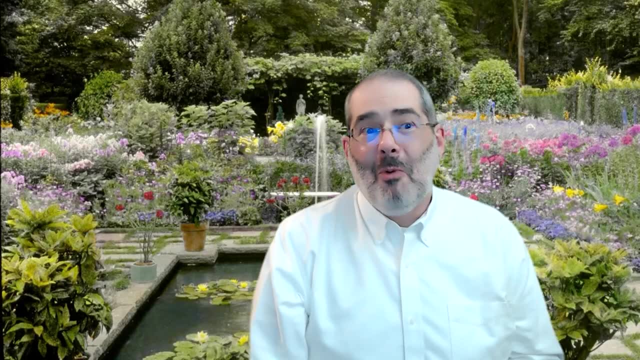 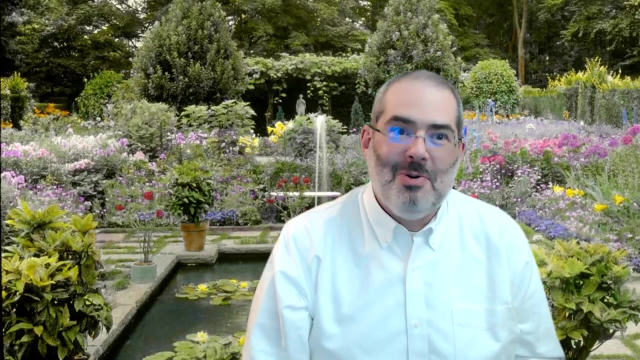 necessary to perform the appropriate scope of work. However, we would caution that licenses for general purpose software are more likely to be covered through your institution's indirect cost pool rather than as direct costs to any particular award. That said, propose the costs you need to accomplish the work you propose. Love it, Thank you. 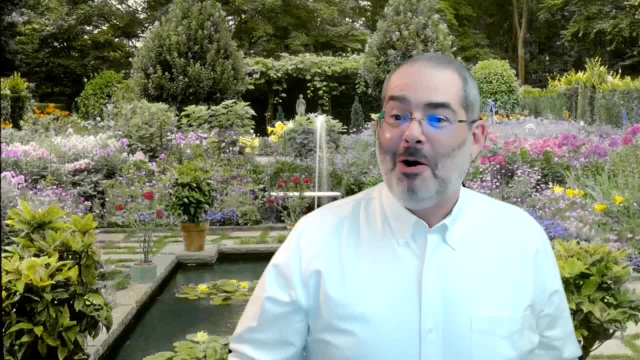 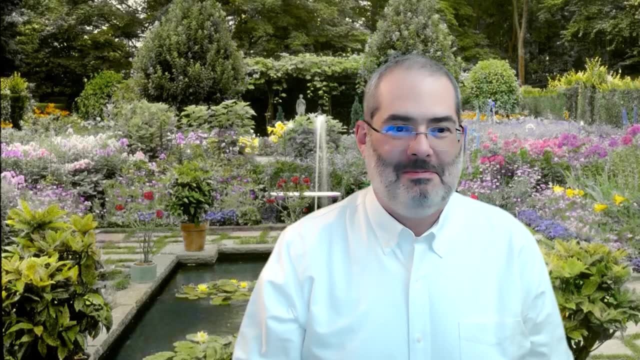 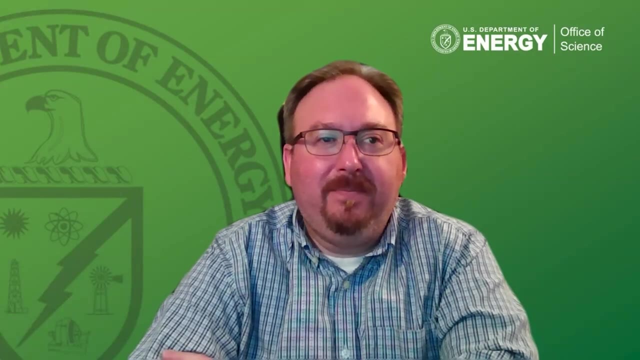 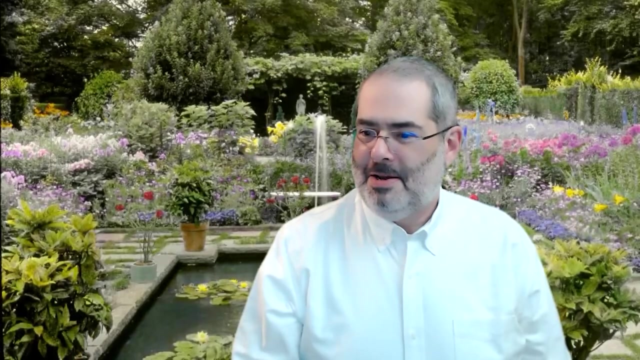 Pleasure. Does this FOA also cover separation of silicon-28 from silicon-29 for quantum computing? I would encourage reaching out to me to establish an offline conversation, please, And right now the questions seem to have slowed down. That's okay. 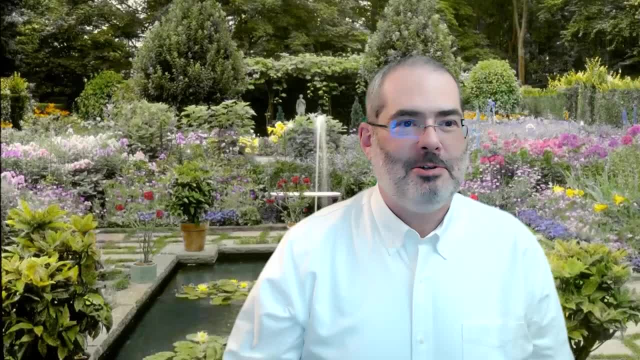 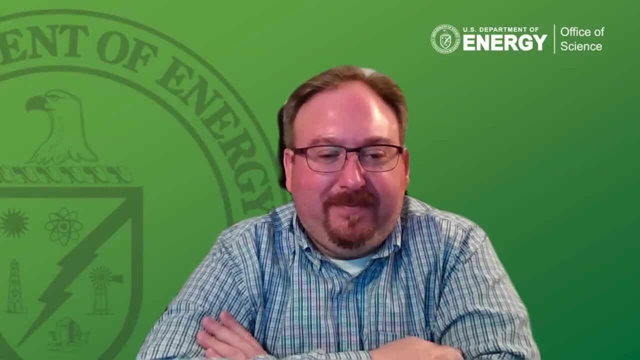 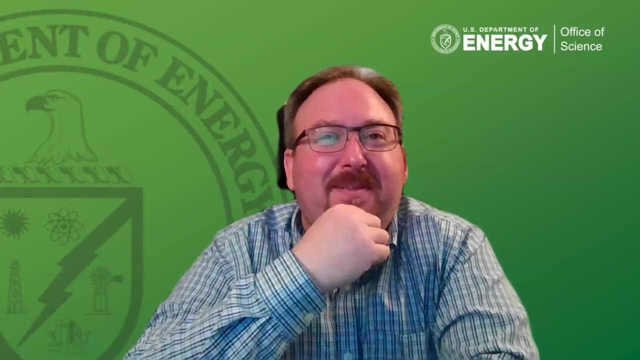 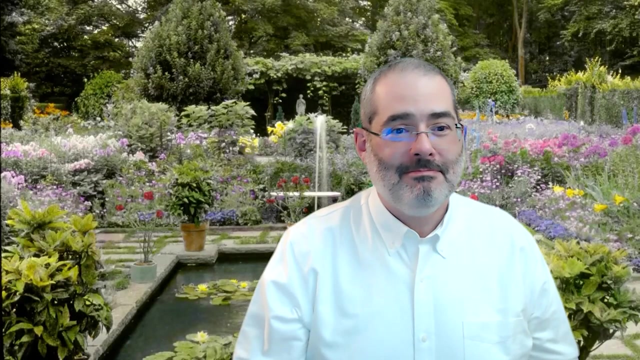 I have complete confidence in your research community. They will come up with more questions. Oh, I'm sure. There we go. Indeed, we have agreement. All right, My apologies, I'm probably over-caffeinated for this webinar. So, for those that don't know, the distinguished gentleman who is 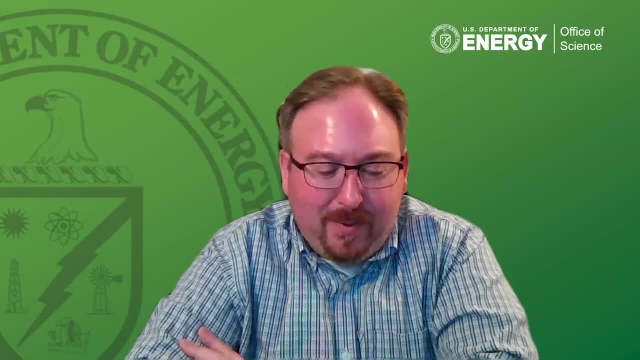 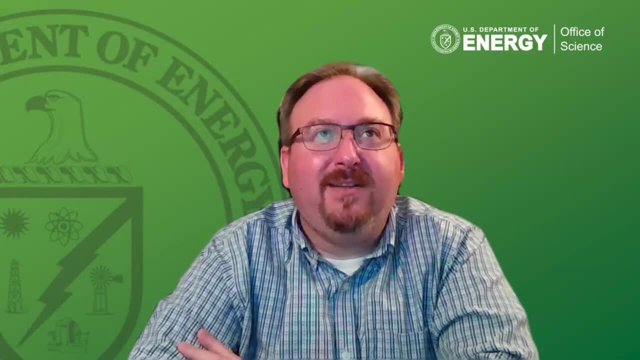 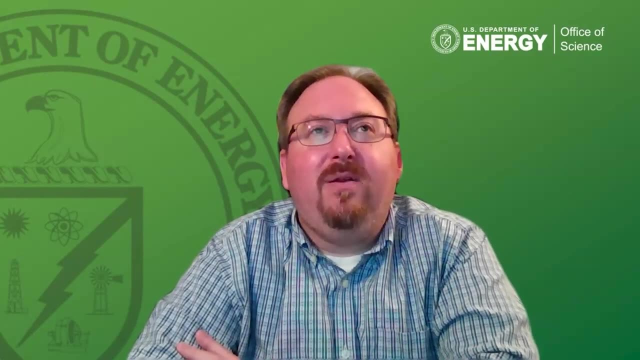 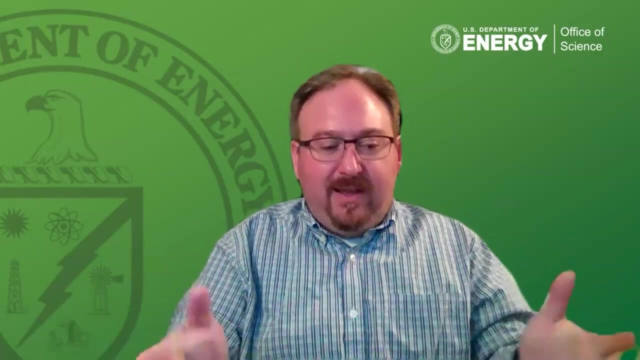 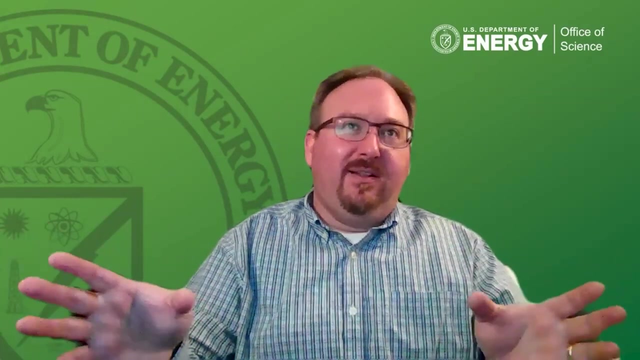 Mike is the office director for Office of Science, Grants and Contracts And within at least the headquarters building, he's the one who both facilitates the announcement that goes out that you all see the FOA, as well as make sure that the package we send up to Consolidated Service Centers in Chicago is in appropriate order. 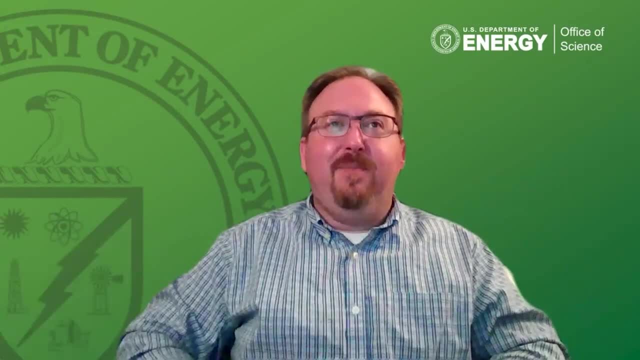 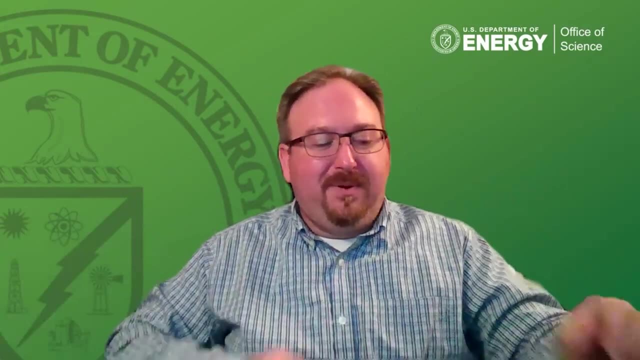 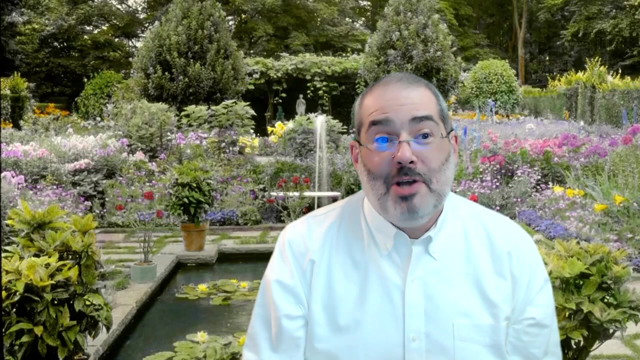 and make sure things keep marching along. So he is a wealth of knowledge that we all depend upon. The good news is that after 20 years of research administration, I have neither lost a program officer nor a researcher. Nor do we intend to. 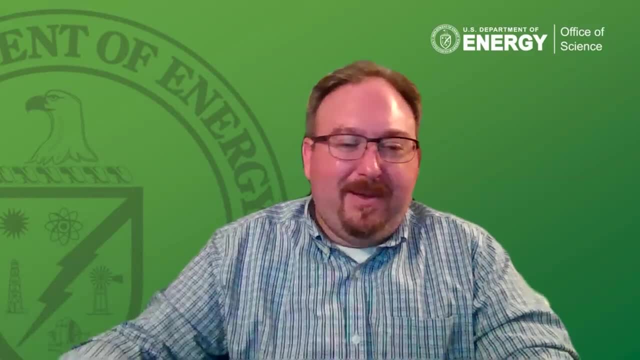 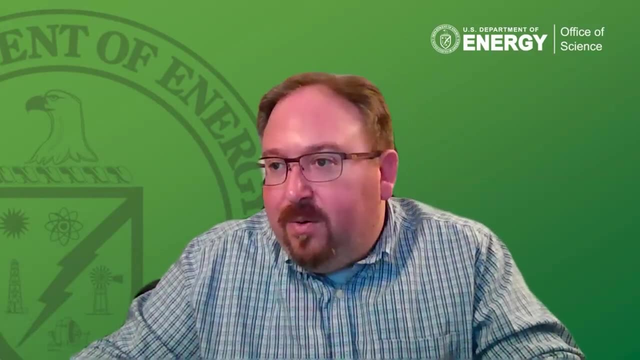 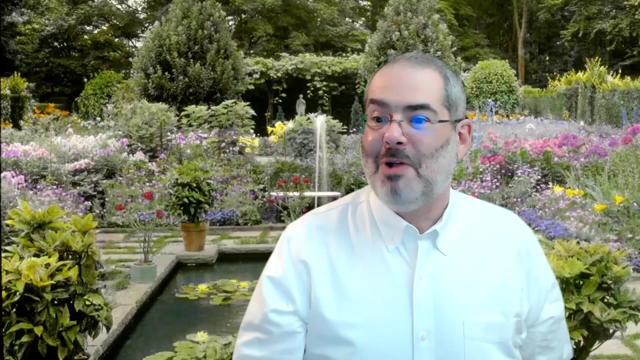 So I'm going to give you a little bit of time to start Here here, All right. Well it is. Oh, there we go. Okay, Can you please re-explain the OR clause for the priority topics? Will scoring be adjusted for priority topics? 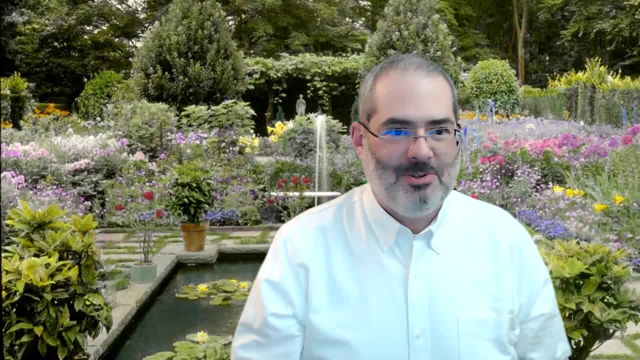 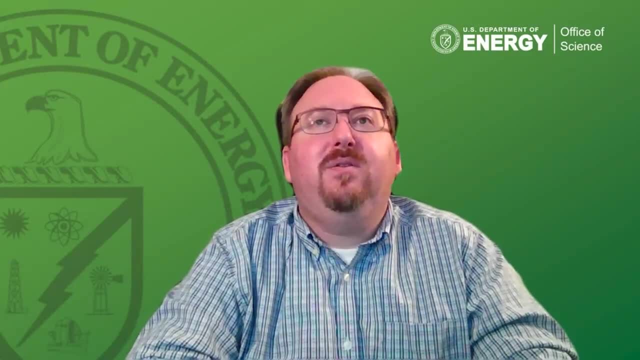 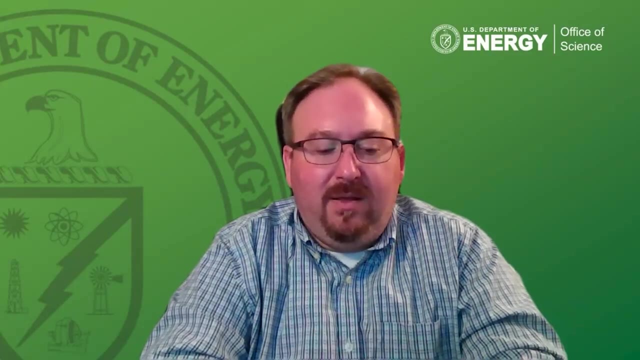 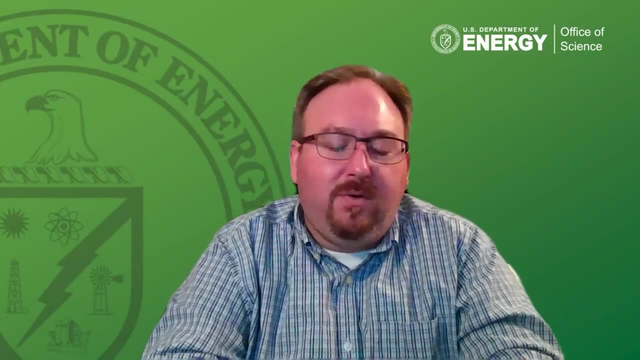 Does that mean you need to explain scoring and review matrices? So I would encourage everyone to take a look at the list of what are called program policy factors that are contained in the section on the review. In there, just read the. you can just read the paragraph related to the explanation of what program policy factors are. 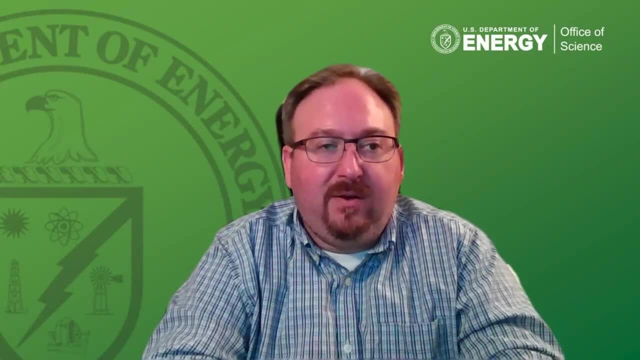 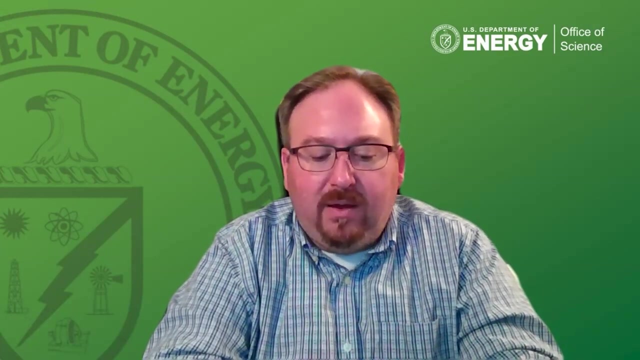 And then you'll see the laundry list of the program policy factors, Some or all of which might be applied, And I think that will answer your question. The OR clause stipulates that we recognize that those are the highest priority items to the program right now. 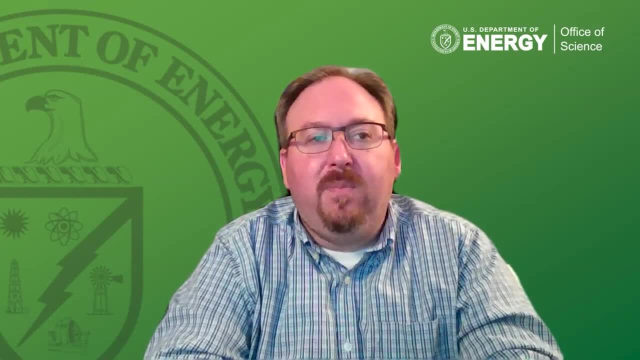 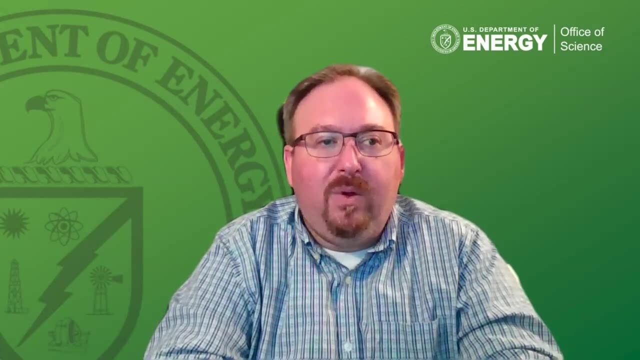 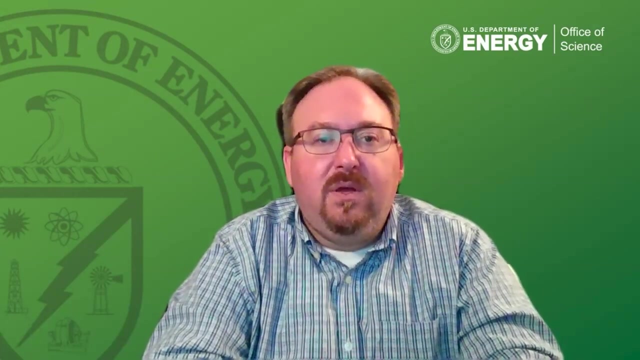 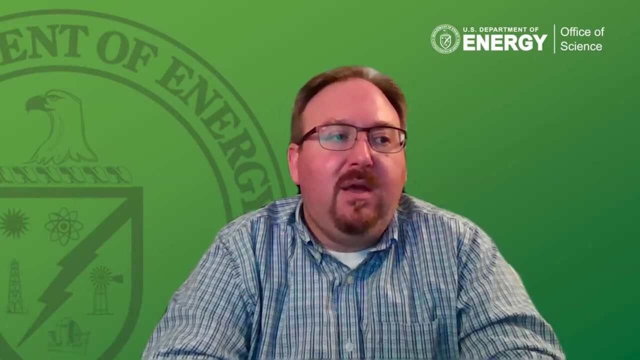 But there might be something that someone's mind develops which would be compelling to the program And we did not want to just have a slammed door seeking responses to just those six, those six bullets. That said, the swim lanes are helpful. It shows the community what we believe is the highest priority R&D and the direction that we're seeking this particular FOA to cover. 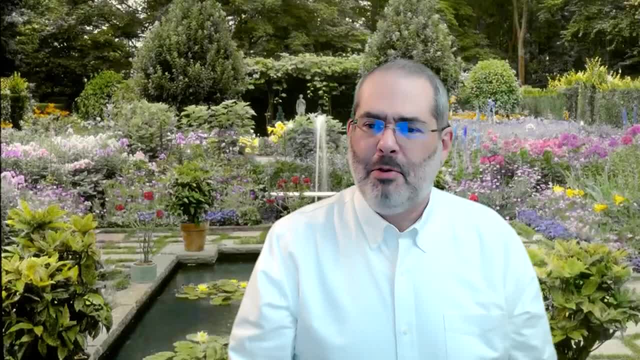 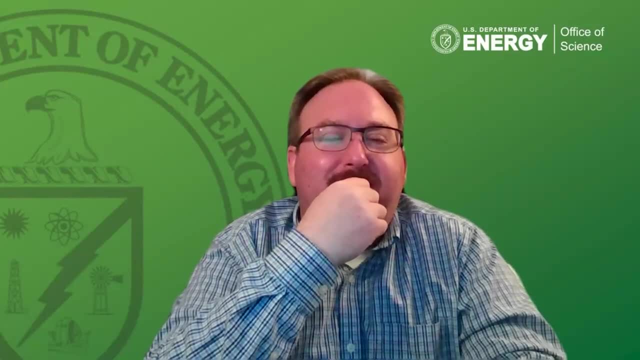 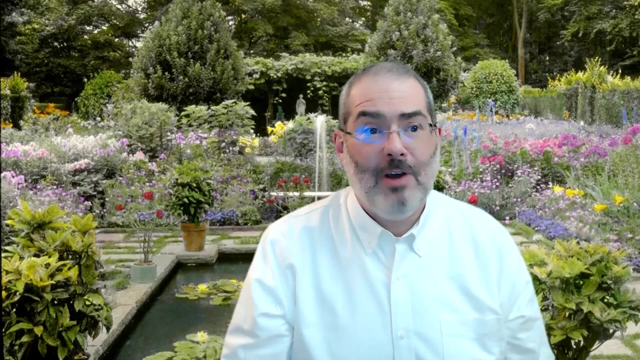 We have another question about where the recording of this webinar will be accessible, and the answer is it will be posted along with these slides from this webinar on both the isotopes microsite and the Office of Science Grants microsite. If you could find the slides, you will be able to find the recording, but please give us about a week or so for the automated transcription. 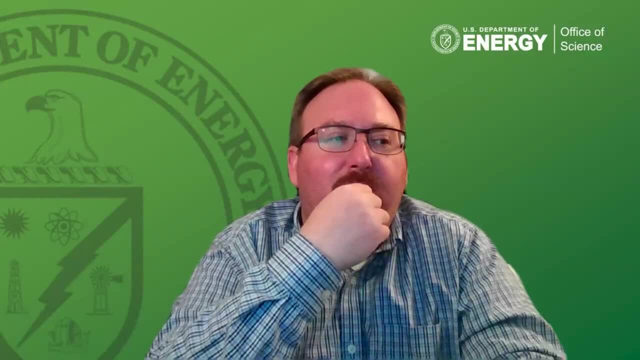 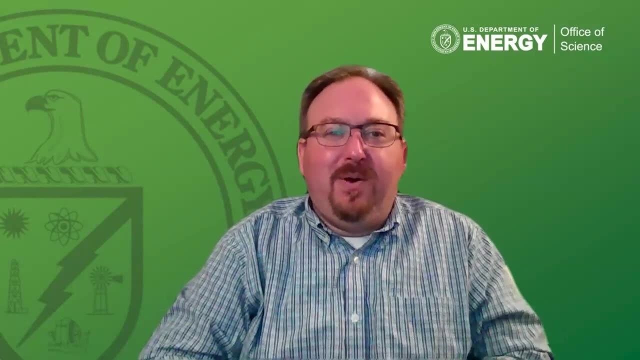 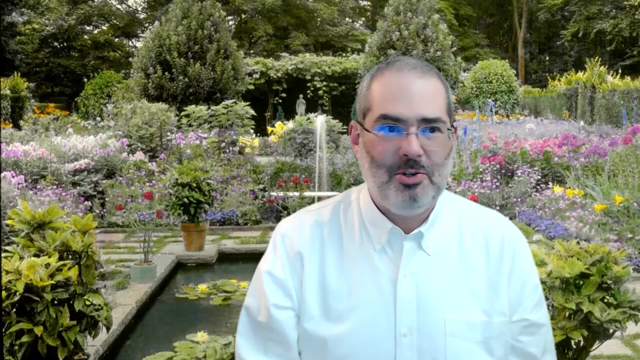 Yep, Where are you? Where are you? Okay, Where are you? Where you were able to find the actual solicitation is where you will find the slides and the recording. All right, We have a question about elaborating on the collaborative proposal submission route. And, if you don't mind, I'll try to take a first swing at that, Please do. Okay, The difference between collaborative proposals and prime and subs should be entirely driven by the nature of the relationship between collaborative proposals and prime and subs. The structure of a collaborative proposal is based on the relationship between the various institutions in the team. 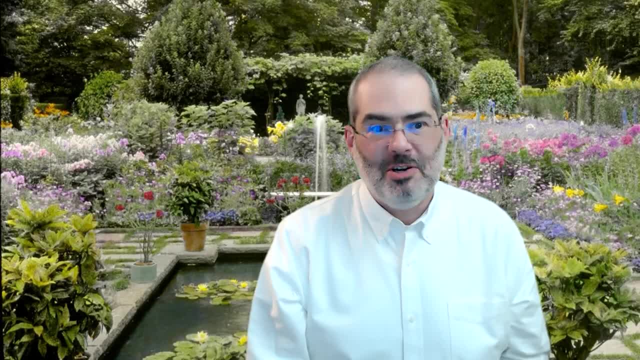 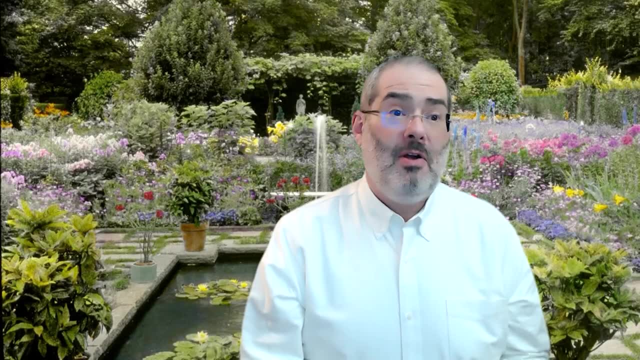 If someone is truly leading the effort and is more in a command and control position over the other team members, that describes a prime and subs model. If, however, it is more a network of peer level institutions working together for the same objective, that's more a collaborative proposal route. 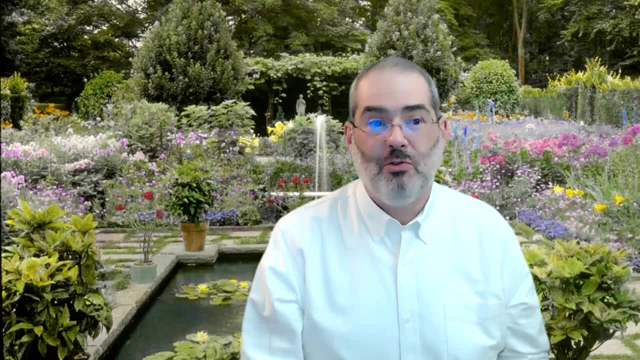 The other one is a collaborative proposal, rather, That's a collaborative proposal, collaborative proposal route In a prime and subs model. our objective is to make one award to the institution who will then manage, and therefore directly control the work at the subs In a 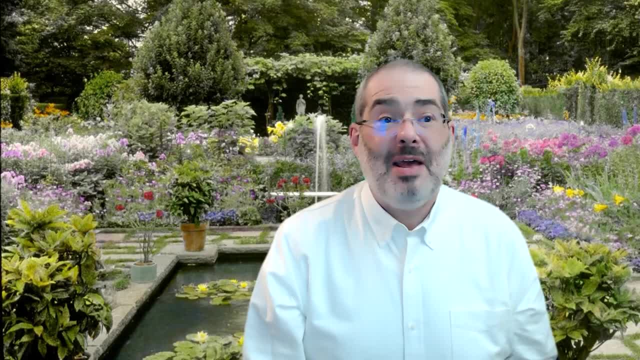 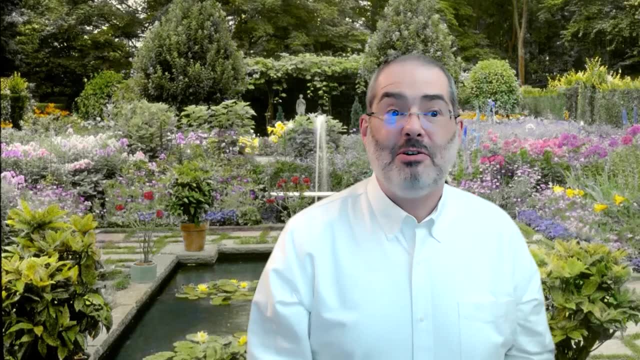 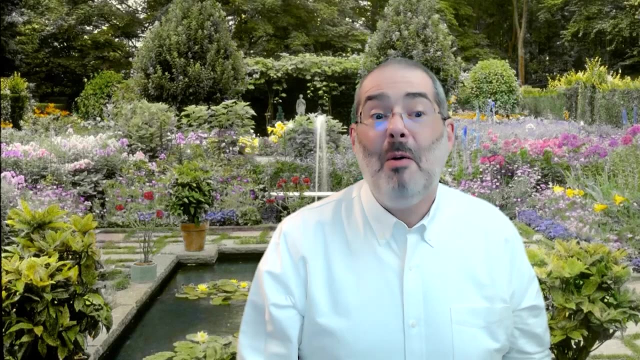 collaborative proposal process. our objective is to make multiple independent awards to each of the selected team members, who are then going to perform their own work, again presumably in the same direction, to advance the same objective. but no one institution is capable of telling other. institutions exactly what to do to reach that objective In a collaborative proposal process. it's therefore critically important that we receive exactly the same research narrative from each of the proposed teams members. Each institution needs to propose its own budget, describe any unique facilities or. 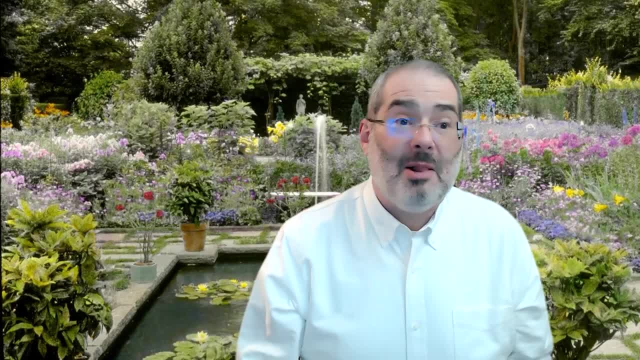 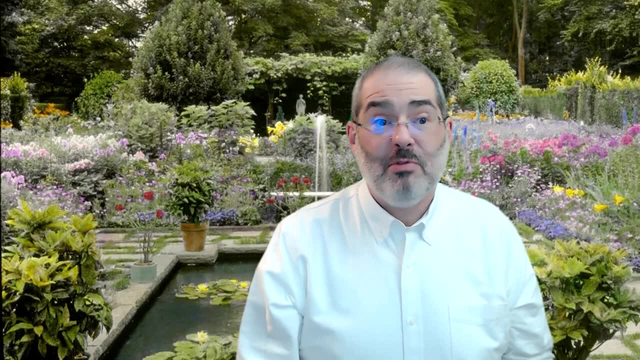 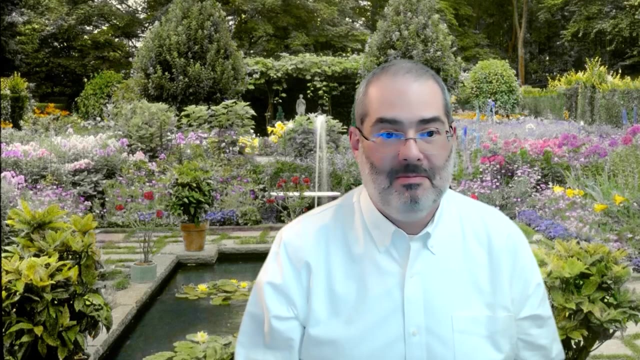 equipment and provide material about the personnel at that specific institution. But presumably, if you're working as a collaborative proposal, you need to have one common research narrative from every team member. Did I hit it for you? That's everything. yeah. Might be thinking that I've actually done this before. Historically many awards have gone to a small number of institutions. Is there a component to the review process that motivates new sites that have not been funded by DOE in the last decade or more? 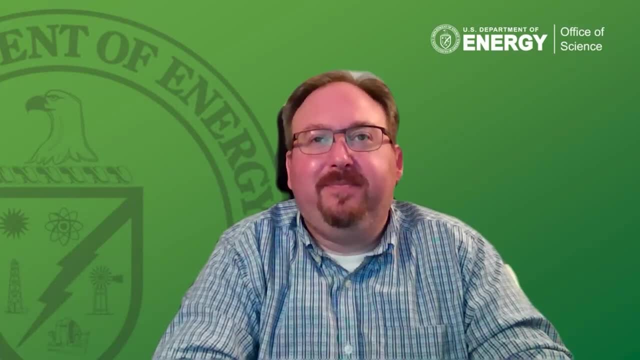 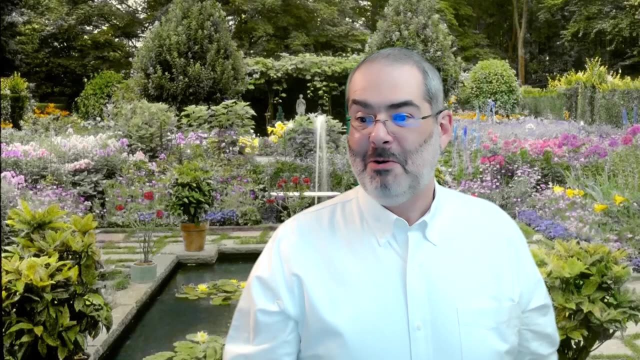 Absolutely. Take a look at the program policy factors. Will there be double-blind reviewing for this FOA? No, there will not be. Can proposals be anonymous to reviewers to provide non-biased reviews? No, there cannot be, because the comments. 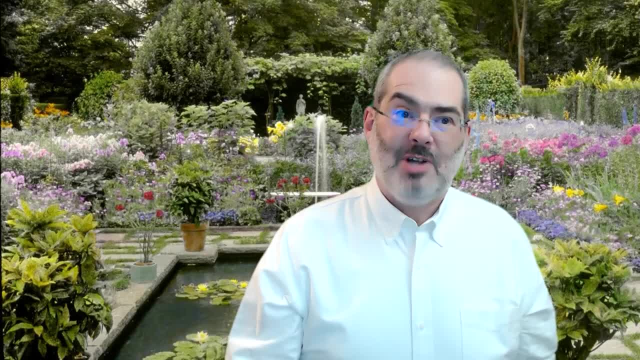 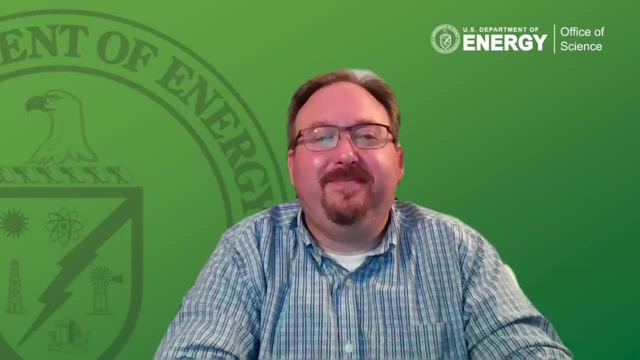 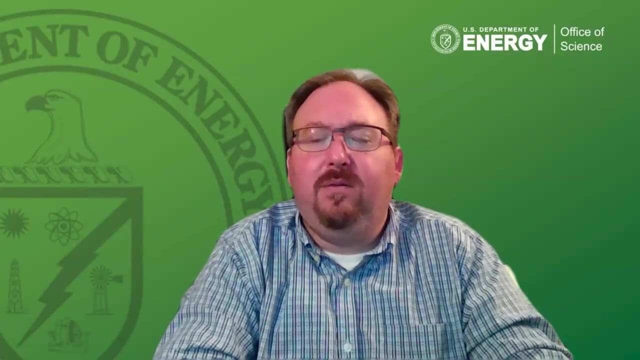 of the mocking personnel are an integral part of the Office of Science Review Policy as established by regulation. Sorry to steal your thunder on that We did. Can you share the reviewer metric's charge by which the reviewers score each proposal? So the well. 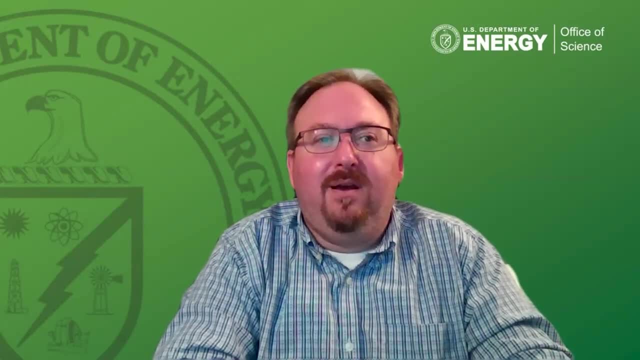 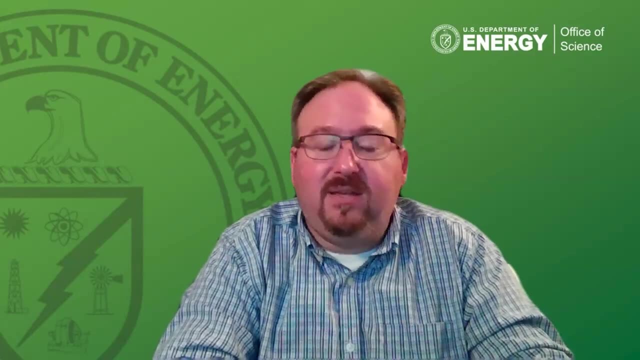 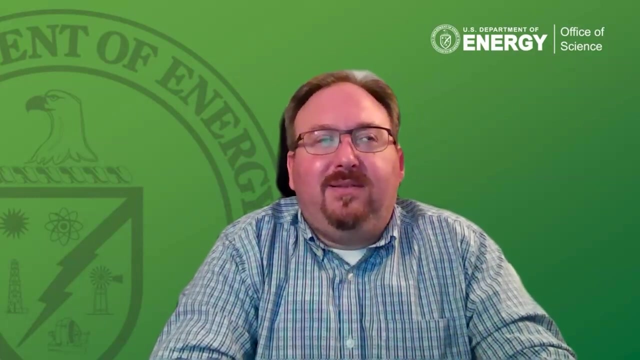 So the charge elements are listed And they were described in the, in the slide as well as in the FOA, So you can see exactly what the reviewers will be, will be reviewing based on You know. that's, that's, if you can address those metrics, if you can, if you can address those. 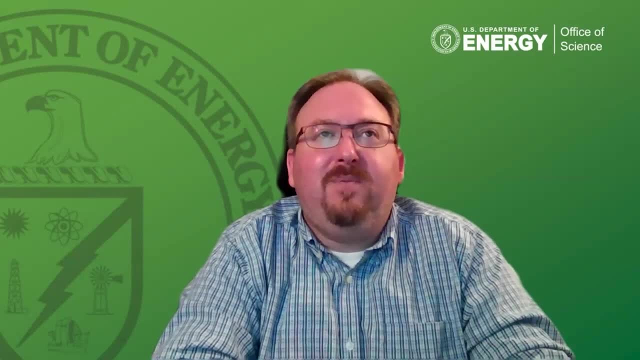 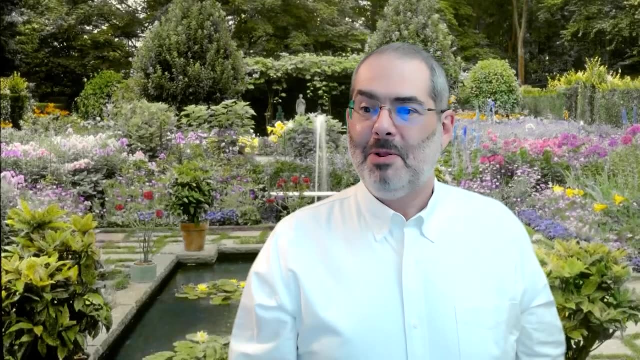 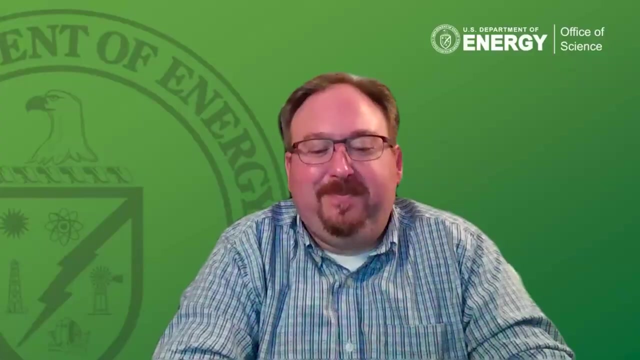 those charge elements, then you've set yourself up for the the highest possible score that you can potentially receive. Are there any stipulations regarding funding US citizen versus non-citizen students? Absolutely not. The only thing to be mindful of is that, if you are planning to perform, 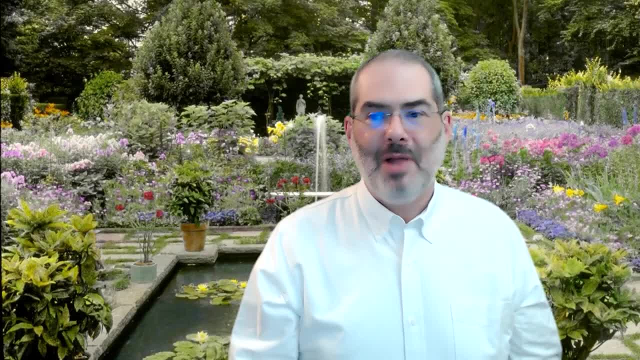 work at a DOE site or facility or national laboratory, non-US persons may have an additional screening process before they gain physical access to that site. However, that is physical access to a DOE site. that has no bearing to what you may do on campus. 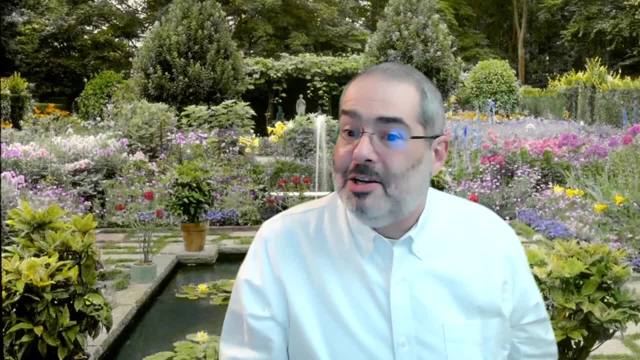 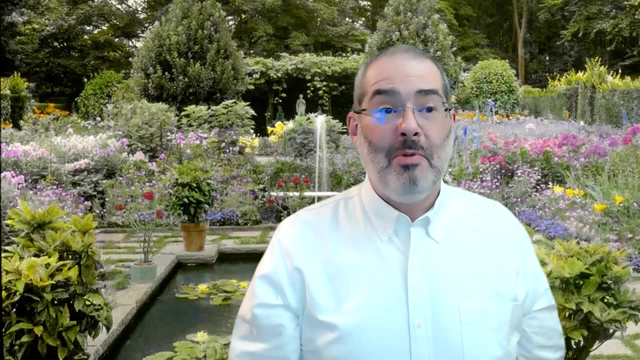 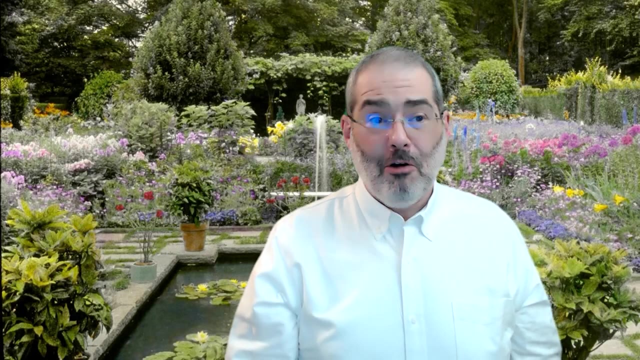 Is DOE enforcing the provision of a living wage to graduate students working on funded projects? No, The Department of Energy has no authority to impose or enforce a minimum wage. However, we may encourage- and we do encourage- all institutions to consider what flexibilities may exist within their internal policies and procedures to advance the objective of a living. wage for all students. If the submitted proposal to this FOA is similar to a previous submission to a different FOA from the DOE, would this impact the acceptance to fund any of the submitted proposals? Yes, We will not fund the same scope of work twice. 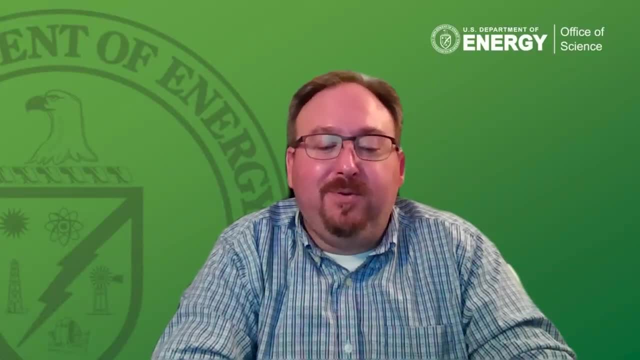 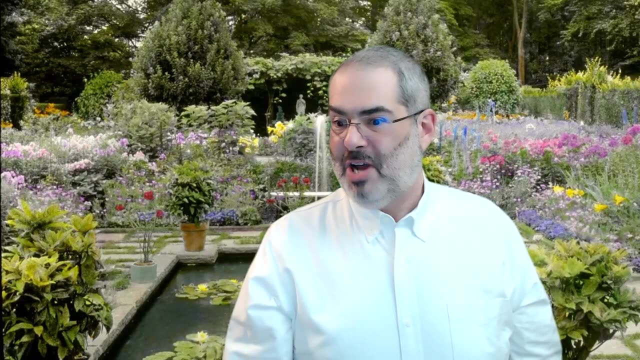 If it was declined, you're more than happy. you're more than able to resubmit. Given the difficulties, delays and change of staff associated with COVID-19,, would the DOE be able to fund any of the submitted proposals? Is it acceptable to submit proposals that expand upon and complete? 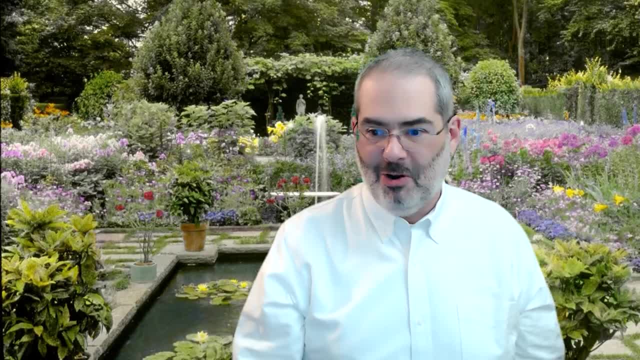 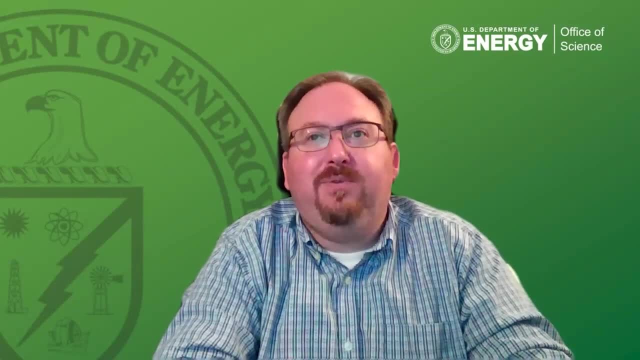 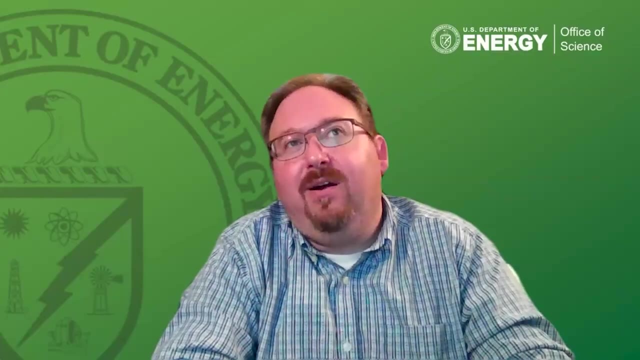 a previously funded scope using the same technology and lessons learned. Well, that would be an expansion of previously funded work on a terminated award. That's absolutely acceptable. Also known as the D part in R&D right, That's the development part You're. 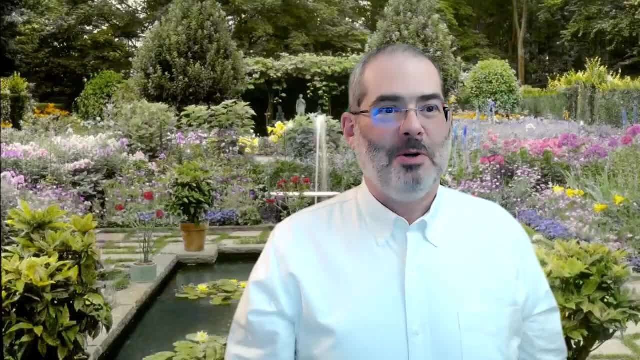 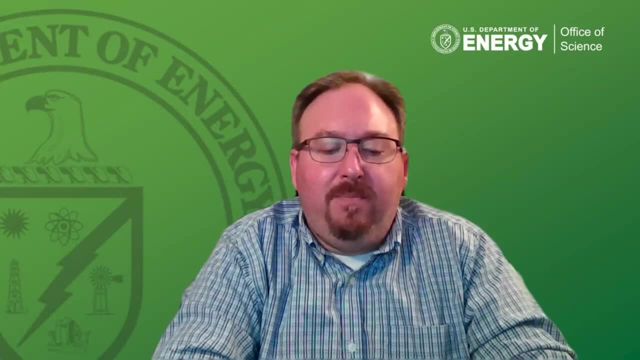 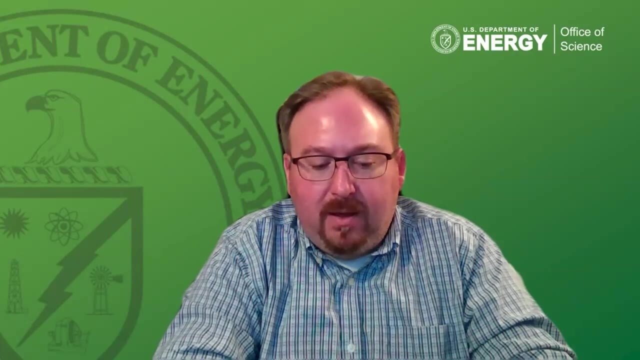 expanding. How are reviewers chosen? How are reviewers chosen? How are their board members chosen? The best way to do that is to refer to the DOE website and sign a request. Reviewers are chosen based on subject matter expertise. Peer review is an integral part of the proposal and funding activities of the Office of Science. 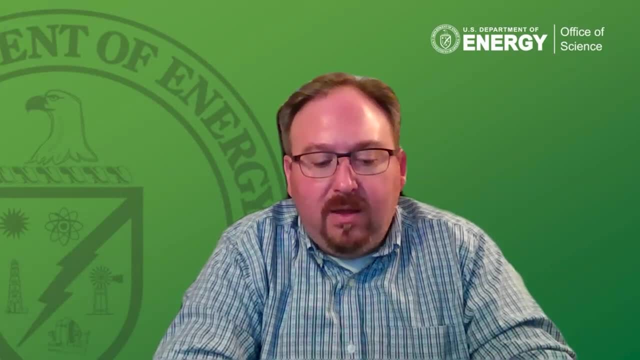 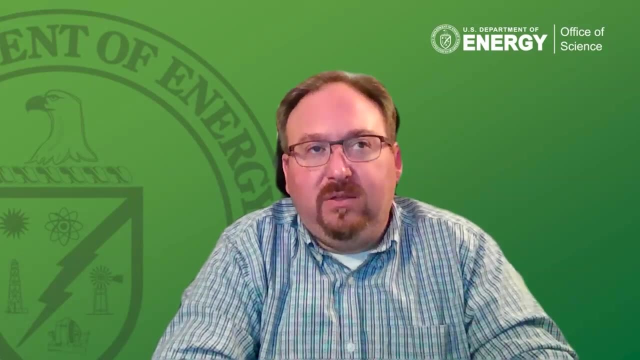 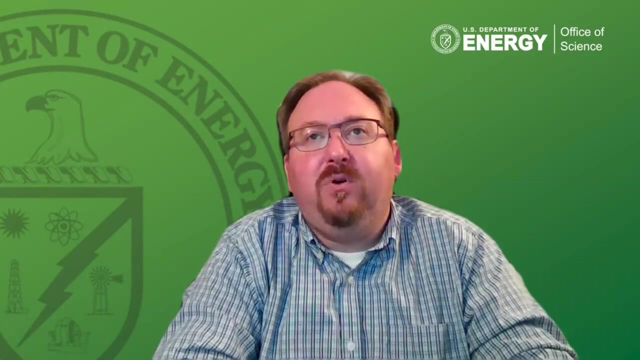 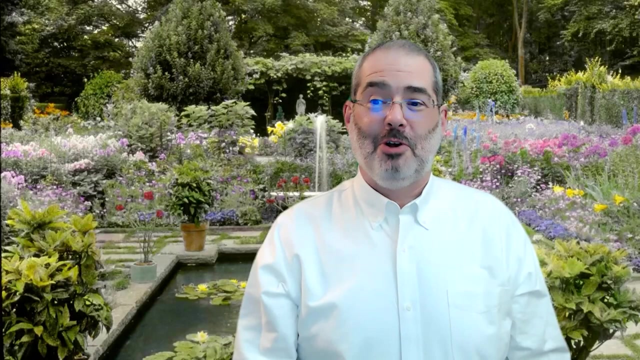 We guarantee a high-quality, unbiased review by subject matter experts, but I do not guarantee that the same review panel will be used year after year. That's just based on availability of personnel and the pool of proposals received. Can principal investigators also be reviewers? 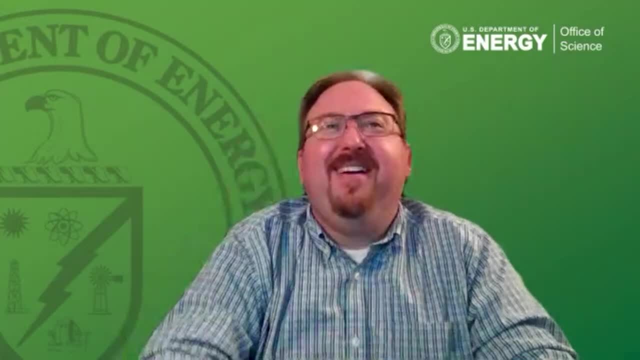 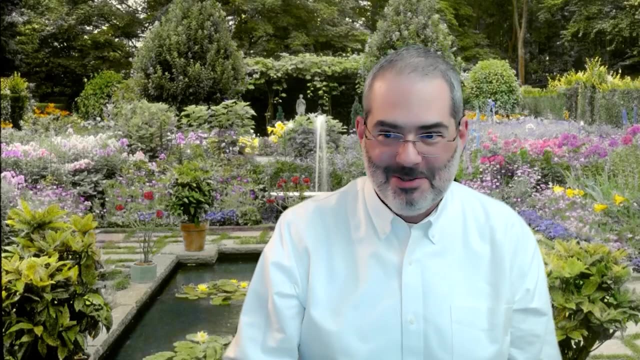 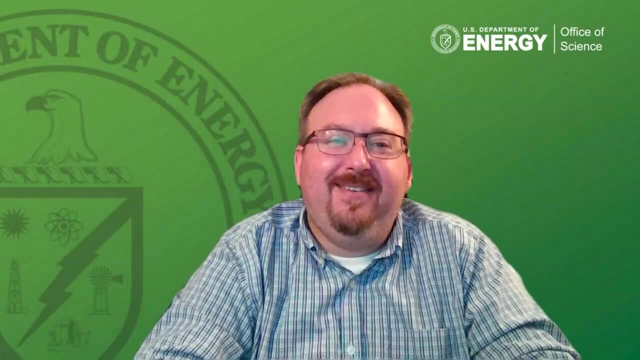 They can be reviewers On the same solicitation. There you go. Presumably, if you have proposed work under a solicitation, you are conflicted from evaluating your competitors. Yes, Oh, come on, We've got eight more minutes in the Ethan and Mike show. 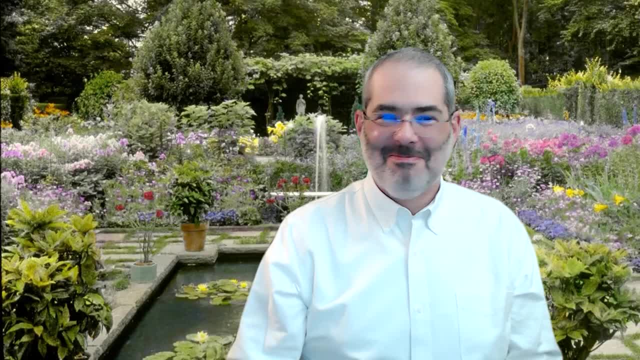 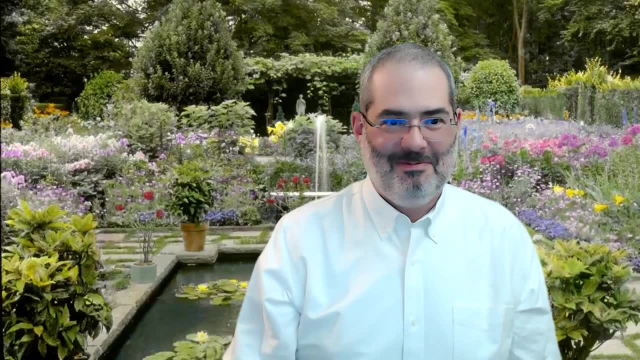 We need more questions. There's one: What are the top three isotopes that IP is in? What are the top three isotopes that IP can be in? What are the top three isotopes that IP can be in? I would direct you back to the bullet points. 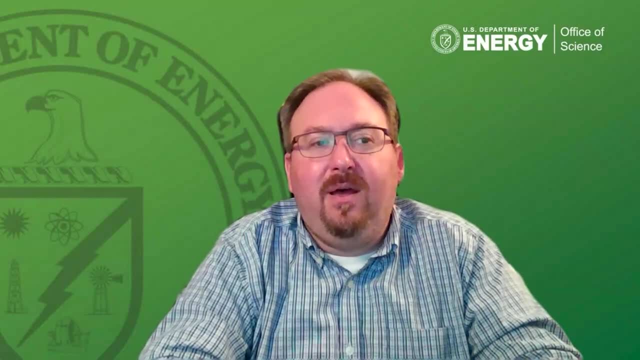 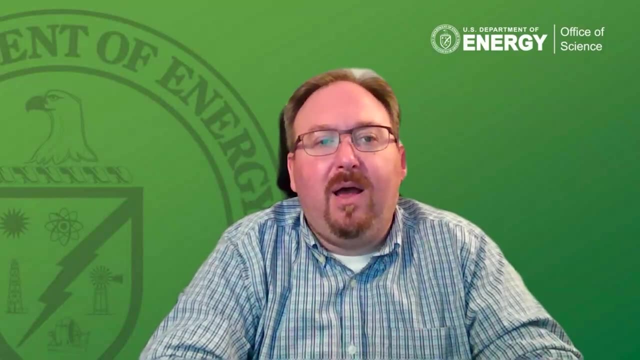 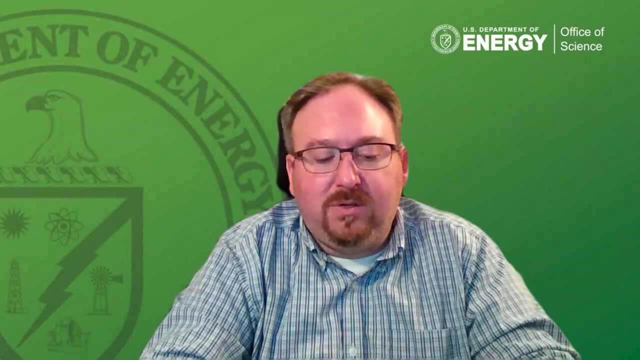 There's no way for me to say one, two, three. There are categories of things that we are interested in and rankings in each category, So I would look at the bullet points that are listed in terms of the high-priority research for the office. 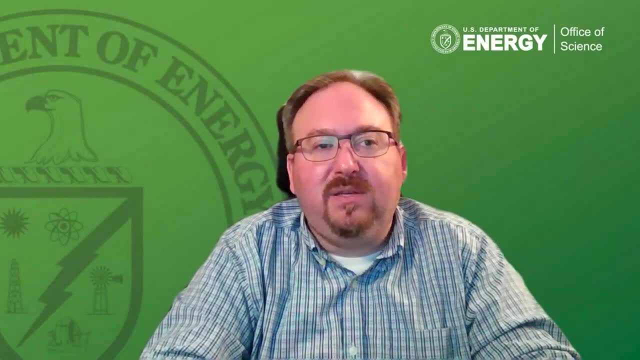 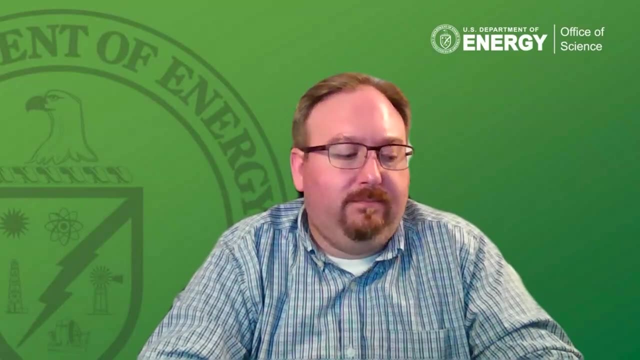 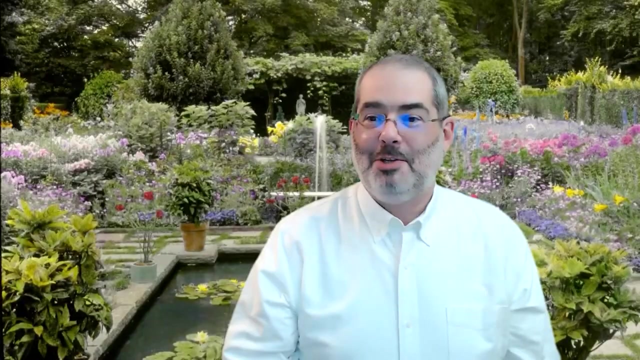 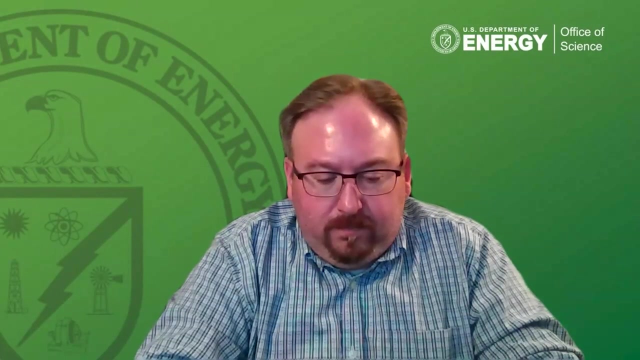 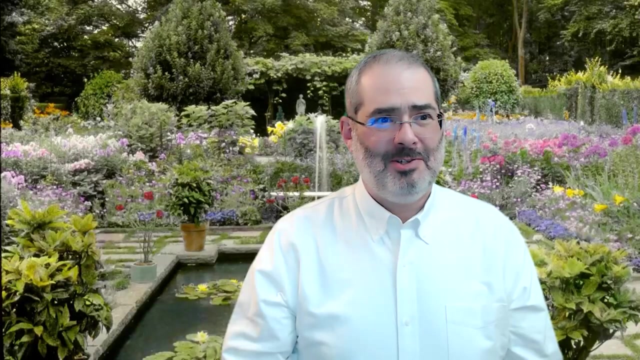 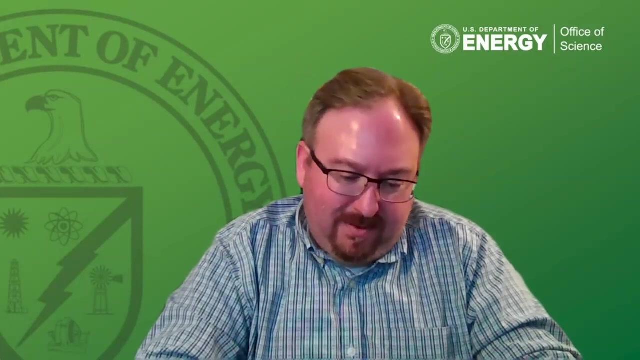 And if there are examples, examples listed, you can, you can take those as you will. Is research to advance existing techniques for isotope enrichment of interest? It feels like it's getting into the discovery science versus applied research. Well, there's, there's the. there are several components to this answer. 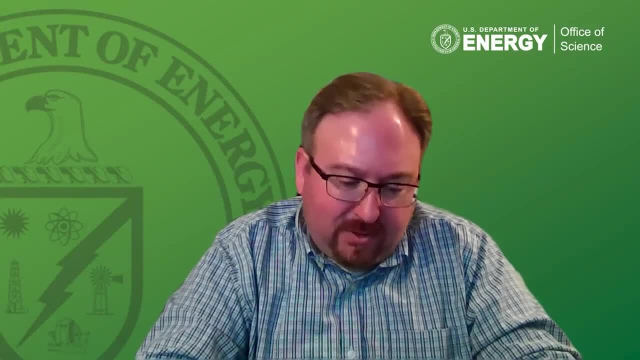 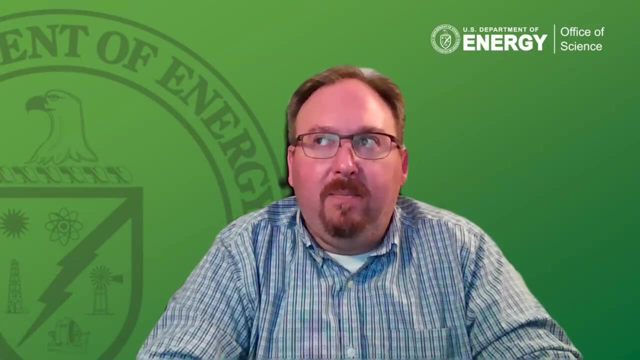 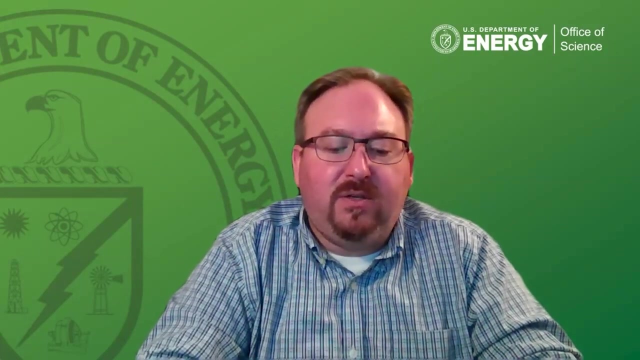 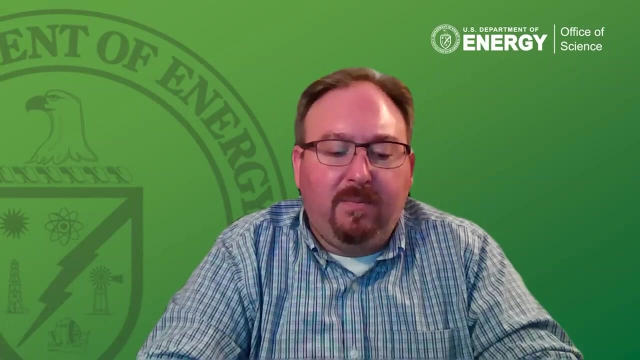 But the answer is that there are substantial investments being made in aspects of isotope enrichment by the isotope program. If you're intending to engage in that type of Rn D, then I would suggest you reach out to to me to request an offline meeting. 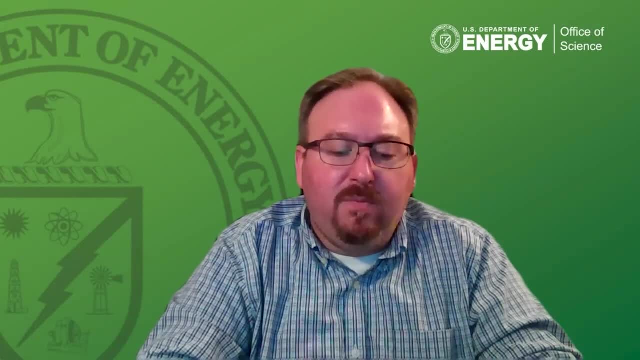 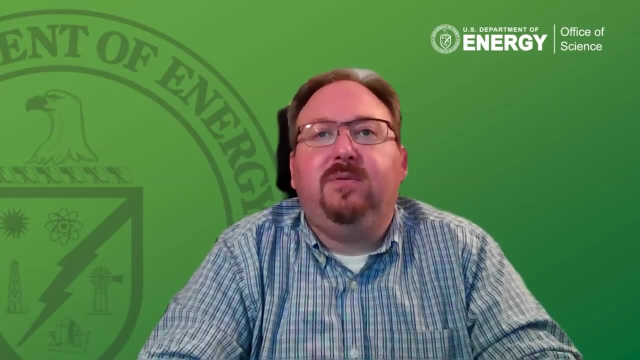 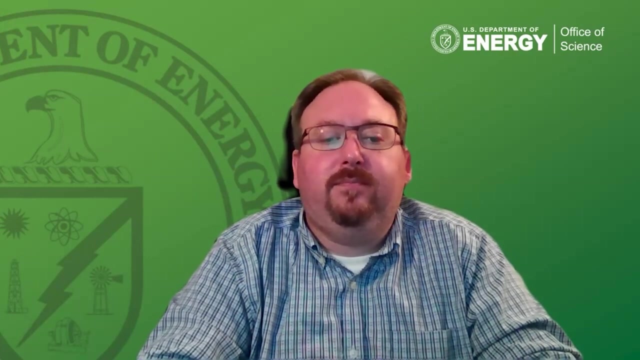 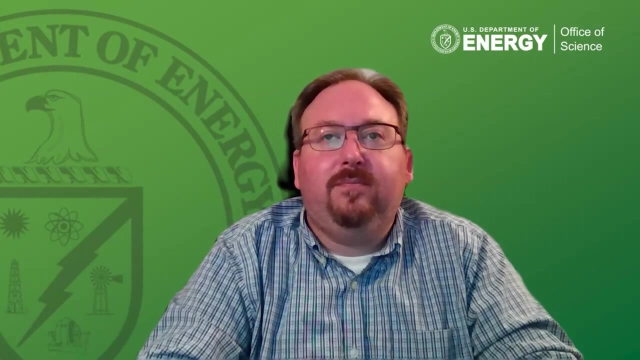 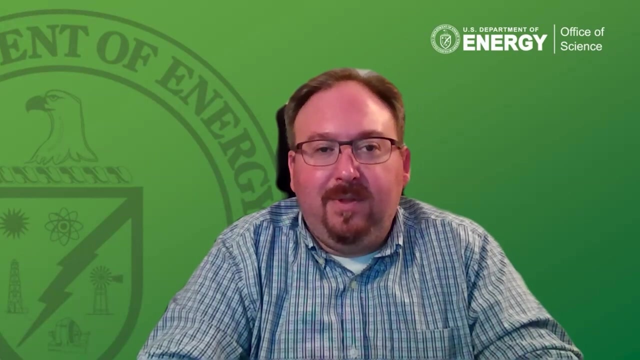 I want to make sure that, before you waste valuable time and resources developing an idea to maturation, that you're within the correct swim lane boundaries. If you have any questions, please feel free to reach out to me. Anybody else If not, you all know where to reach me and how to find me. 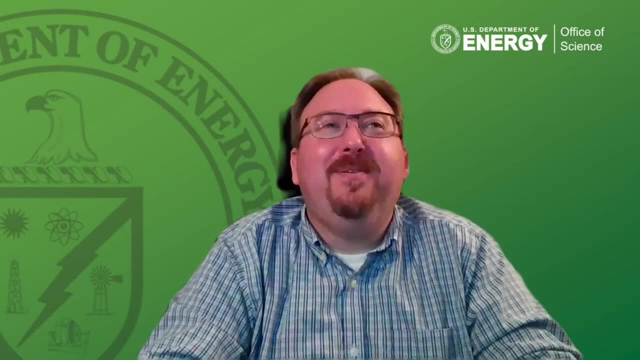 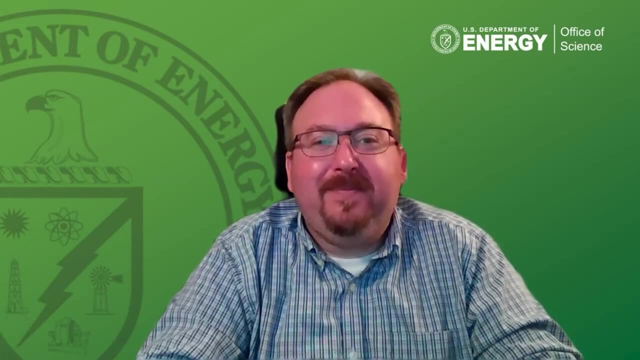 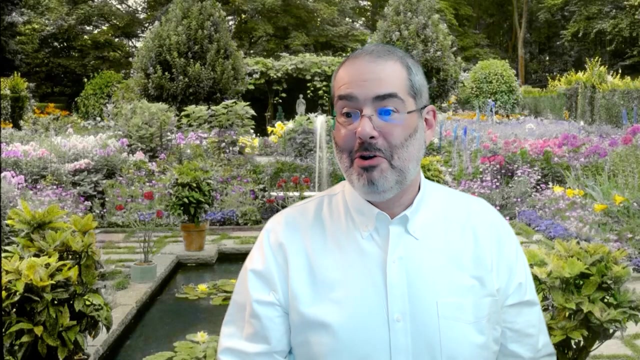 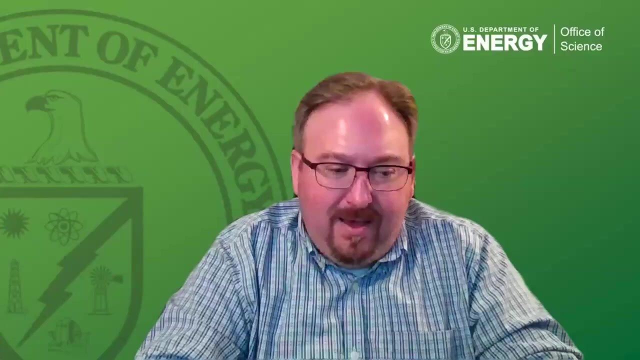 Of this I have no doubt. Oh, there's one. Okay, What would be the acceptable level of isotopic and chemical purity for the proposed isotope of interest that a Pi could propose? How much would what would chuck shock? Yeah, that's really difficult. 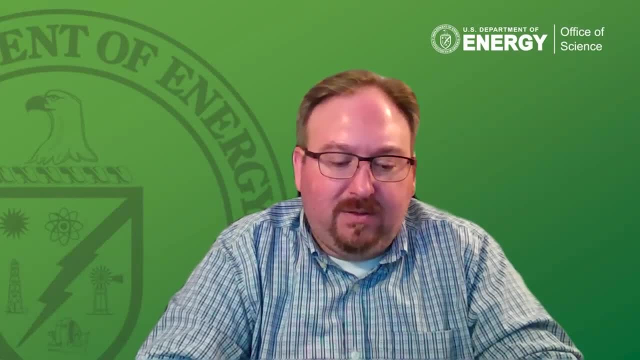 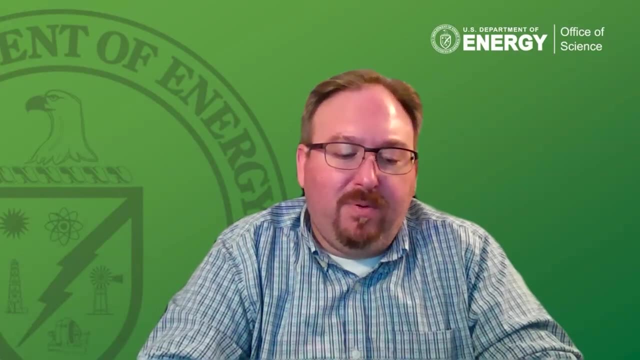 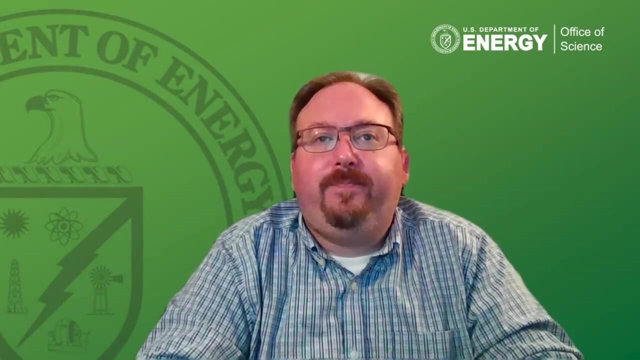 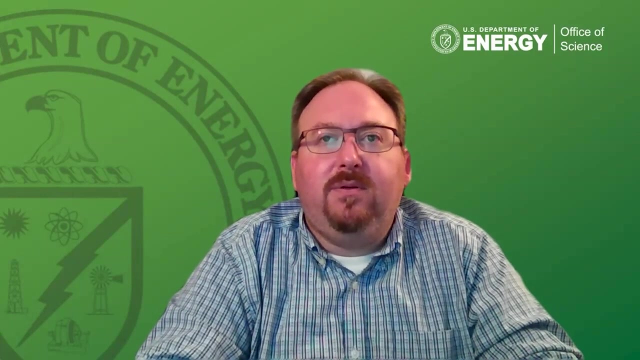 I think you just need to come up with your, with your best, your, your best estimate, And you know you're, you're gonna put in, you're gonna, you're gonna submit your own proposal. I'm not gonna define a a relevant limit across the board. 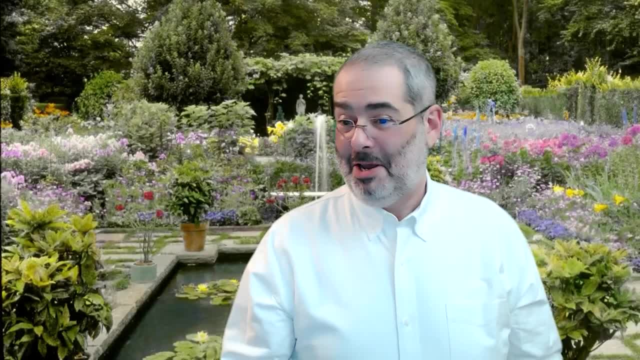 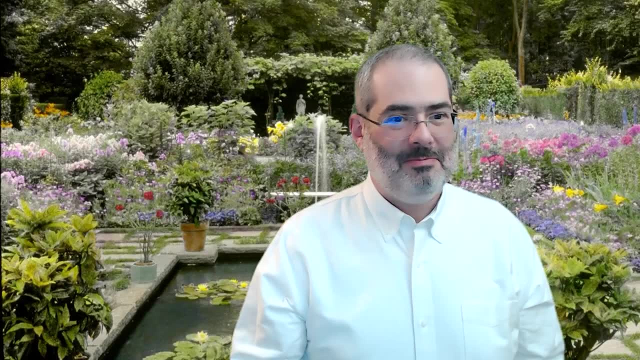 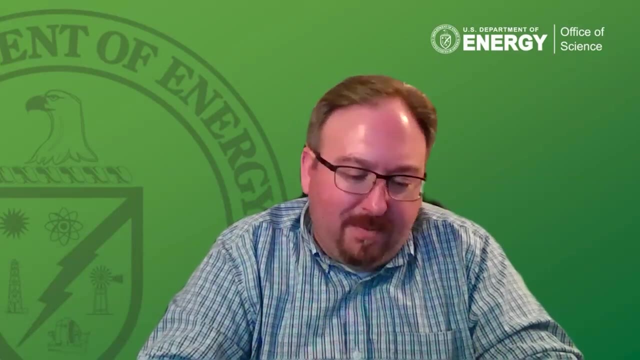 The second one. The second one was a thank you. Oh, here we go. Is it okay to have a collaboration with private companies outside the Usa, such as Iba? So, if you're, you mentioned the word collaboration. They're the, the, the pi or the. the researcher who asked the question mentioned the word collaboration. 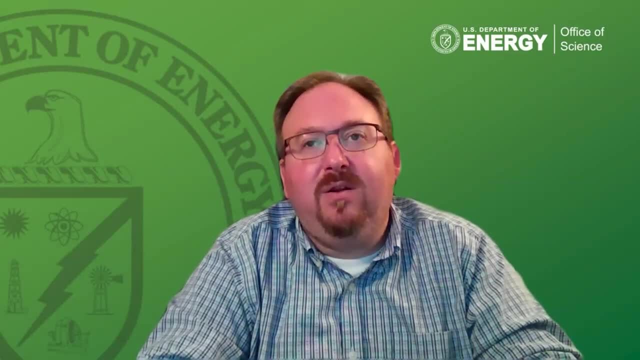 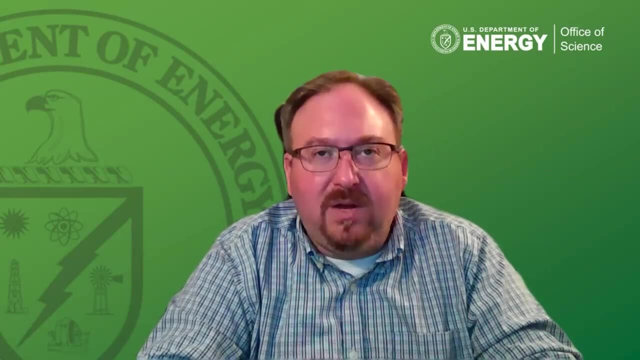 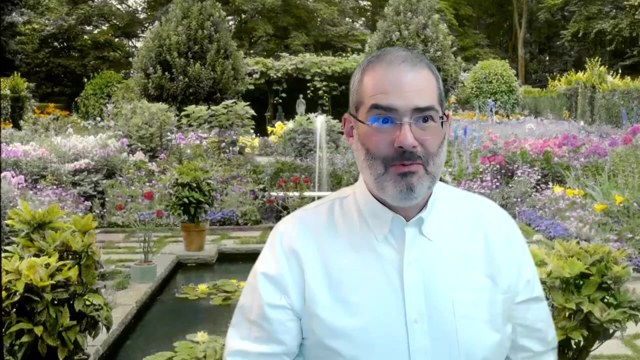 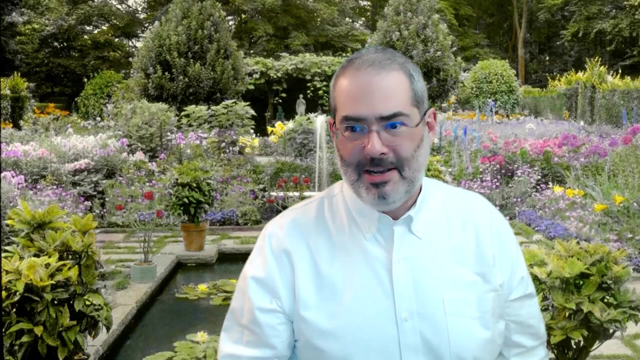 A collaboration in grant speak indicates that an award would be made. In the first few slides we indicated that industry was not eligible to receive an award, So the answer to that question would be no if we're talking about a financial collaboration. If, however, it's purely an intellectual collaboration- whereas someone on the scientific staff at Iba was your best friend in grad school and you still like bouncing ideas off of each other- and no money is going to the company- 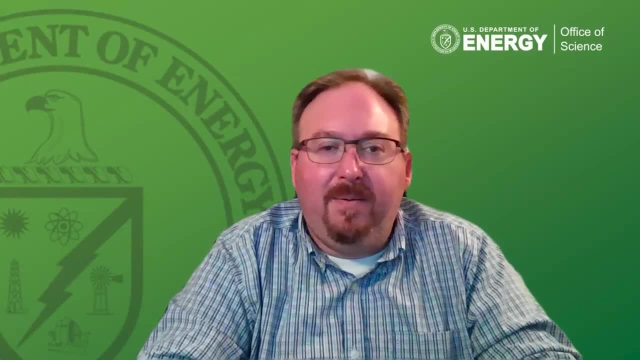 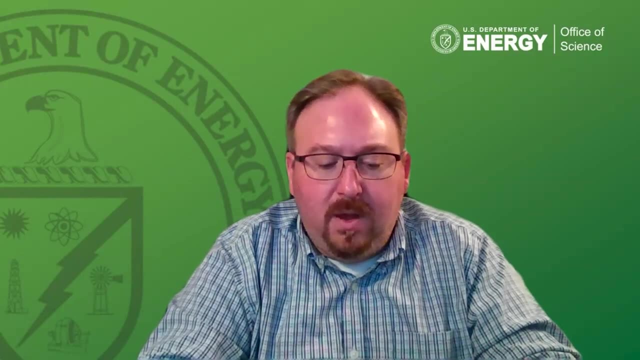 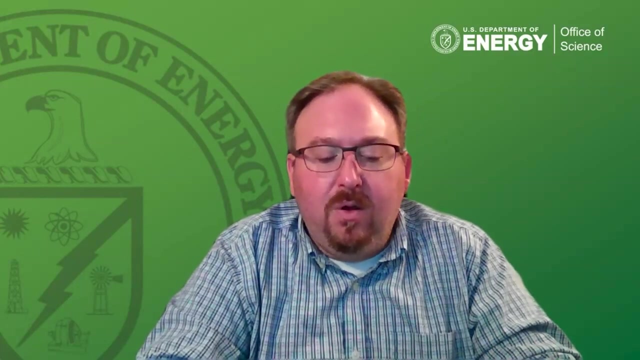 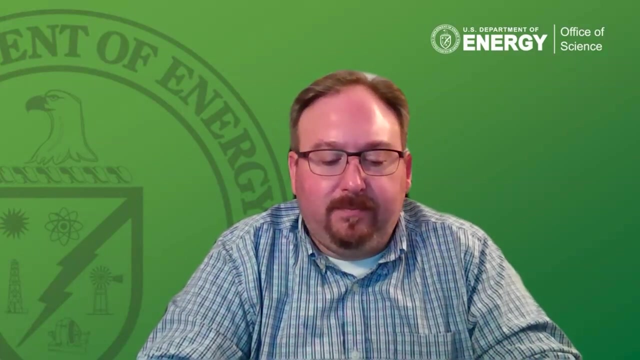 I don't think that's a problem, right, that's, that's a little bit different. And so what I would say there is, yeah, I would say I would say schedule a meeting just to make sure that What, what's actually gonna be, who, who's actually who's actually going to hold the Ip, that's developed. 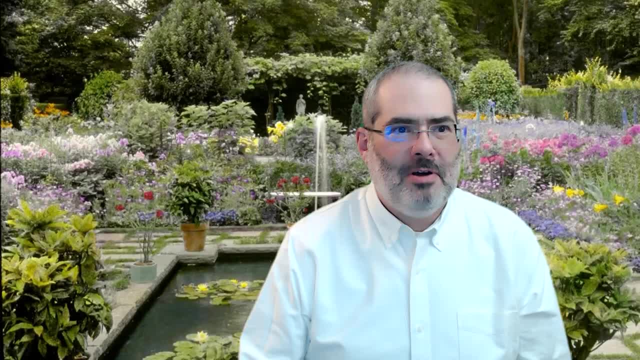 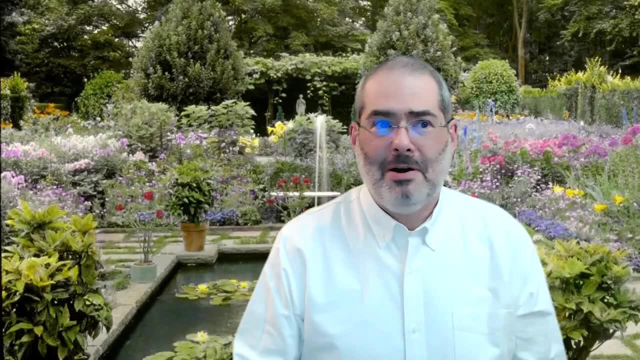 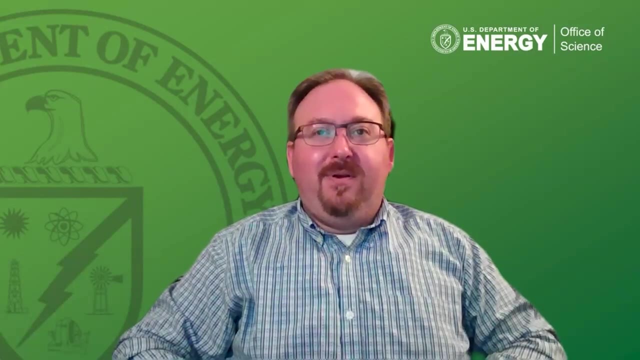 And with a reference to intellectual property from the isotopes program. I've just heard too much about Ip, indeed, And with that said, I believe we are approaching time. Okay, We are folks. I appreciate your time. Oh, we have one more. 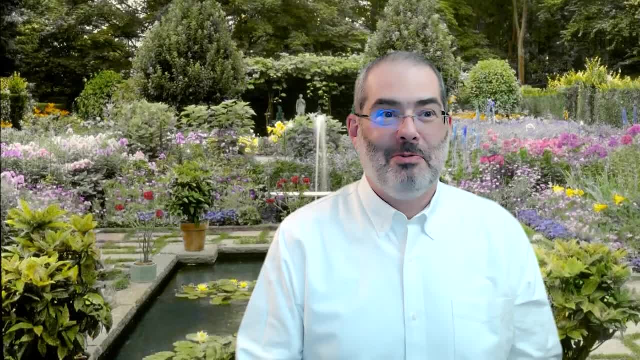 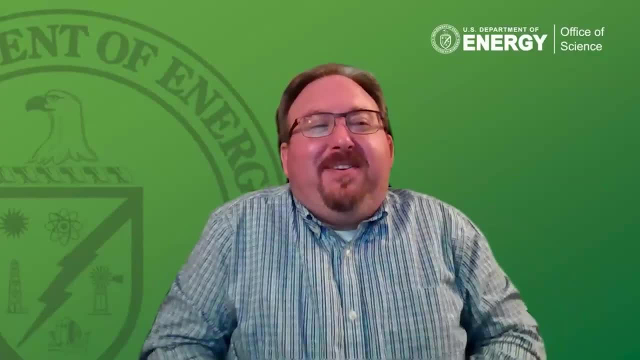 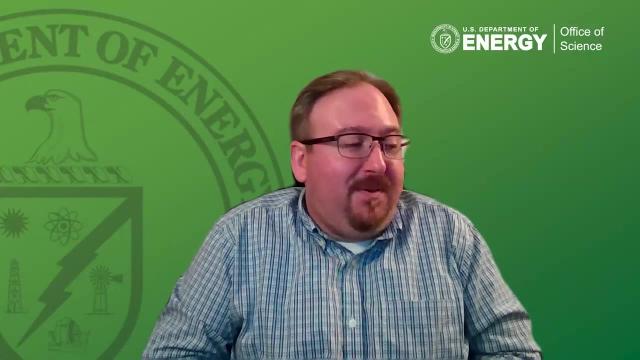 Is it a thing we have? We have a thank you message, All right, always appreciated, because gosh knows we civil servants don't get enough warm and fuzzies. I appreciate your time, I appreciate your willingness to spend the hour with me, and I am at your service. 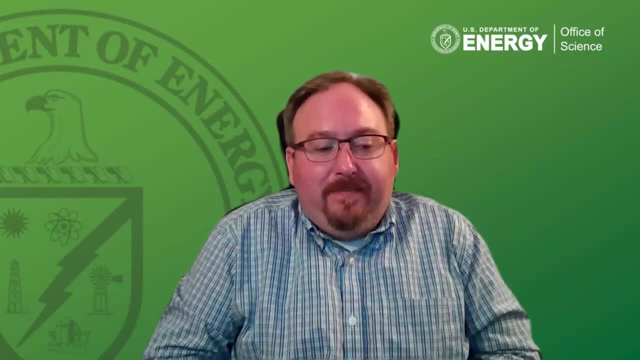 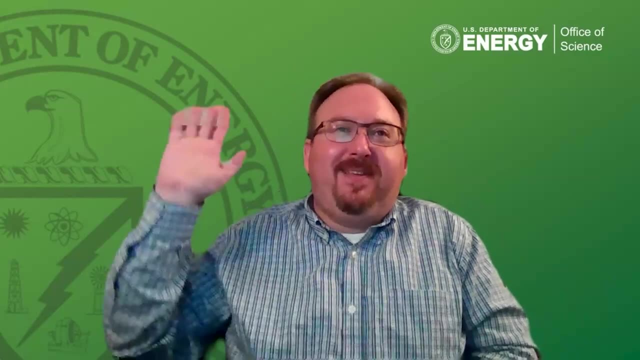 If you have questions regarding this foa, and I look forward to seeing what the community can develop. Thanks very much. Take care folks.